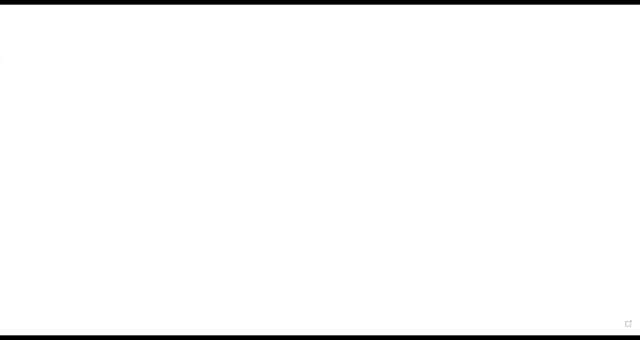 So what I'm going to do now is to just go over the FarmLog Unlimited story. So you have already come across the situation here. Here is the situation. Anytime you are doing a linear programming problem, okay, you will have to write the objective function First. 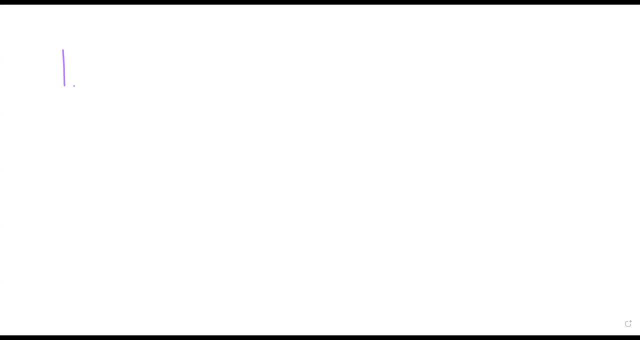 thing you want to do is to determine the decision variable. You determine the decision variable or you write the decision variable. The second thing you want to do is to formulate the objective function- The objective function- And then you will formulate the constraints, And then 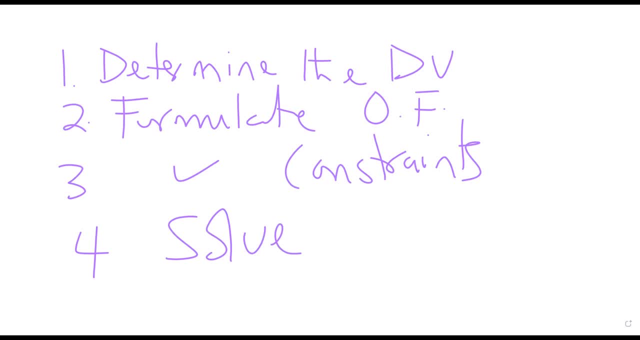 you will solve. You're going to do that solution graphically, So we're going to do the whole process graphically. So I know the entire story, So I'm going to tell you the entire story. In the process of telling the entire story, I'll tell you the answer. So the first: 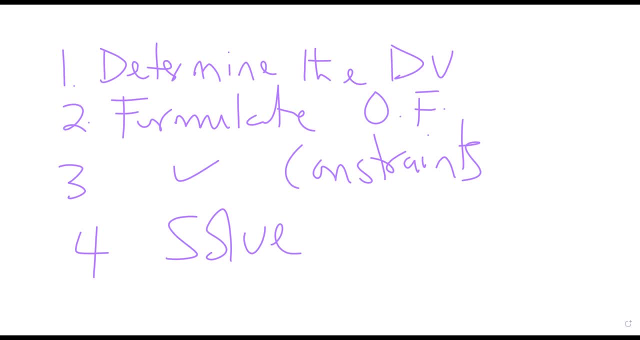 thing is to identify the decision variable. In the story preamble, the decision variable was that FarmLog Unlimited has to produce fan yogurt and fan chocolate, So you have to do that. So the decision variable okay was for you to represent X1 by something and 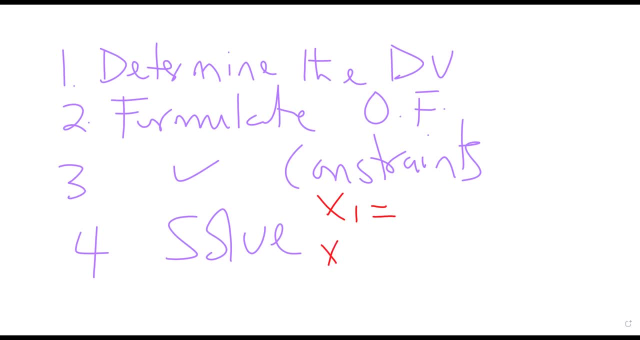 then X2 by something. Now the problem is that sometimes when people want to represent the X1, they just say X1, fan yogurt, X2, fan chocolate. That's not correct. You want to bring the unit of measurement, FarmLog, Unlimited. the fan yogurt is measured in sachet. 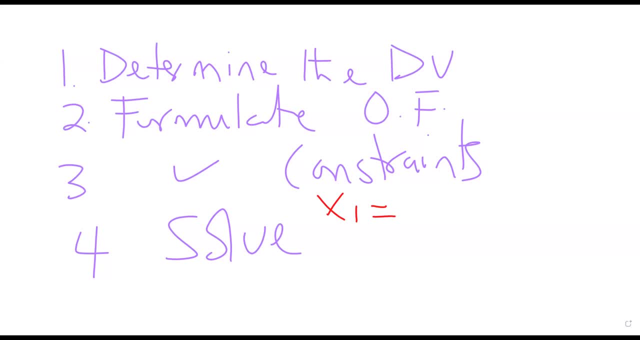 And the fan chocolate is measured in sachet. So you have to say that X1 is the number of sachets, okay, of fan yogurt to produce. Okay, And I want you to be writing this because while you're writing this, it's going to help The number of sachets of fan yogurt to produce. 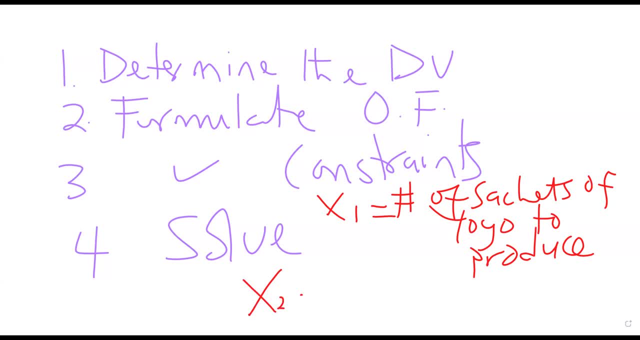 X2 will be the number of sachets of fan chocolate to produce. Okay, So it's very important to recognize this, understand this and apply this any time you are dealing with any of these things. It's very important. Okay, If you don't get it here, you let me know If. 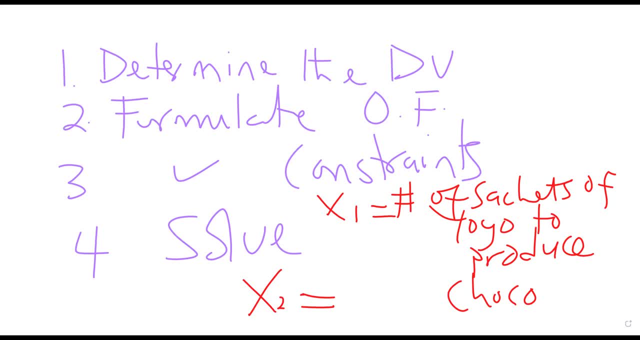 you don't get it here, you let me know now. If you are not getting it here, you let me know now. Okay, So the decision variable is the number of sachets of fan yogurt to produce. Okay, If you are not clear with this, you let me know. Okay, So learn how to formulate, because 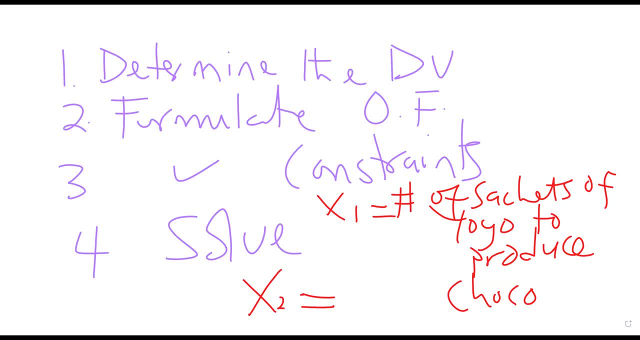 I normally will ask you all of these scenarios like what are the decision variables or define the decision variables? You've got to be able to tell me. And if you write the decision variables without adding the unit of measurement, wahala, So you have to add the unit of measurement. 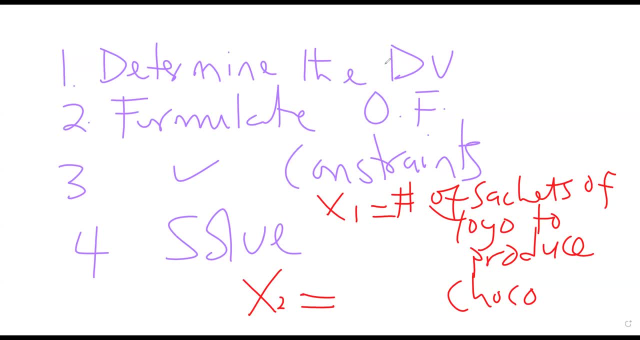 In this case and in this context, the decision variable is the number of sachets of fan yogurt. Any other question? The unit of measurement is the number of sachets, The number of sachets. So that's the first thing. The second thing is to formulate an objective function. Now, in the story that 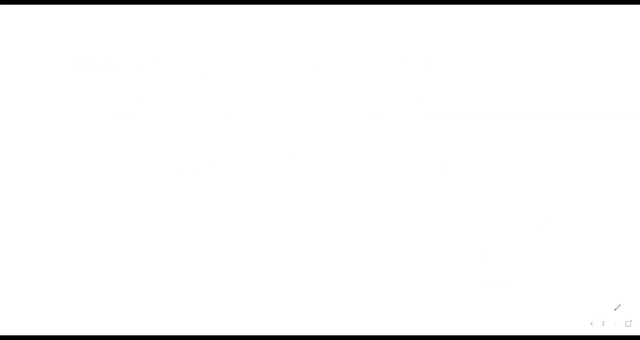 we were given, we were told something about objective function. Any time you are formulating objective function, you bring it where the letter Z. Z is the objective function. Z can be revenue, Z can be profit, Z can be cost. Okay, About what you use Z for The. 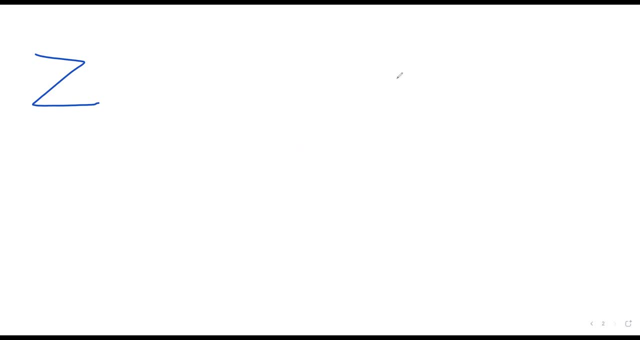 number of sachets: X, X, X, right. Their value Is always equal. Okay, Now, if you are not clear with the generation of meetings, whatever we do your budgeting, we're not going to put it. z can be distance and you always write it as z max or z min Max. when you have identified that. 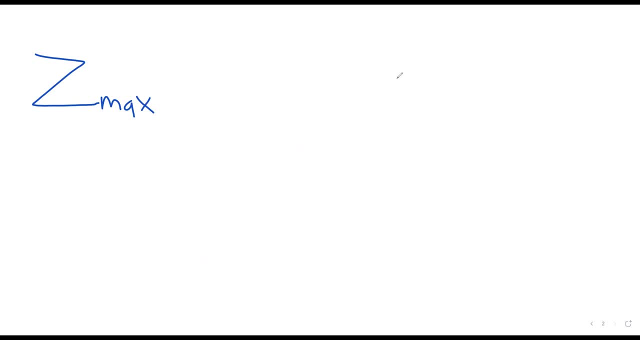 is a maximization. Now, according to the story which I know you all have in front of you, the story said that Farmer Ghana Limited want to know how many sachets of Fanyogo and Fanchoko to produce in order to maximize profit. 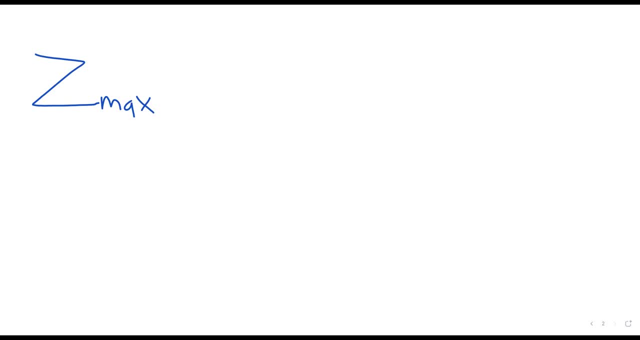 So the z function is supposed to be z max, max as a subscript. Then you make it equal to and I'm giving you the general approach. the general approach is that c x i plus c j x j, that is as many of the variables that you are dealing with, up to c n, x, n, In other, 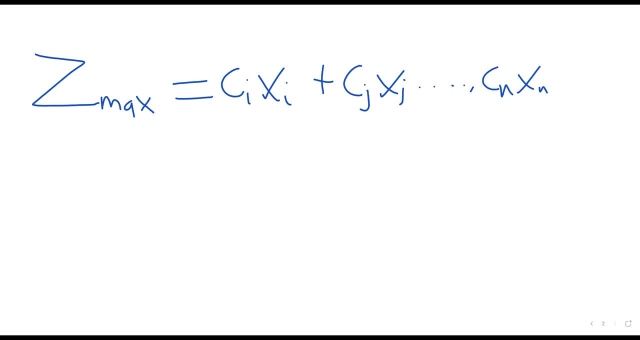 words. as many of the decision variables are there, each one must have a c coefficient. The c, ladies and gentlemen, the c is the coefficient. Another name for the c is the coefficient. It is a per unit, something per unit profit, per unit cost, per unit revenue, per unit distance. 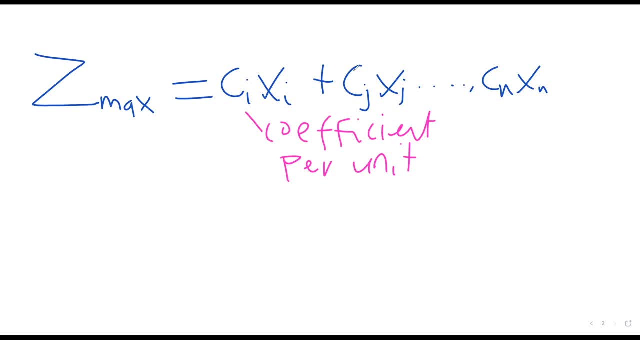 per unit, something, and it is being multiplied by the decision variable. So each of the coefficients is a number, It is a number, okay, and it's multiplying. So the goal is that, now that that per unit means that it is for. 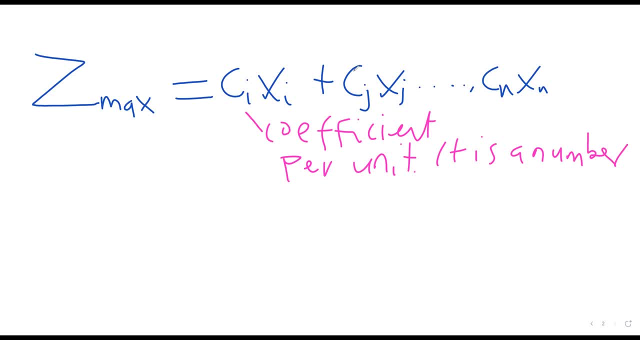 a single one of the decision variables. you are dealing with one of them. one of them And for our purpose and for this course, we were told that this guy, this company, is producing how many sachets of Fanyogo? of course, Fanyogo is x 1. We are told that they are producing 40 units. 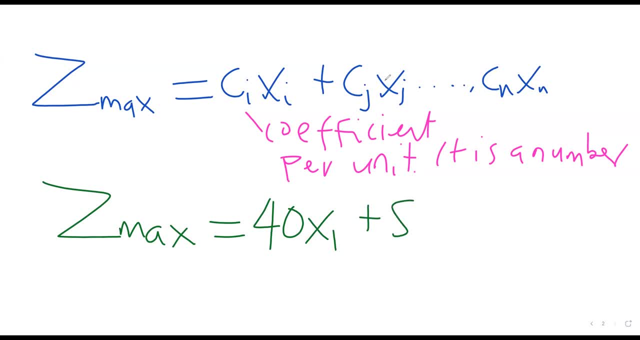 of fine yogurt and 50 units per unit of fine chocolate. Of course, if there was another one like fine ice, we would have had a coefficient for it, and then that would be x-ray okay. So this is how you formulate objective function. 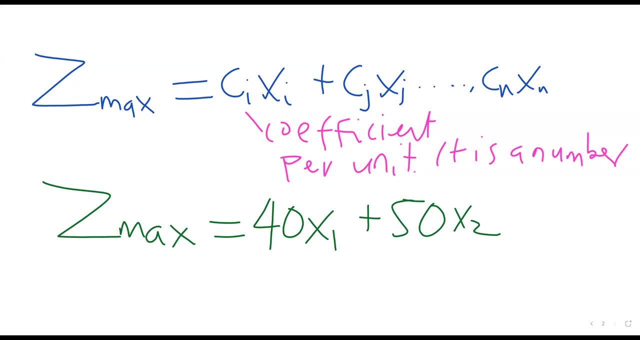 After you formulated objective function, then you are now good to go forward. Now, if you don't understand how you I formulated this objective function, you just raise your hand and I'll just clarify it. Okay, now, after you've written objective function. 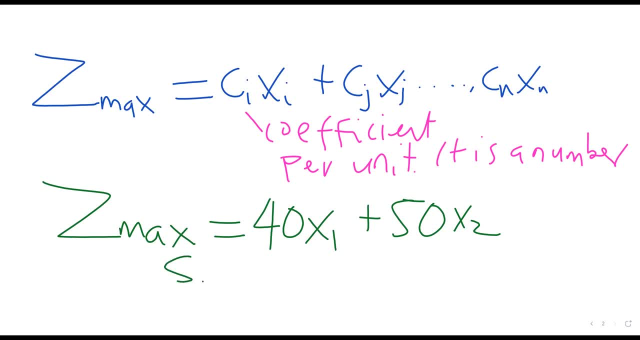 you now bring the terminology subject to, because you've already learned that you cannot maximize profit alone, because you are limited, You are restricted, You are constrained by some constraints, And so you're gonna be able to formulate the constraints. Now, the way you formulate a constraint: 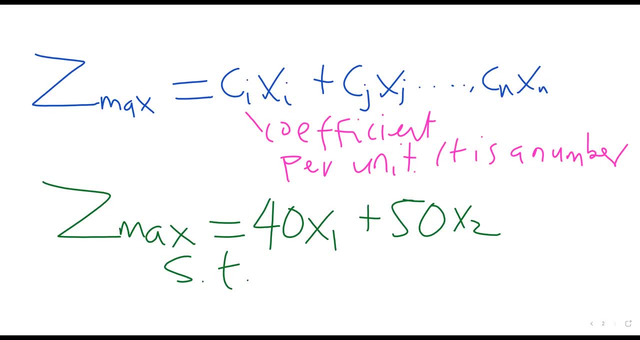 is very important. ladies and gentlemen, There is an approach you should always follow whenever you are formulating the constraint. The first one is to know that we have the left-hand side of the constraint. We have a symbol or a sign, and then we have the right-hand side of the constraint. 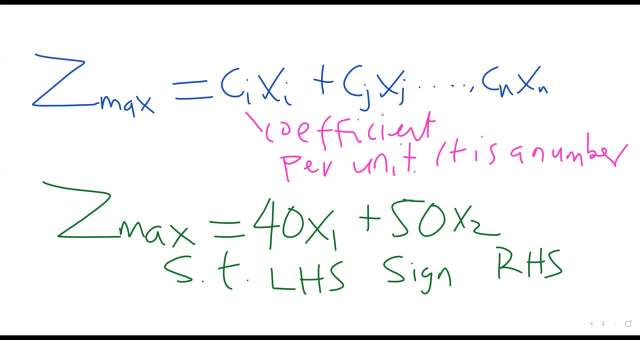 Okay now. the left-hand side of the constraint is usually called usage- usage. Then you have your sign and then you have the right hand side of the constraint. The right hand side of the constraint is known as available- available. I'll explain each one of them. 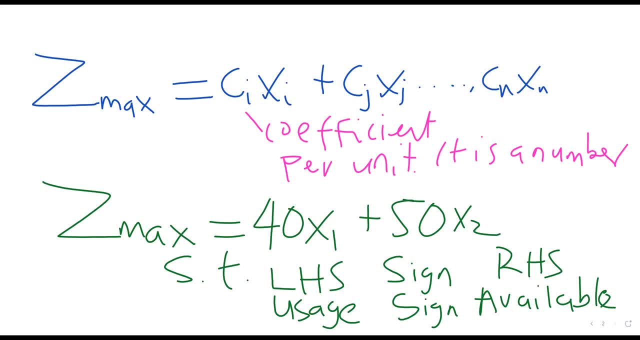 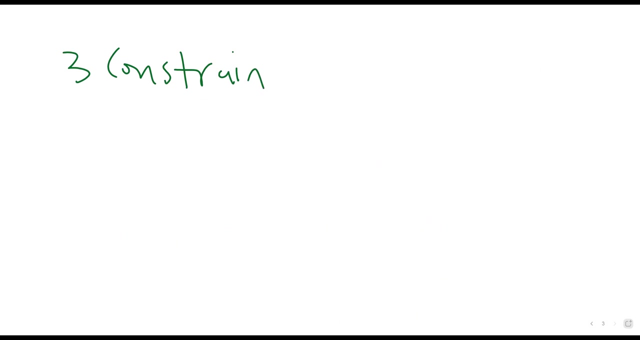 Available Now. usage deals with the number of quantities you actually used of those resources. okay, Now, please note that there are things kinds of resources, or there are three kinds of constraints. okay, there are three constraints that you should have in mind. the first one is known as a resource constraint- resource constraint. then we 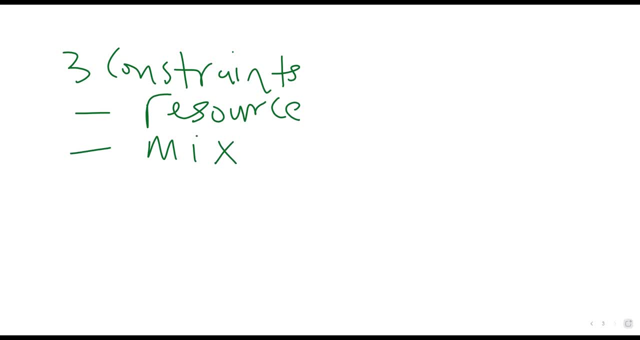 have the mixed constraints, and then we have another constraint, well known as the non-negativity constraint. non-negativity constraint: now, these constraints are what might be given to you whenever you are doing the formulation: okay, now you'll be told of the available consciousness, available resource constraint. that is there. so that is what will go on the right hand side. 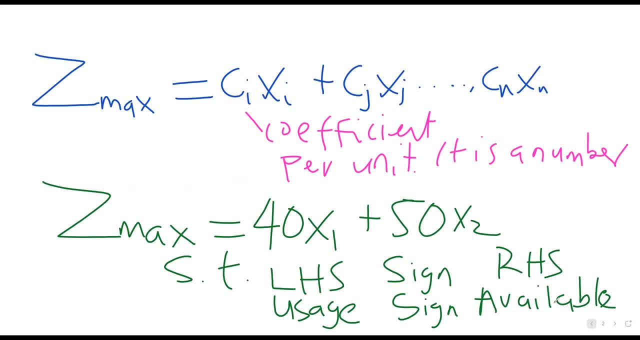 so on the right hand side, is that available now? the word available means something. it means that That is all there are. That is all there are. You can use all of that or you can use less of that, But you can't use more than what is available. 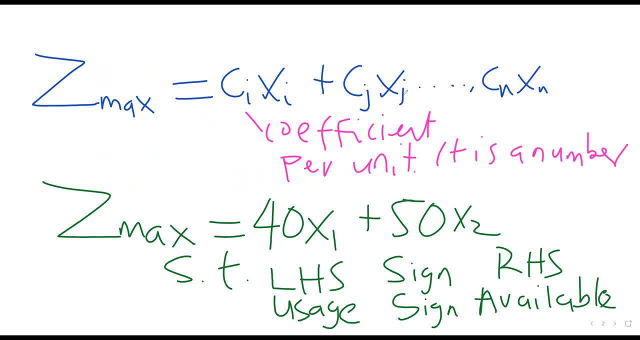 You can't. You can't do that mistake Because the resources are limited, Resources are limited And because resources are limited, you are limited regarding how much you know labor hours you can use And when you look at the story very carefully, you will be told that the hours of labor that is available is how many. 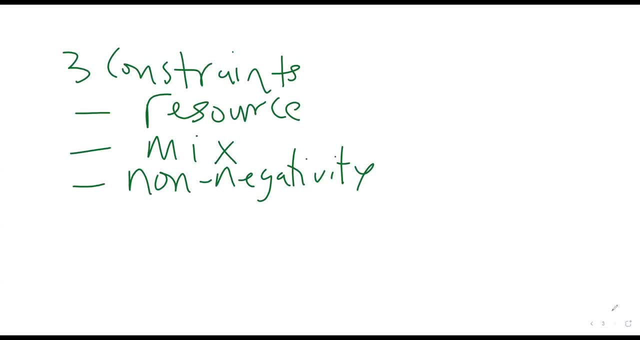 You can tell me. Type it there for me. The hours of labor available is what. What was the hours of labor available? Just type it there in the chat for me, This one saying it will be two something. What is the hours of labor available? 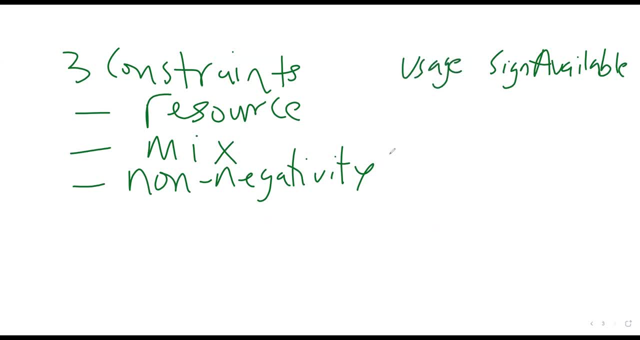 Type, Because I'm recording this and I want to use this to give Max to do that type things. The hours of labor available is 40. So you will now, on the right-hand side you are going to put the number 40 hours. 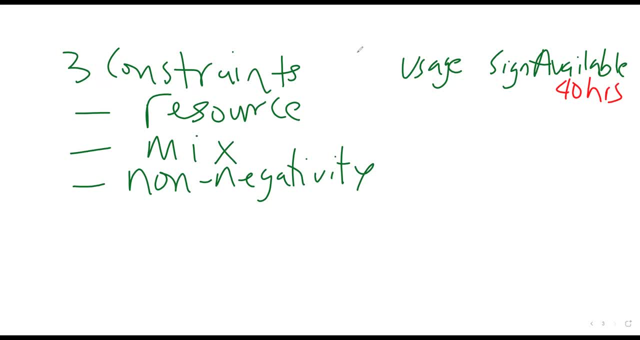 40 hours. And then the gallons of milk. So we are talking about labor constraints, And then we are talking about milk constraints. We are told that the gallons of milk available is also how many Gallons? Excellent Victoria. So that is 120 gallons. 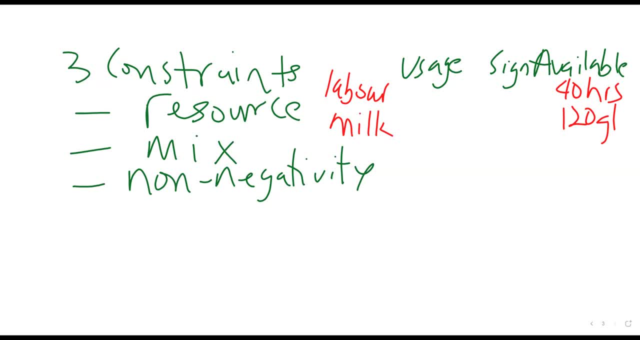 120 gallons Now, because these things are available and you cannot use more than what is available. what sign do you think should be used for this? What sign should be? What mathematical symbol should be used? What is available? What is available. 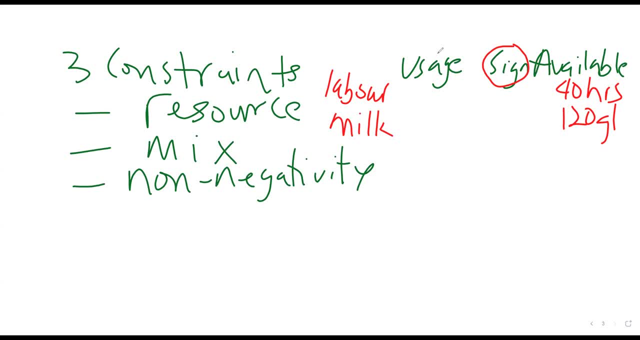 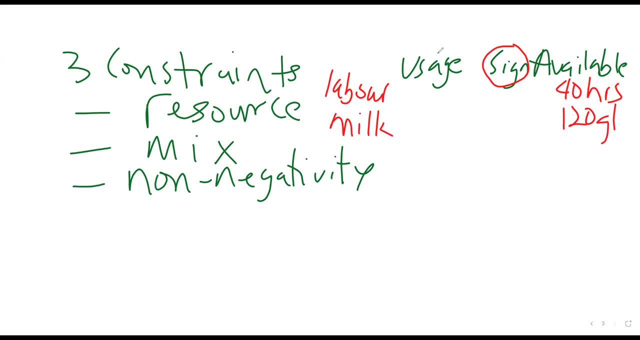 Susanna, that answer is wrong. Vincent, your answer is correct, Because it cannot be less than, It has to be less than or equal to. So the less than or equal to is what you are going to write for the sign. But I want you to understand what the less than or equal to means. 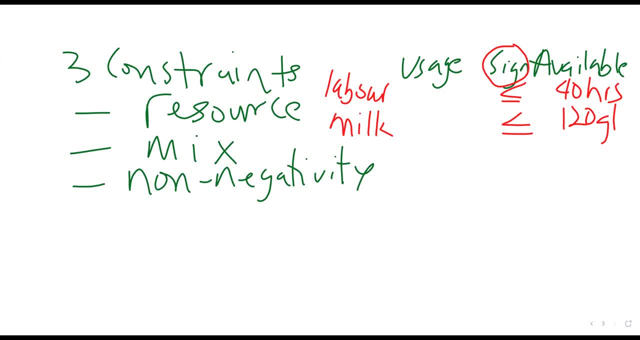 What is the equal to part? The equal to part is when you have used everything. Everything You see. the usage is on the left-hand side. So if you use all of the existing powers of labor, then the symbol becomes equal to. 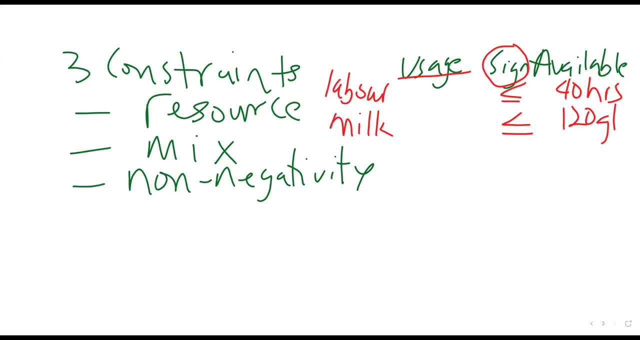 But if you don't use all of the available resources, then it becomes what It becomes: less than. That is why it's less than or equal to. Now go to the story again. Go to the story. See, I'm not the one going to show you the story. 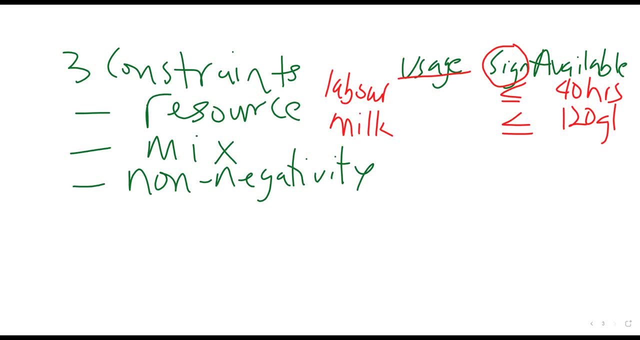 By now you should have your story in front of you. The story said that, in order to, one hour of labor time was used to produce fan yoga and two hours was used to produce fan choco. So watch: One hour was used to produce fan yoga. 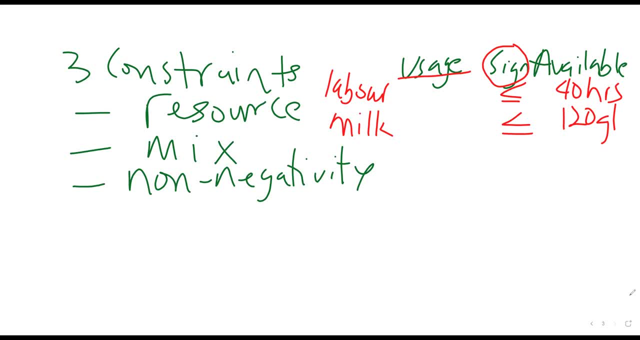 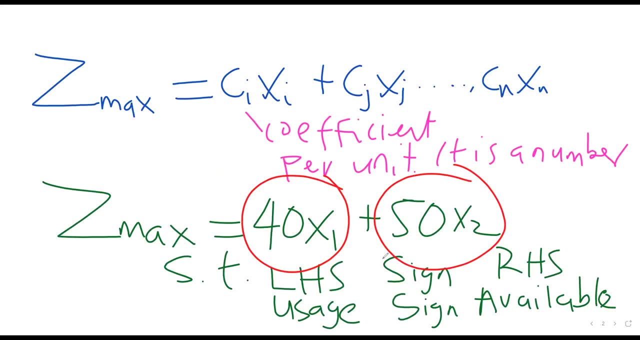 And we know that in the X and the Y formulation fan yoga comes first and fan choco comes second. One hour was used to produce fan yoga And then another one hour, two hours, was used to produce fan choco. So the usage will be 1X1. 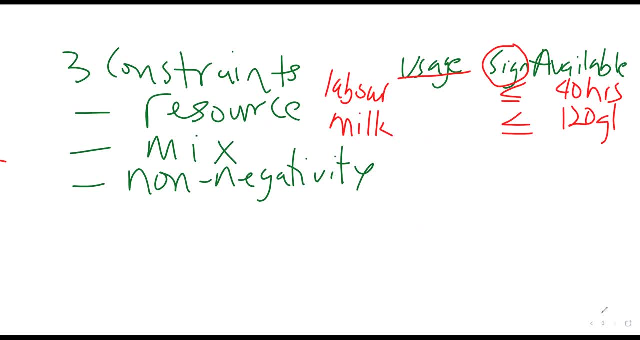 That is one hour. I'm writing the one for a reason, And then for the choco you will have 2X2.. Okay, You have 2X2.. And then we're told that for the milk, four gallons. 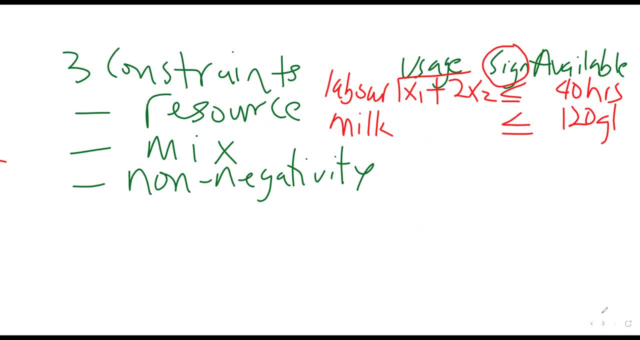 of milk was used to produce the choco. Four gallons of milk was used to produce choco And three gallons of milk was used to produce fan choco. So fan yoga has four gallons used, used, used, utilized. So that's how you do the formulation. 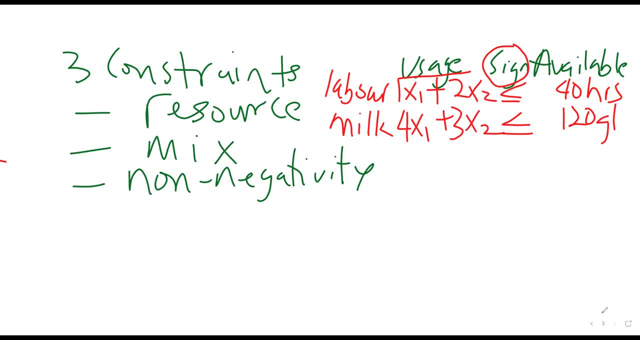 And then you bring your non-negative, non-negativity constraints. which is what? Which is X1 and X2.. That is your decision. variables should be zero or positive. It's not like they should be, they should be just positive. 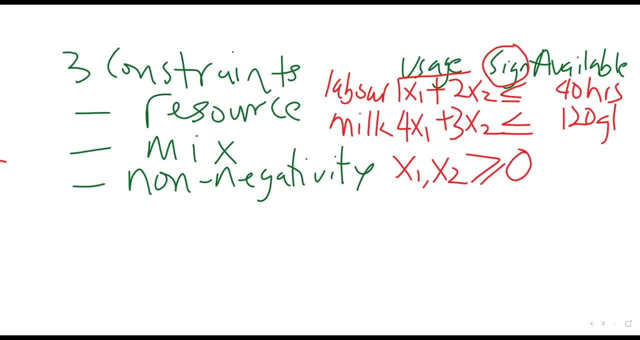 but they should be zero, Because sometimes you will not produce anything. Some people start company, Okay, And in the first year they produce nothing. You know it's all loss, loss, loss, loss, loss. So the zero part of the non-negativity is reasonable. 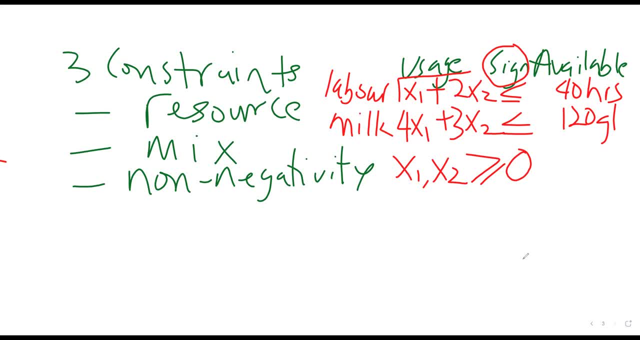 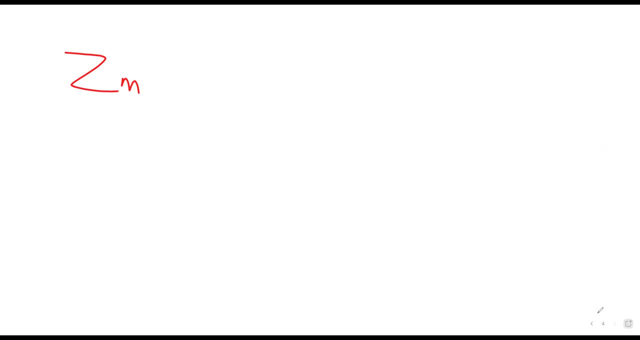 So, on the basis of this, we can now rewrite our entire entire formulation, And the formulation becomes Zmax equal to 40 X1 plus 50 X2.. See now, when you see it like this, you're not afraid, because you know where it came from. 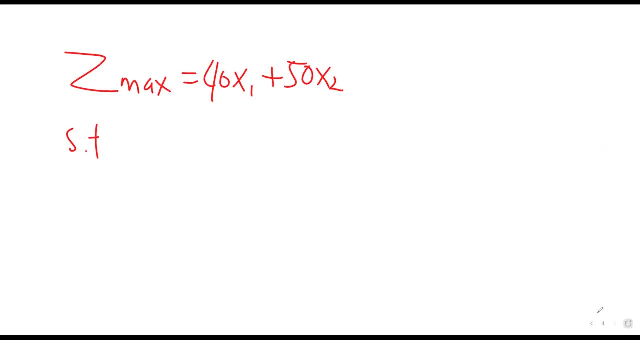 Okay, Subject to. then you have your first constraint, which is X1 or 1 X1 plus 2 X2 less or equal to 40 X2.. Then 4 X1 plus 3 X2 less or equal to 120.. 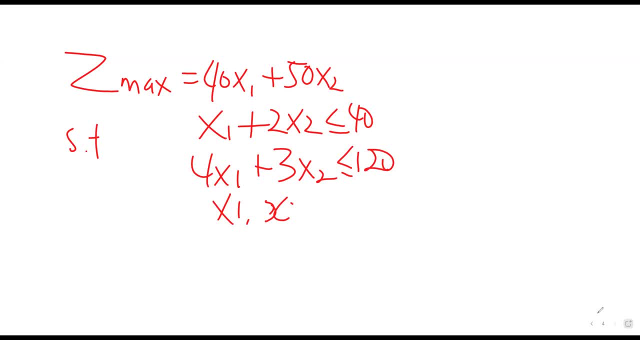 Then your non-negativity constraints. Okay, So this is your whole situation. Now the question is that we need to be able to find the optimal solution, but you can't find the optimal solution unless you have the optimal feasible solution. Okay, 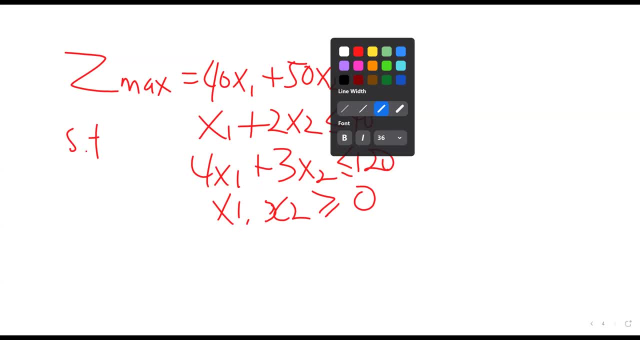 So, in the feasible solution that you get, you guys have learned already. I'm just recapitulating: You have learned that you have to plot your X and then your Y: X1 on the X axis, X2 on Y axis. 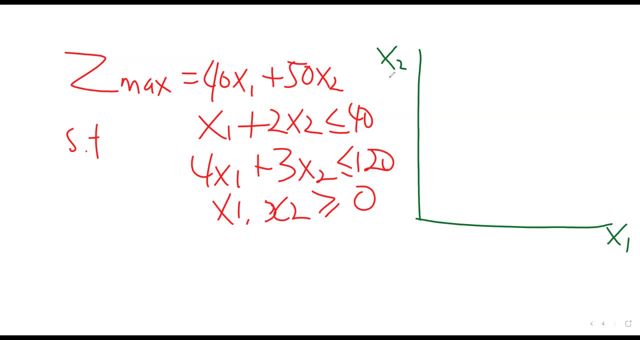 And you're going to plot them. How do you do the plotting? How do you do it? What you do is that you first deal with the constraints. So you deal with the labor constraints and then go and deal with the milk constraints. You start all the plotting with a constraint. 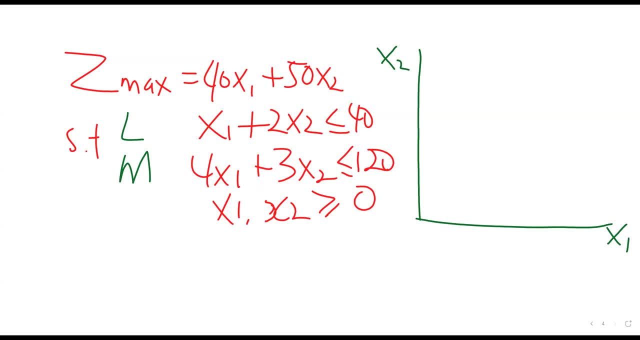 So the constraint is to say: follow me here, follow me here, follow me Please if you are getting value type value. if you're getting value type value, because I need to be sure that you are on the same vicinity with me. 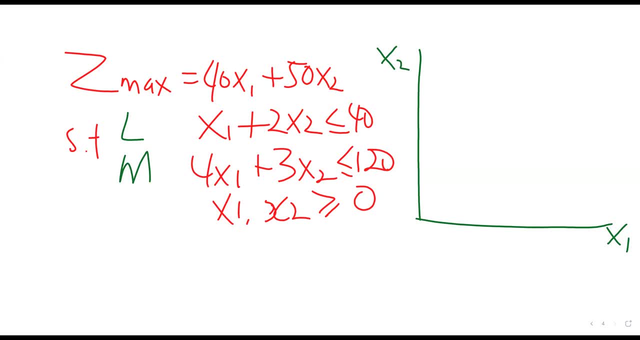 Got to get some value type: value type V. If you are getting it, say yes, I'm getting it. If you are not getting it, say no, no, no, no, no, You are getting it. say yes, Yes, yes, yes, I need to be sure. 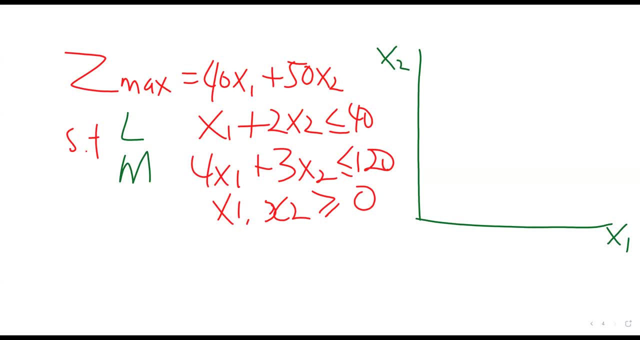 And you know what you are typing. if somebody is saying that: why do I have to type? Now imagine that that typing is what is going to get you, is what is going to give you an, a, you will type. or a million dollars, you type. all right now, once. 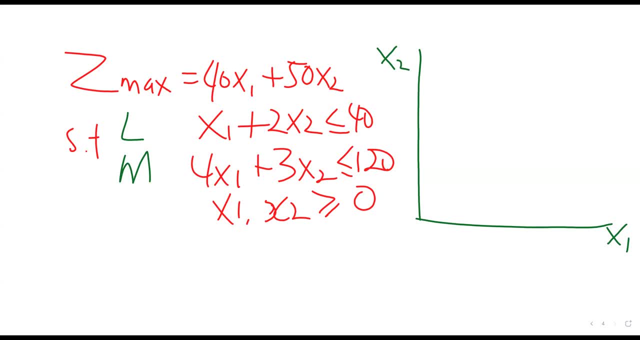 you've done that. now let's deal with the first constraint. the first constraint is x1 plus 2, x2, equal to 40.. why am i using equal to? because at least i'm using the maximum value. okay, because everything is below it, okay, so the equal to is going to be the line below it, which is the. 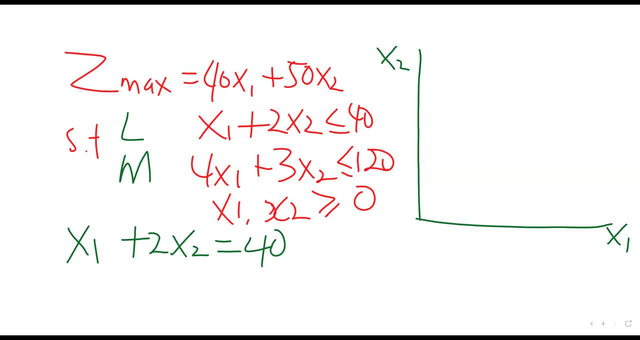 less than is going to be the space below the line. now, this is an equation of a line. in case you've forgotten an equation of a line. an equation of a line is: y is equal to mx plus c. okay, that's the equation of the c is the number, which in this case is the 40. okay, and then the y and the x are the x. 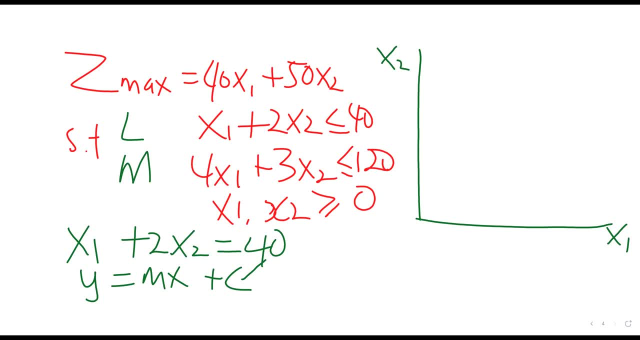 one and the x two here. equation of a line. you just need two points to draw an equation of a line. okay, so all you will tell yourself is that let's assume that that's what you do. you make an assumption here. you say that, assuming that this x2 is zero, okay, assuming x2 is zero here. 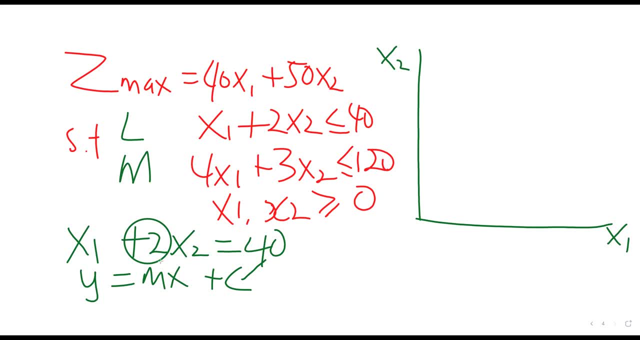 what is going to be x1? who can tell me, assuming x2 is zero, what is x1? assuming x2 is zero? what is x1? okay, if x2 is zero, then x1 is 40. somewhat good answer. okay, if x2 is zero, then x1 is 40.. so you will know that, that the coordinates that you need, the first. 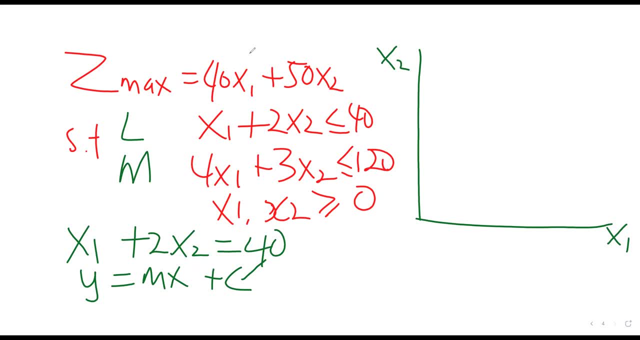 one is 40.. okay, now, if x1 is zero? what is x2 if x1 is zero? what is x2 if x1 is zero? vincent, good, that is 20. okay, so you are going to plot 40 on the x axis and then 20 on the x uh y axis. 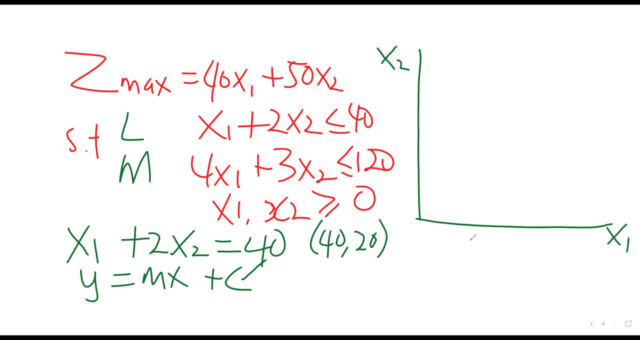 so 40 on the x axis. so 40 is the x1. so when you look at the x1, just identify somewhere here and call it 40.. okay, and all you need are two points. and then go to the x2, that's the second number, identify somewhere there and call it 20.. 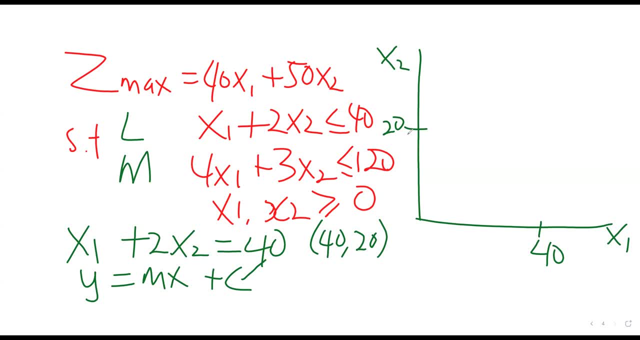 and all you are going to do now is to join the two lines together. so you take the 40, join it to this. now you've been able to plot that one. now you go to the second constraint. so if i were to name this constraint, okay, if i were to label this constraint, it is going to be x1 plus 2x2. 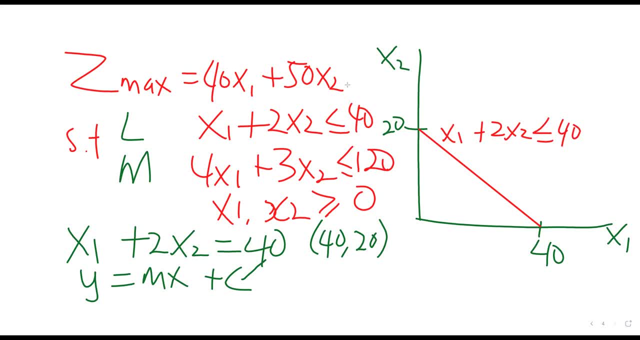 less or equal to 40, whereby that less or equal to 40 is referring to the entire line plus the space. okay, and you want to really note that thing. it is referring to the entire line plus the space, all of that entire line plus the space here. that is what is referring to that. 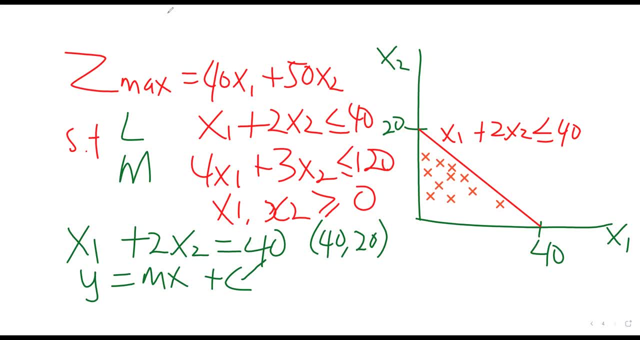 now we can go ahead and now do the second constraint. now, what is the second constraint? the second constraint says that you have 4x1, okay, plus 3x2 less or equal to 120, or in this case, we'll make it 120.. so you have 4x1 plus 3x2. 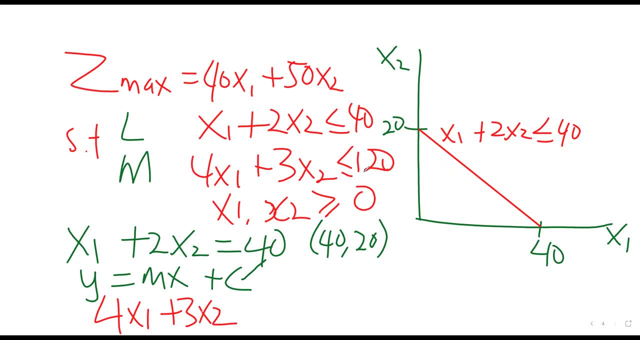 equal to 120.. we just take the limit, okay. so if x2 is zero, what is x1? if x2 is zero, what is x1? and this is where i need you. i need you to be working along with me. if x2 is zero, x1 is 30- fantastic, okay. 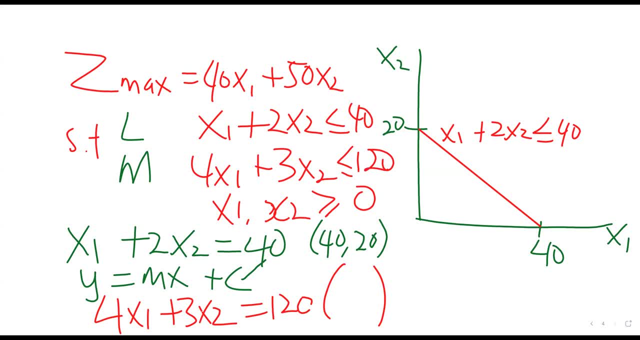 there are some great guys helping me here. okay, so x1 is 30. if x2 is zero, x1 is 30, and what if x1 is zero? if x1 is zero, if x1 is zero, x2 is what, x2 is 40.. all right, so on the x1 axis, you can see that you have 30, okay. 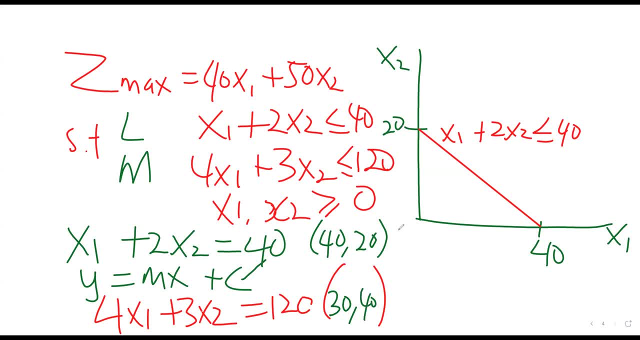 and then on the x2 axis you have 40. So here you have 30, and 30 is going to be below 40. So you put it somewhere here and call it 30. And the 40 for the x2 is going to be above the 20. So let's put it somewhere here. 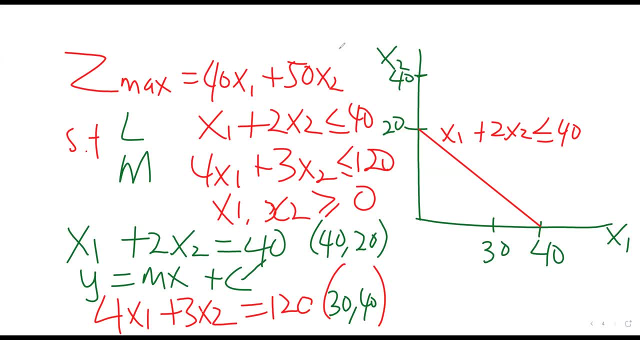 and call it 40. Now the job you got to do is to join these two lines. That's what you want to do: Join these two lines. So you join the 40 to the 30, like this, And so the space in question. 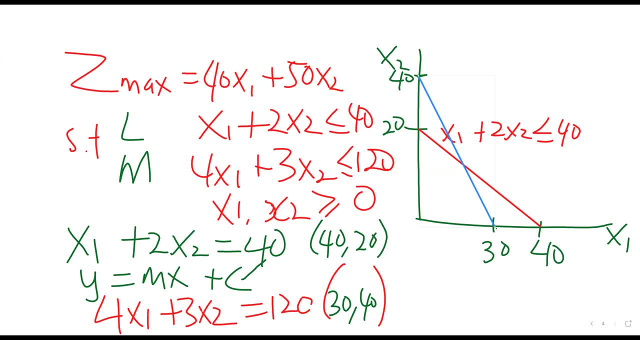 okay, for this whole, you know number, that is the space in question. That is the space in question. That is the space in question. So, on the basis of this, these are called the feasible solution area. okay, The feasible solution area, Both the three spaces And what are the three? 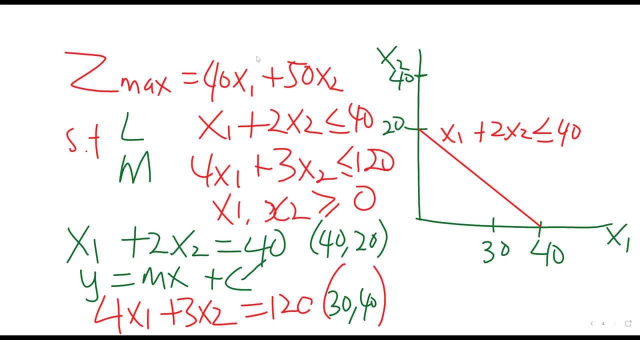 spaces. Well, you can see clearly that the three spaces are the three spaces. Let me just go back to this. okay, The three spaces are one: this one, this one, this one and that one. Those are the three spaces. 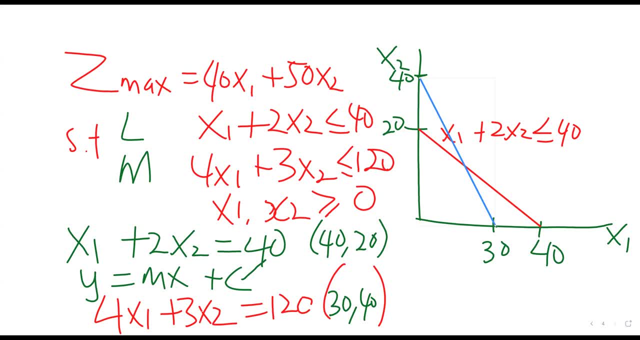 One of them is common to all of them, and that is known as a feasible solution area. okay, Feasible solution area. And that feasible solution area, or a common solution area, is a feasible solution area, And that feasible solution area is a common. 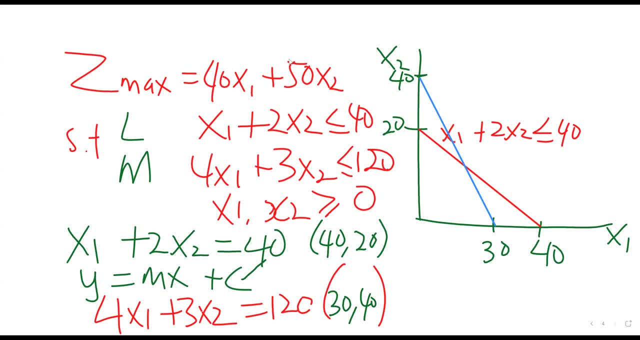 solution area And that feasible solution area is a common solution area And that feasible solution area is a common solution area And that feasible solution area. that is going to be the number that you see here. So let's call this point A point, this point B point and that point. 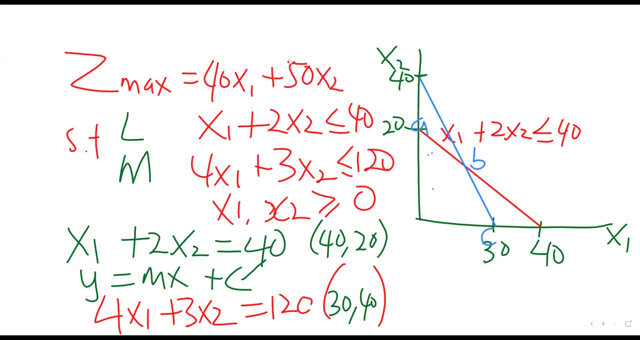 C point. So this area that you see here, that is a feasible solution area. Now listen here. This is where it gets interesting. This is where it gets interesting. Your job is to find the coordinates of all the vertices of this area, And that is the feasible solution area. And that feasible solution. area is in thoseiant and that is the feasible solution area. So, where it gets interesting, This is on. So that is the feasible solution area And that is the feasible solution area, And that feasible solution area, and that is the feasible solution area, And that is the feasible solution area And that happy. is a position where you would have virtually no improvement on something like that. Now, this is a conceptual solution, So you have to learn how to use it in a test effects process. you know It is kind of an ass. 1960s there is, it is. 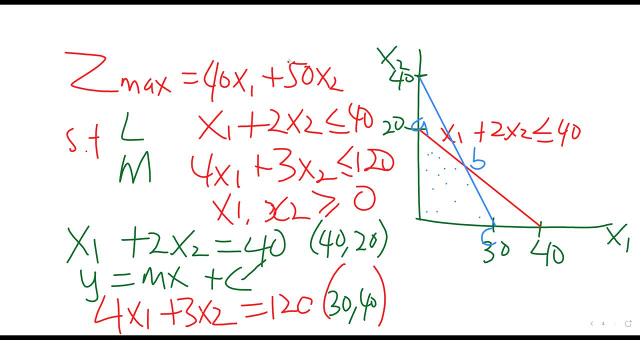 quadrilateral کو 2018, kinda ha-ha-hà. You remember the good old days of A level and the SSS? You have to learn about quadrilaterals. you have to learn about quadrilaterals: a polygon, a hexagon, playful. 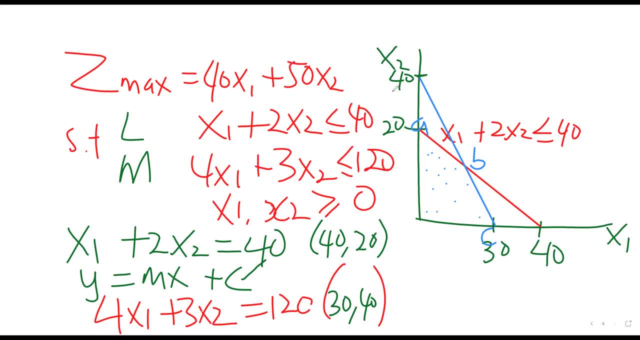 Now, this is a quadrilateral. what is a quadrilateral? the quadrilateral is from this. The quadrilateral is from this section: A, A, A, all the way. I'm just going to use a different thing to show. You've got to be able to have a feel. 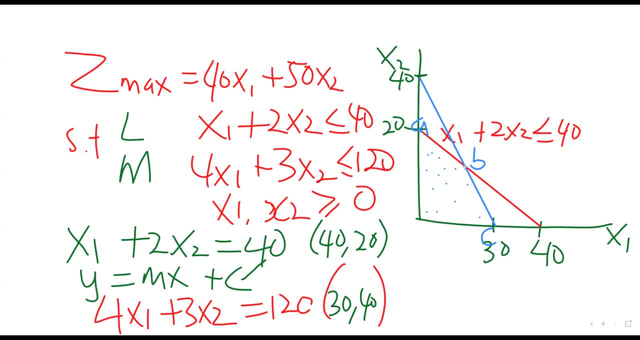 It is A to this point B, and then B to this point C, And then bounded by this distance up to the zero, followed by this distance up to the C. So you can see that space, That space has got vertices. 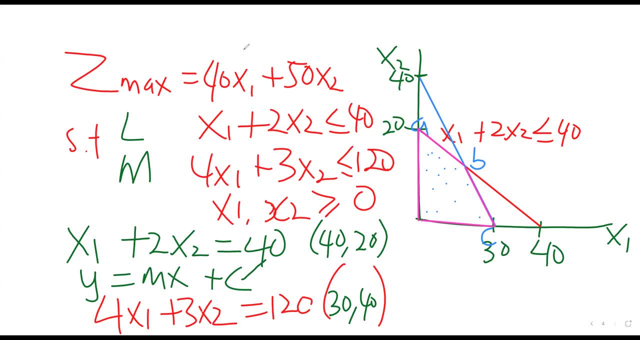 And the first vertex is the zero, So we don't want to deal with it. That point here. zero, zero. So that one is not too important. What is important are vertices A, B and C. Your job, listen, your job is to find the coordinates of each of those vertices. 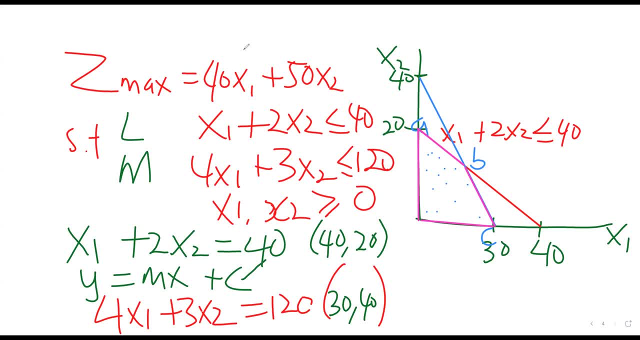 And when you put those coordinates back to the Z function, where is the Z function? This is a Z function. When we put them back into the Z function, the one that will give you the highest profit. that coordinate is the optimal solution point. 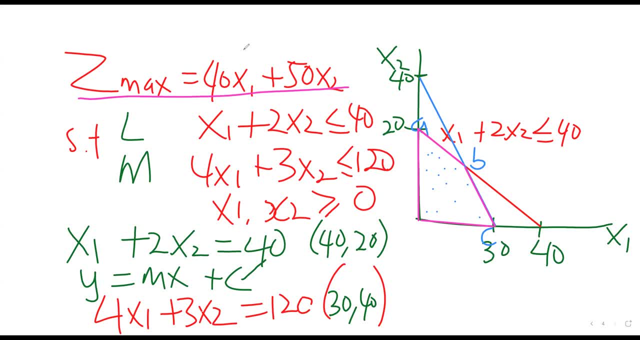 The one that will give you the highest profit is the optimal solution point. So, in other words, I am looking for, I'm looking for Z, and I'm looking for Z value at the point of A And I'm looking for Z value at the point of C. 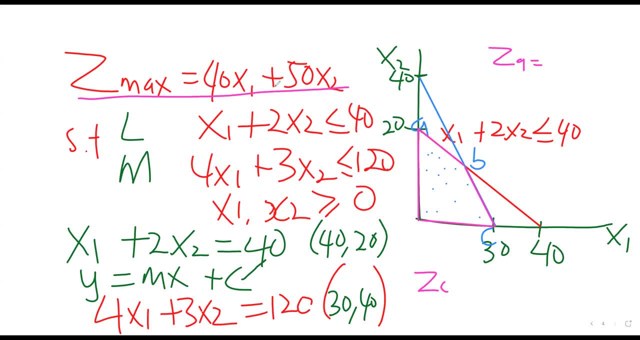 And I'm looking for Z value at the point of B. There's a reason why I put the B last. Okay, so let's go to A. Let's go to A. At the point of A, the coordinates are zero for the X1,. 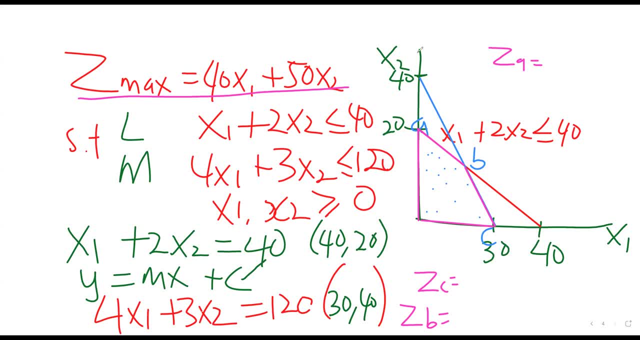 20 for the X2.. Okay, Zero for the X1.. Someone says he can't see my screen. Do you all see my screen? I want to be sure. Do you all see my screen? Okay. so, guy who says he can't see the screen, 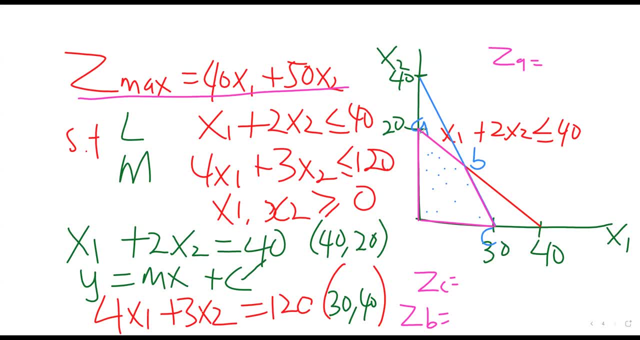 please log out and log back in. It's from your end, Okay. so let's go to A. We want to know the values of the value of the Z. That is a profit If we slot in the coordinates of A and the coordinates of A are zero and then 20.. 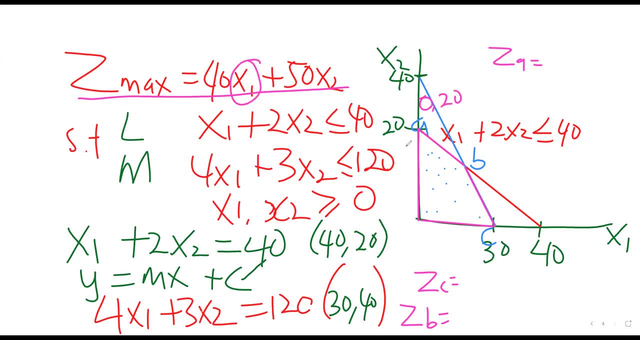 So let's drop it. Whatever we see X1, we put in zero, And whatever we see X2, we put in 20.. You drop that into the Z value and tell me the answer. Who can tell me the answer for that? 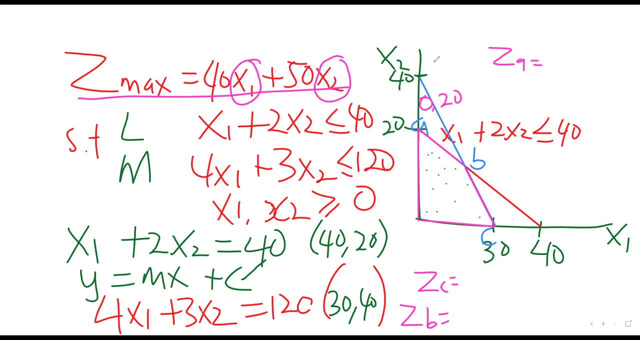 Okay, Okay, If you drop that, if you drop that into the Z value, what will be the answer? What will be the answer? Okay, Some of you have done it already. Fantastic, Okay, So the answer is going to be 1,000.. 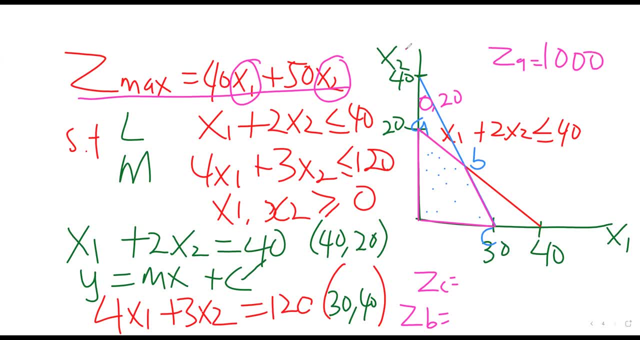 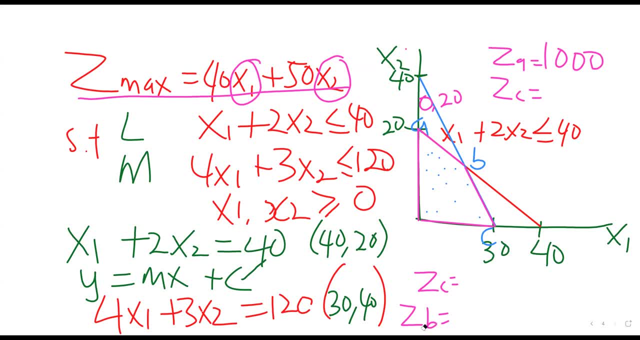 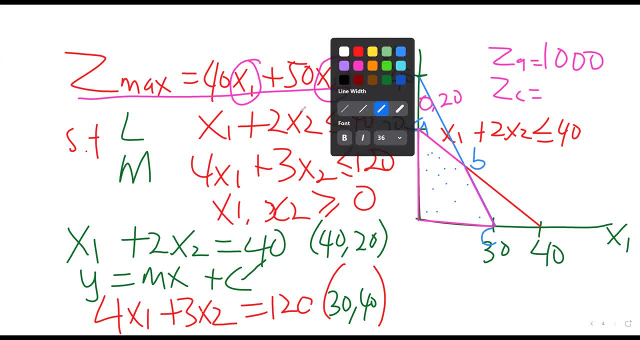 So 30 and 0. So you put the 30 wherever you see the X1,, you put the 0 wherever you see the X2.. What is going to give you the Z value, the profit value, at the point of C? 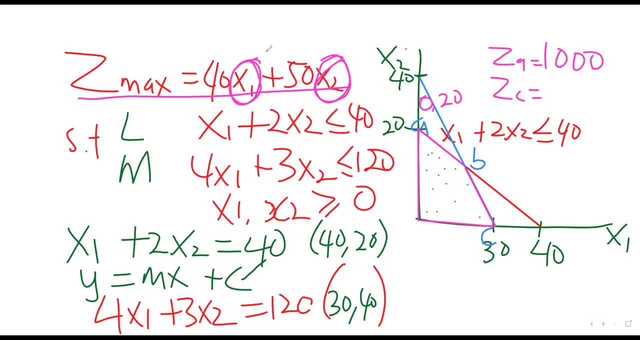 What would that be? Someone should type me the answer. Somebody should type me the answer. Equia, Felix, Samuel Grace. okay, Give me some answers. Excellent, Teofania, Smates, Cyril- these are the names being mentioned into the kingdom. 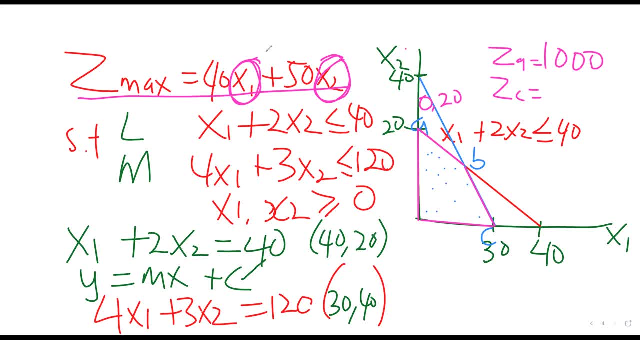 Okay, If your name is not mentioned, that's not good already. That is a correct answer. So you are going to have a value which is equal to 1,002, 1,002.. That is a profit. That is a value you are going to get. 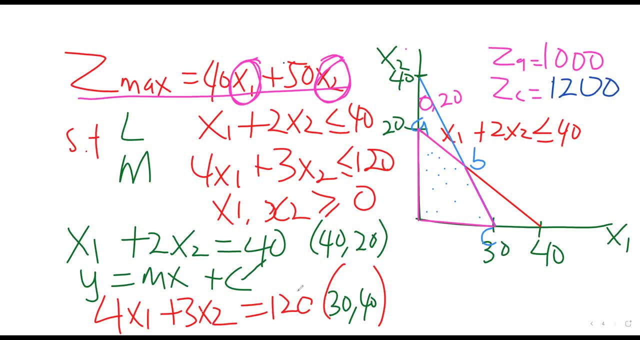 But now let's go to the point of B. Now when you check the point of B B, you see very carefully the point. there is not simple to identify Why? Because when you go to that point of B to get the point, you need to get this line traced. 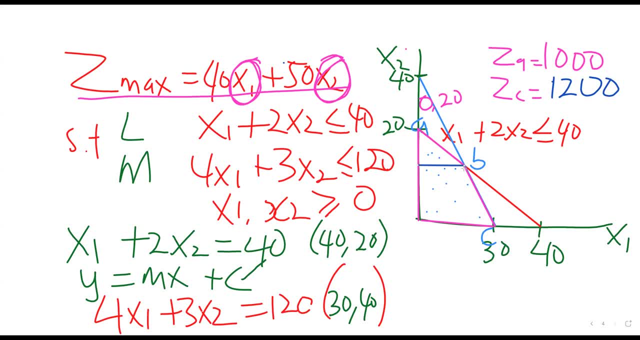 to the X axis to get the X2 value and then trace this one to the X axis, the first one to the Y axis. Okay, Trace this one to the X1 axis to get the value, Because you're not drawn to scale, you can't easily get a value. 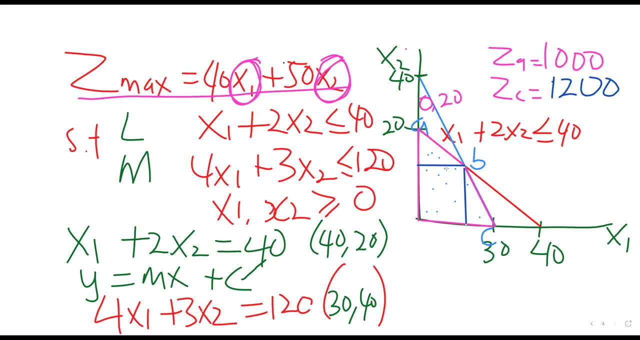 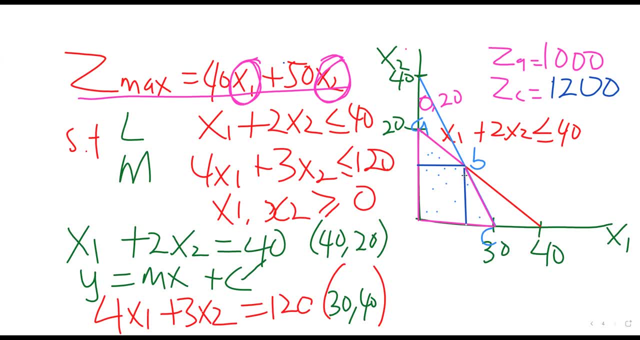 Any time two lines are intersecting, you can use equation or simultaneous equation to solve it. So that means that we need to go to these two- okay, these two numbers constraints here, and then go and handle them. Okay, Go and handle these ones the way they're supposed to be. 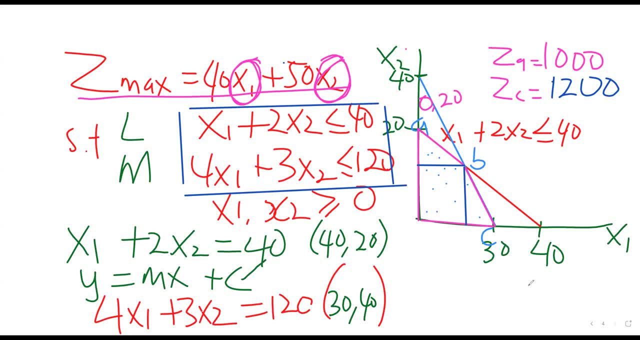 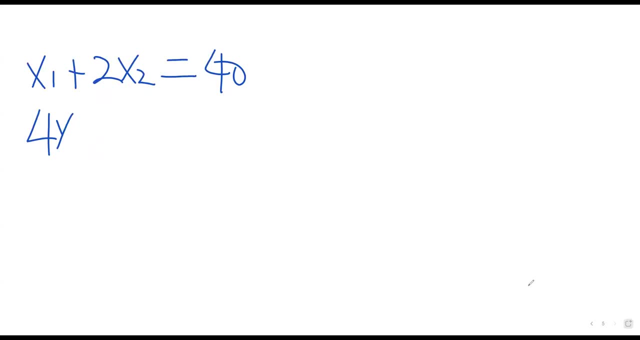 So I'm going to go back and then rewrite these two and solve it simultaneously. They are x1 plus 2x2.. I'm gonna use equal to as a gauge to just solve it quickly. That is equal to, then 4x1 plus 3x2, equal to 120. 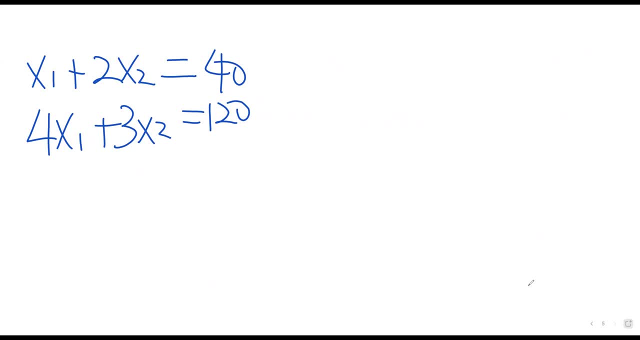 Simultaneous equations simply will require you that, using substitution method, you can call this equation one and you can call this equation two: Hey, go and befriend your little sister and your little brother or mother. And yet easy, you gotta go to them and go tell them that. 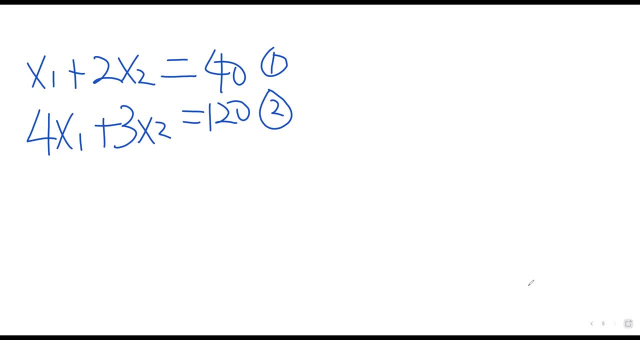 hey, hey. I love you so much. I used to beat you up, but this is not a friendly time. This is a serious time. I beg you, I will buy you ice cream. This is the time I need you to help me. 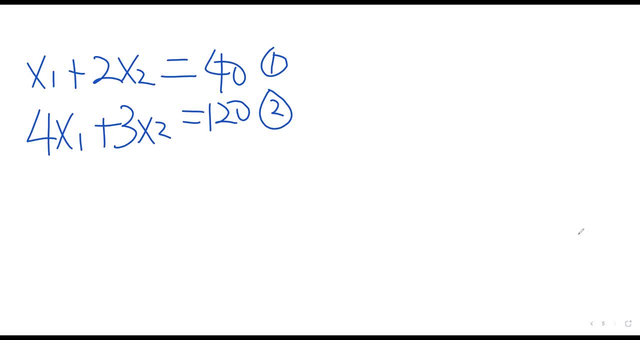 with the akiola mask, The simultaneous equation: I've been seeing you doing planks. If it is your child, go and actually beg your child to teach you akiola And, to be honest, for me to teach you simultaneous equation is not a thing. 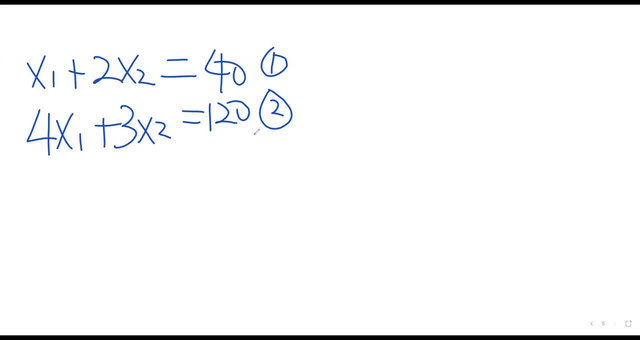 So just get akiola book and just solve the first 50 questions on simultaneous equation. Okay, All right, So let's see how we'll do it. It is the way you learn how to do it that is more important than just showing the answers. 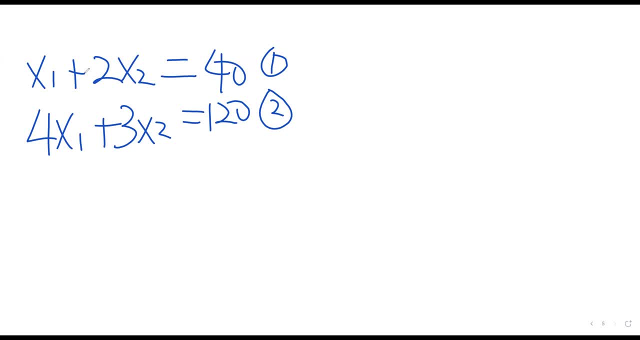 So first one is that you move. you move this 2X to the right hand side. That's what you do, Okay, You move the 2X from the left hand side to the right hand side, That's it, And you'll be left to the X1.. 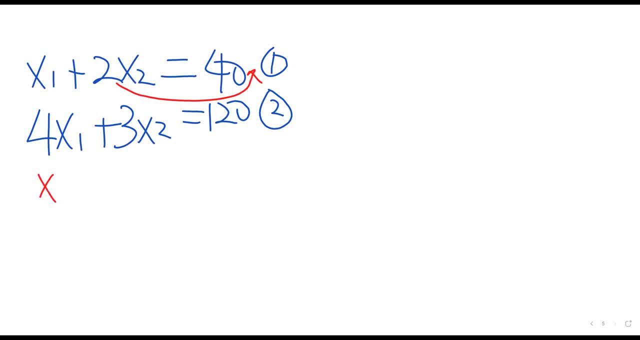 So you have X1 equal to the 40 minus 2X2,. why it is minus? you know it already: Any time something crosses the equal to sign, it turns to minus. Now this becomes your equation. So what kind of equation is this? 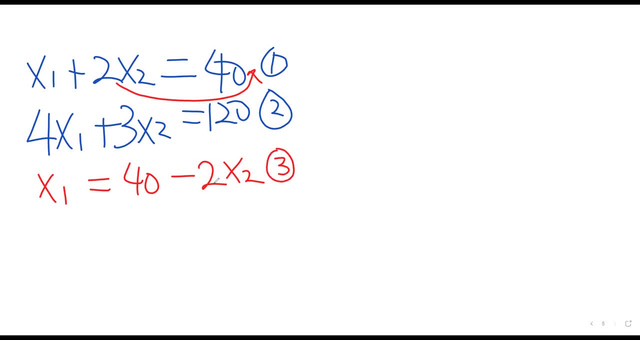 Remember this is前回 jewelry assignment right: The MyYardK しうocky大阪lan贬任工散录 3.. And all you now have to do is to drop this, for you see, it says that wherever you see. 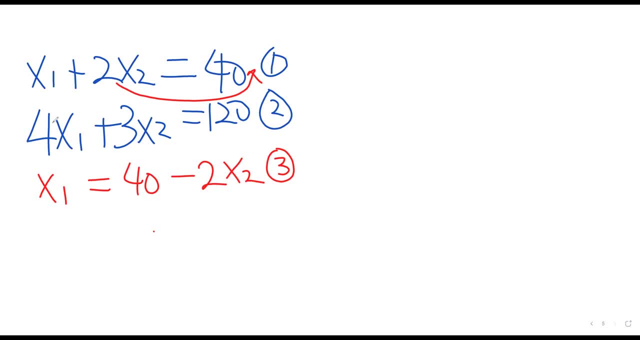 x1, it is 40 minus 2x2.. So go to your second equation, which is equation 2, and wherever you see x1, drop that 40 minus 2x2.. So what is the x1?? Well, it is 40. into bracket the. 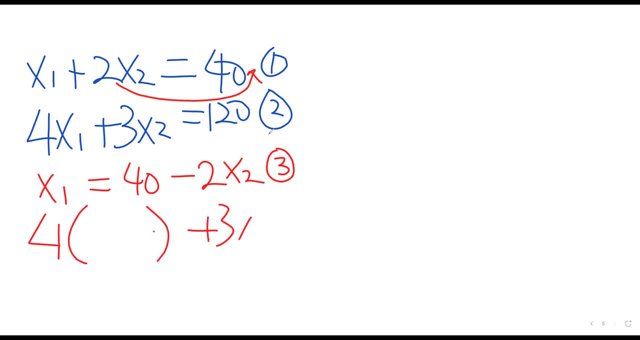 x1, and then plus 3x2, equal to 120.. And what is supposed to be into the bracket? Well, it is that function in equation 3, which is 40 minus 2x2.. Now, this is a factorized. 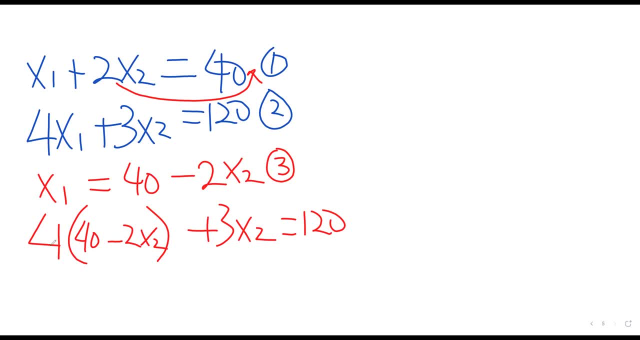 equation. so you've got to, you know, expand it. Expanding it means that you multiply the 40,, 4 by the 40, and then 4 by the 2, okay When you do 4 times 40,. 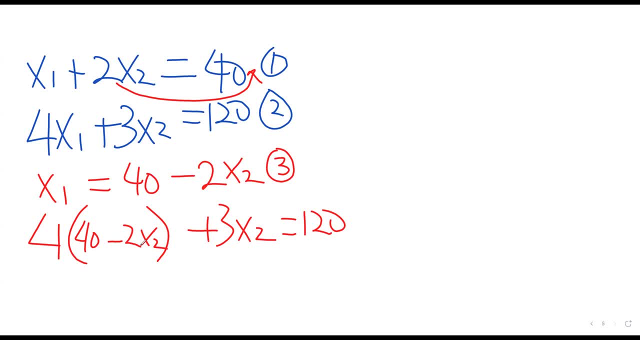 that is going to give you 160.. And when you do 4 times 2,, that will give you 8x2.. Then you add your plus 3x2, equal to 120.. Now you group like 10, the good old days of grouping like 10.. Now 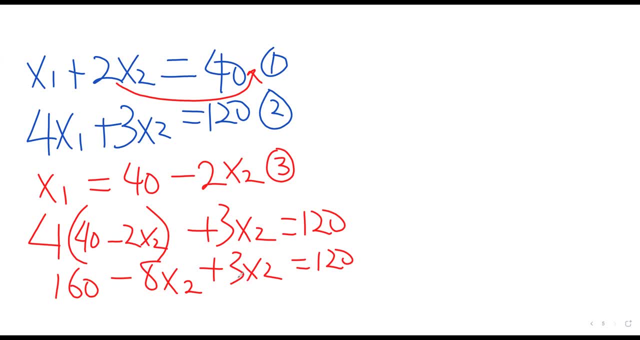 you can see that this is minus 8 plus 3, because they are all x2, x2.. So that will give you minus 5x2.. Okay, Then you go into the equal to sum. The equal to sum, you have on the other side 120 minus 160. 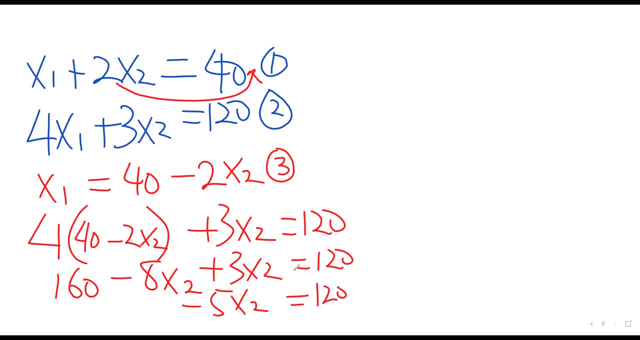 And because it's 120 minus 160, that will be minus 40. So you will have minus 5x2, equal to minus 40, okay, Minus 5x2.. I'm just going step by step for a reason. 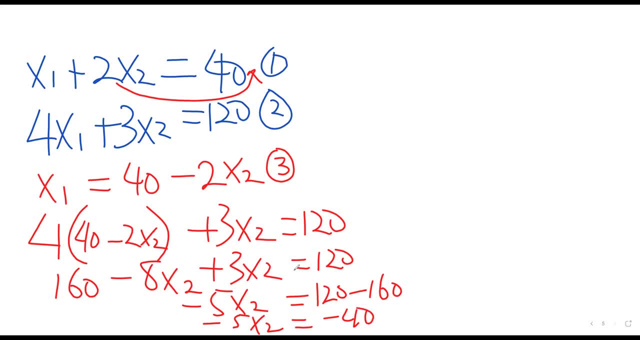 Close to minus 40. Because they are all minus, minus, you can kill the minus and now you'll be left with 5x2 equal to 40. You divide both sides by 5.. You divide both sides by 5.. 5 cancels 5.. 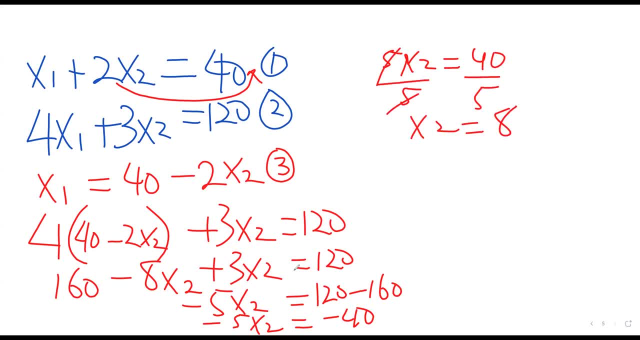 x2 is equal to 8.. That is 40 divided by 8.. So that is the value of x2.. So you have the value of x2 sitting down here Now. remember your equation 3? Remember that equation 3?? We can find x1 by 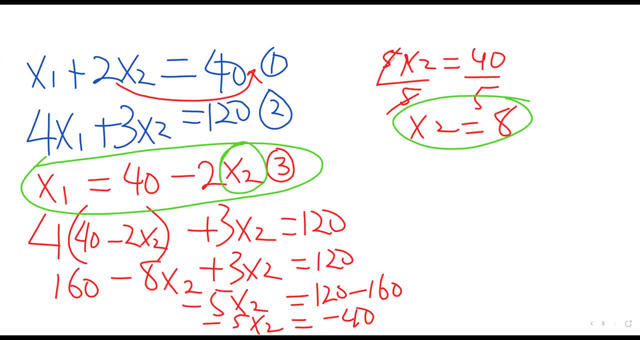 dropping the value of x2 right here, By dropping the value of x2.. So let's rewrite that equation 3.. When you rewrite this, you're going to get x1 equal to 40 minus 2x2.. But we know that x2 is 8.. 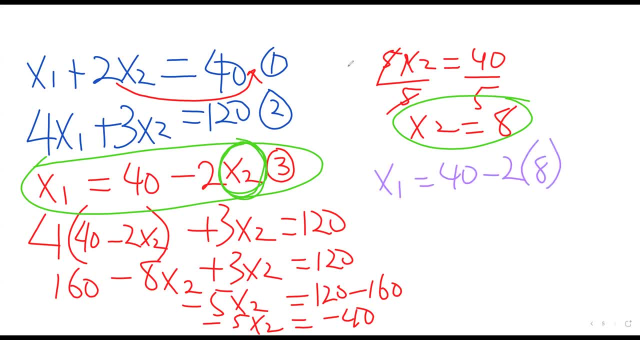 So drop in the 8. And that will give you 40 minus 16.. 40 minus 16 will give you 24.. Remember, x1 is Fanyugo. okay, So this is actually Fanyugo. This is a decision variable for Yugo. 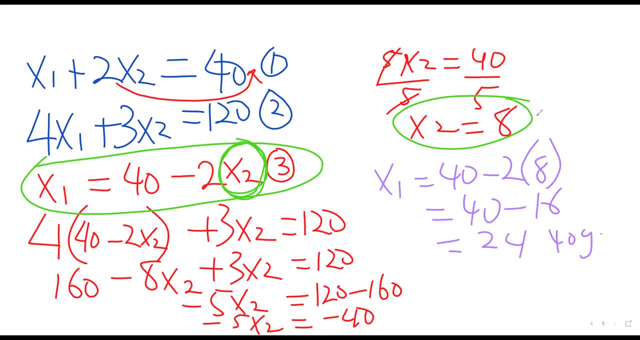 And x2 is Fanchoco, which is what you have up there. So this is actually Choco. These are your decision variables. okay, So now we know the coordinates, We know the coordinates of B. Now, remember, this is not necessarily the answer, We just use it to find the coordinates of B. 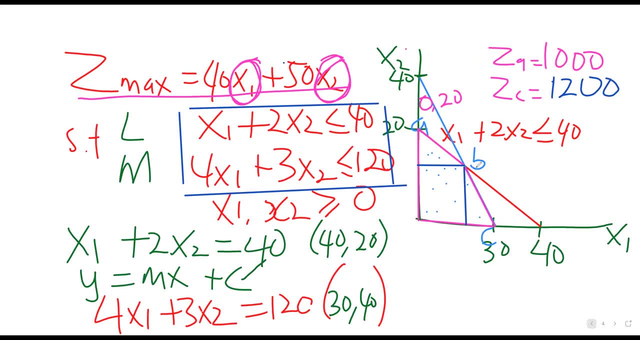 So now we know that the coordinates of B here are 24 for the x1 and then 8 for the x2.. Ladies and gentlemen, do you remember what I told you? How do you know the one that gives you the optimum profit, the best profit? Well, all you got to do is to substitute. So we said that. 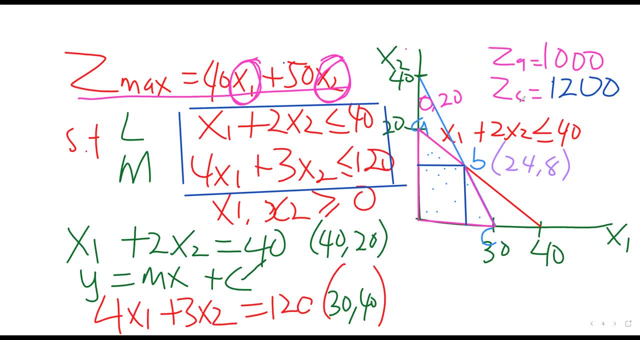 we find the z at A to be 1,000.. We find the z at C to be 1,002.. Now let's find the z at B. Okay, So you're going to put the 24 under the x1 that you found. okay, So it's going to be. 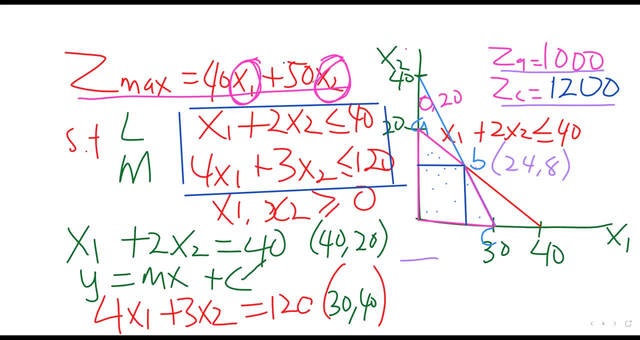 40 times 24 plus 50 times the x2, which was what 8.. These are the numbers. They are 8.. So 40 times 24 plus 50 times 8.. This is where your calculator should be your friend, And that would be 1,360.. 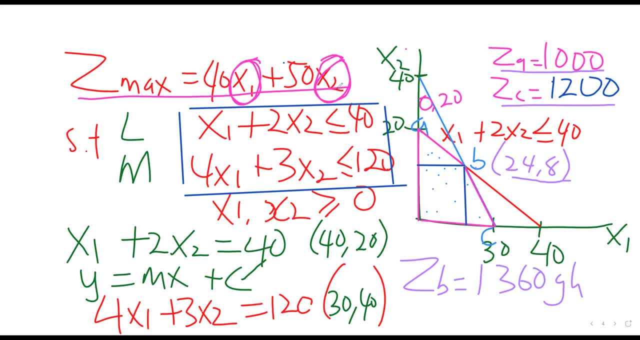 Angli. Dan is serious now. So now we know— we know the values. okay, We know the values of each one, The- how much profit you're going to get at each vertex, At each corner point. We know it. It is not just writing the answer, But you know it in the enquanto. 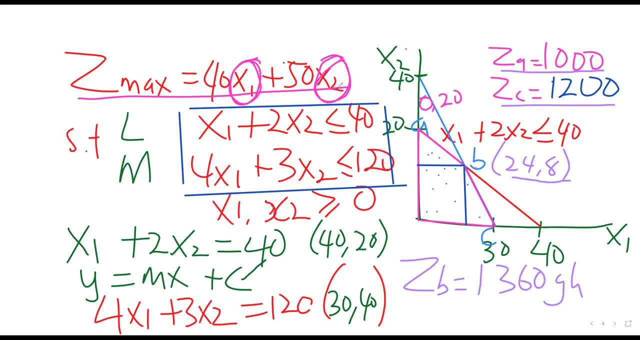 You know it in your heart of heart. You did it by yourself. You didn't wait for someone. You didn't copy your Opel. you didn't copy. You decided to go along with me and you find the position in the ceremonial language. You didn't write the answer. You made that selfish decision. 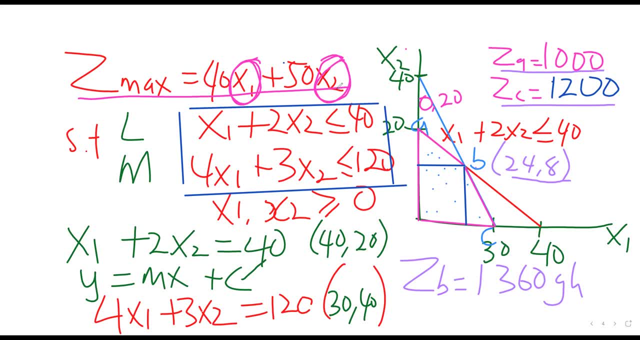 So now you write in theton status You draw up e. I have put the equation Where d, the 18th in botanics yourself. The knowledge was oozing out of you. Your entire molecular structures was having that 1360 inside of you already And you got to follow the tip. Now which one is going to be the optimal? 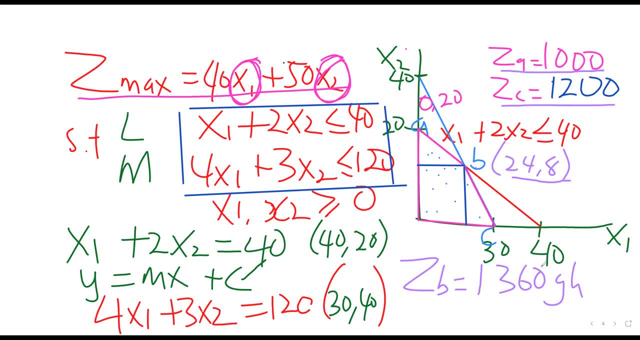 solution point. It is the one that gave us the highest profit, And that one is point B. So you can now come to your conclusion and then say that Pharma Ghana Limited in order to produce a profit of 1,360 Ghana cities in order to generate that maximum profit. 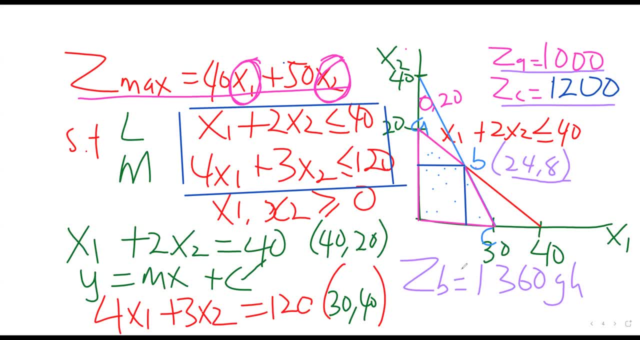 the highest profit of 1,360 Ghana cities. it has to produce 24 sachets of Pharma Yogo and eight sachets of Pharma Yogo to maximize that profit. Now you are putting in numbers. This is your advice to management, Because you give them managerial advice and you tell them that 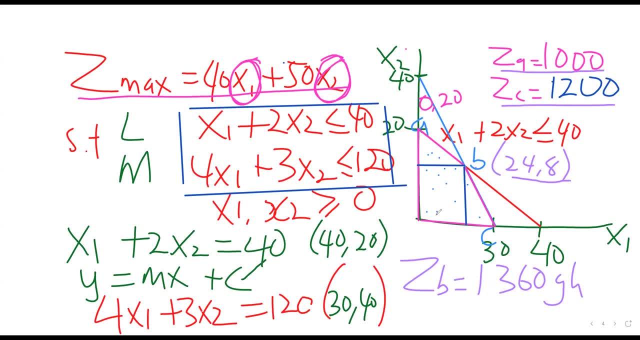 And this is how you do it. If you can observe carefully, I didn't go through all the mumbo jumbos regarding the ISO profit, shifting the ISO profit up and down and all of that. You see, I left all of that. I've made it quite simple for you to be able to identify. 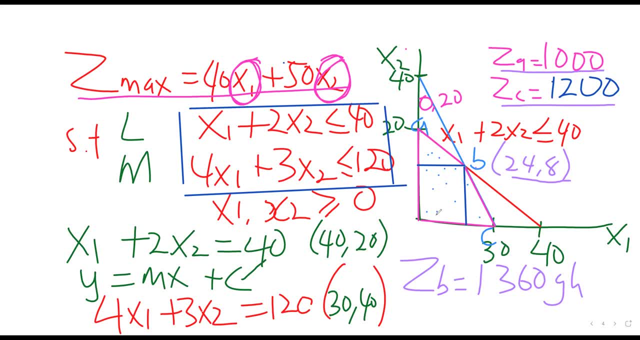 Now, that is not to say that you couldn't have used a graph to do it, But the thing is that sometimes you are not only using the graph, but you're also using the mathematics alongside the graph to guide you. So the optimal solution point is there, And that one is also one of the vertices of the quadrilateral. 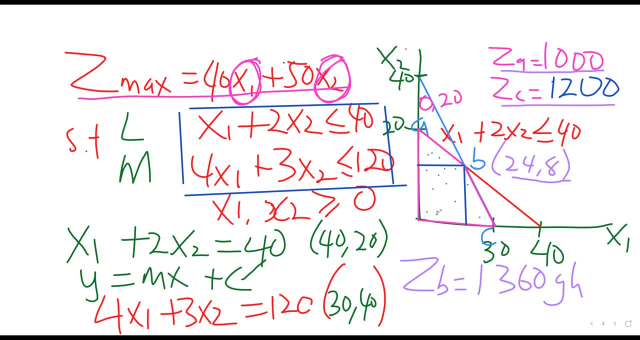 And that one is also one of the vertices of the quadrilateral, And that one is also one of the vertices of the quadrilateral, and so it is within the feasible solution. it's within the feasible solution, okay. now, if you don't understand something here, you let me know. this is why you gotta raise your. 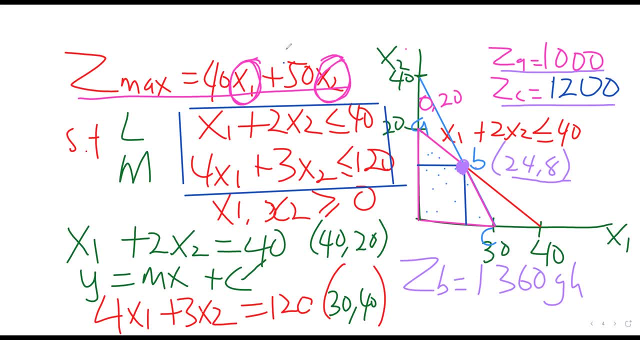 hand, if you don't understand something. something didn't work out the way you want it. this is where you are. other than that, let's move on. you have been able to find the profits, okay, so you've got some people with questions, okay, so let me start with: uh, uber, uber, do you have a question? yes, let's. 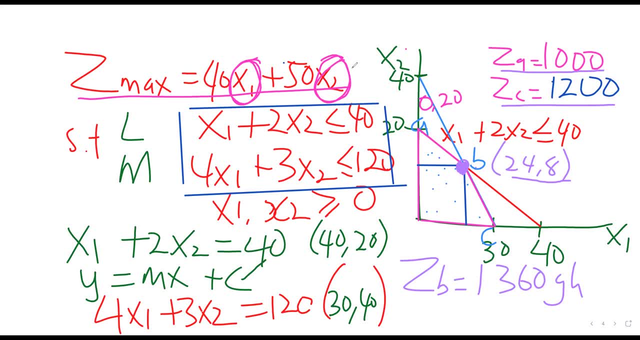 go. yes, but thank you very much for astounding and excellently, but my question is based on the three kinds of constraints, please. uh, you touched on the second one being mixed constraints. please could you kindly explain that a little for me, please? okay, so i will talk about a missed constraint. 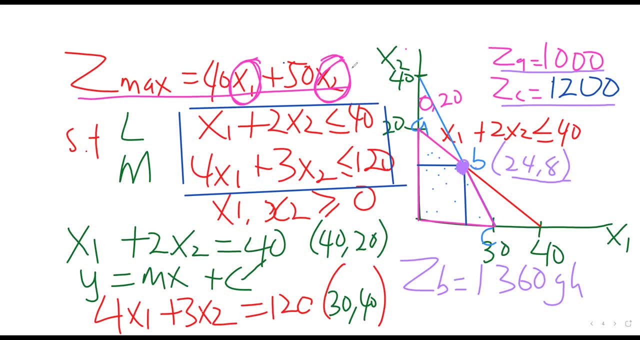 in the next few ones. we are going to do so when we get there. i'll handle the missed constraints no problem at all. i never used a missed constraint. it wasn't part of the constraint here. here we had labor constraints. it's a resource. we had milk constraints. it's also a resource, not mix. i'll talk about mix. 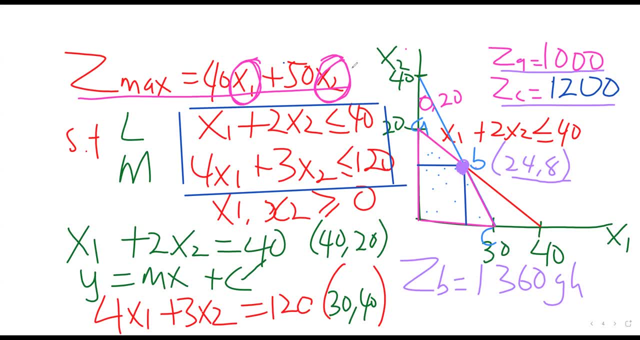 when we go into the irregular types. let's go to melody. melody, you have a question? yeah, not a question, doc, please. i actually sent you a message. i wanted you to slow down a bit for me so that i could grab it very well. well, i can tell you that i've been able to slow down. 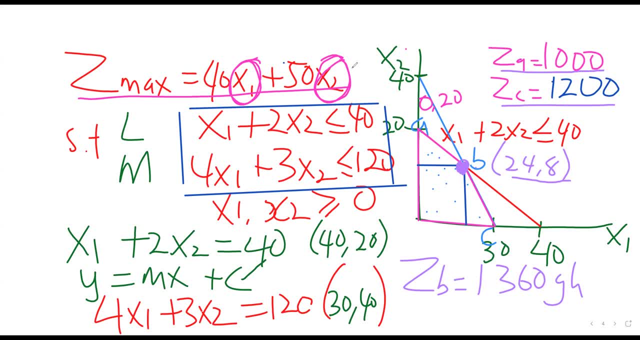 significantly. so when normally you don't grab it that well that this is the time you ask me, your grabbing, not grabbing well questions, but then you have. you have the video as well to go and look at it, so the video will also help you significantly. okay, vincent, let's go. 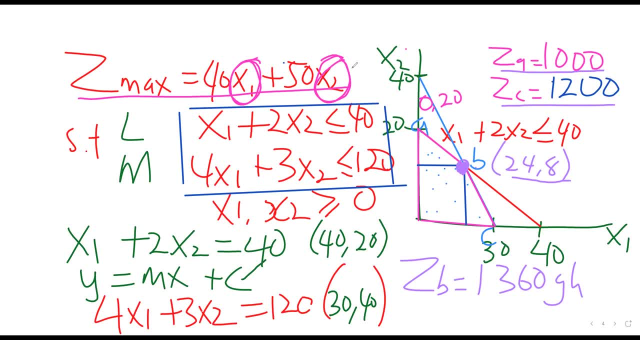 to vincent? no, please, i wanted to find out. and for the simultaneous equation, doesn't matter the method we use. no, it doesn't, just stick to this one. oh no, anyone in the way you're comfortable. okay, you know what. all right, so let's move on. let's move, because they are exciting things to 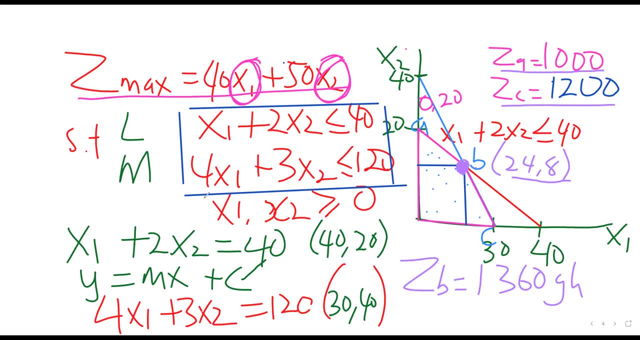 to detect from here. somebody says, uh, please, uh, all of you who are new, okay, don't worry, if you are new. somebody says he's new, he means that he's missed the previous lecture and all of that. it doesn't matter at all. just go watch the video once. i guarantee you, by the time you watch the video three times, a three times just. 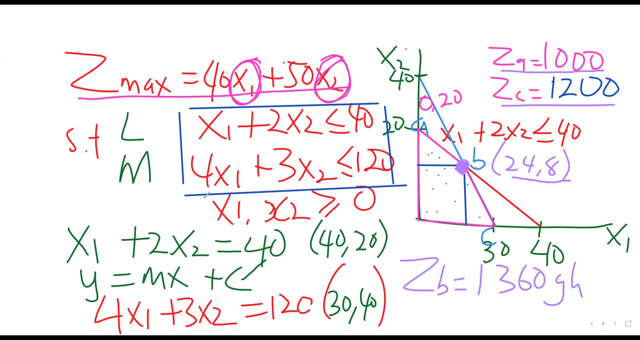 three times. you know how you drive from your workplace, your home, to the workplace, and you spend about an hour in the traffic. sometimes it's a lot of work. just play the thing in your ears. or when you come home one hour before you go to bed, use it to just listen to the video. 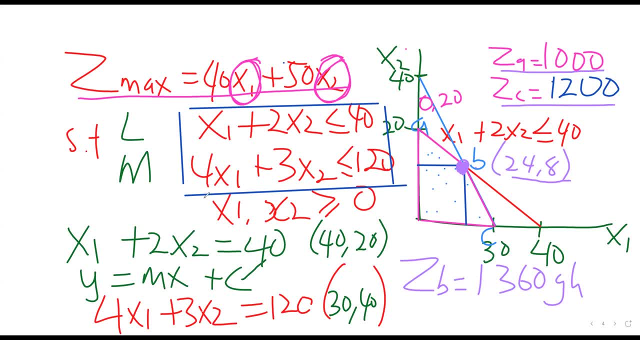 okay, or one hour before you wake up. wake up earlier than that and then use it to what you get it. the only reason why a person might not get something like this is because it's not sat down at least for an hour to look at it. but it's not all the time. you can get it all here, not all of. 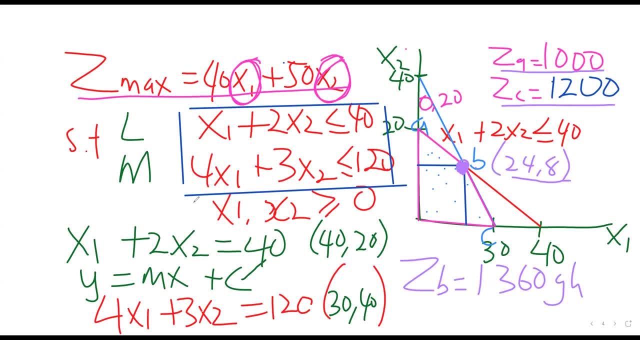 you will understand all of it here today. it doesn't happen. i don't know how that should happen anyway, because this, this has taken people time to write a book, so take your time. not all of most of you will understand it, but not all- i mean most of you will understand it immediately. 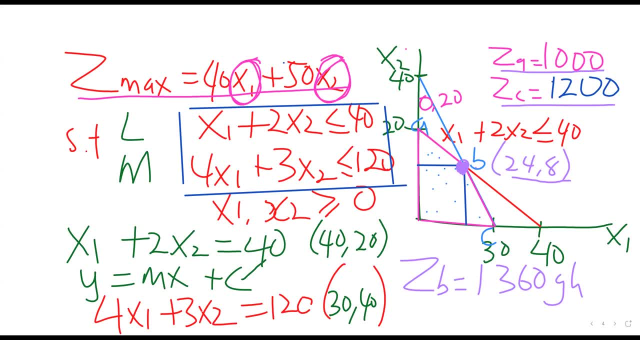 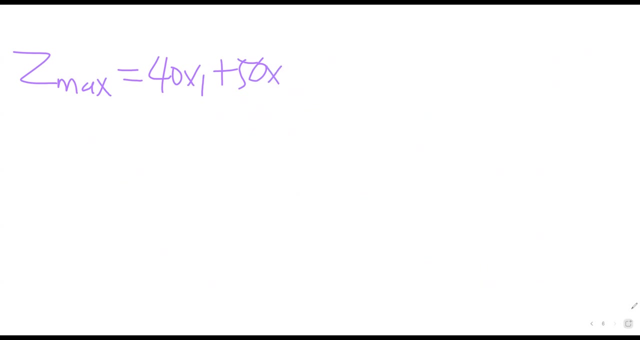 but not all of you will understand it immediately, but all of you will understand it eventually. all right, now let me read, write the the function for you. the function we have been dealing with is z max. okay, equal to 40 x 1 plus 50 x 2. okay, and this was subject to x 1 plus 2 x 2. 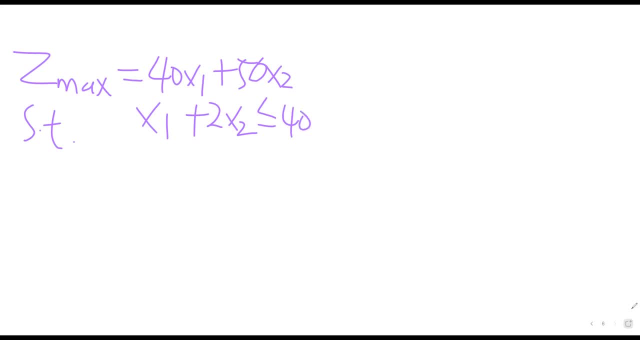 okay, less or equal to 40, and then 4 x 1 plus 3 x 2 to 120 gallons, and then you have the non-negativity constraint. okay, this is what we've been dealing with: all these words, and this is known as a non-standard. 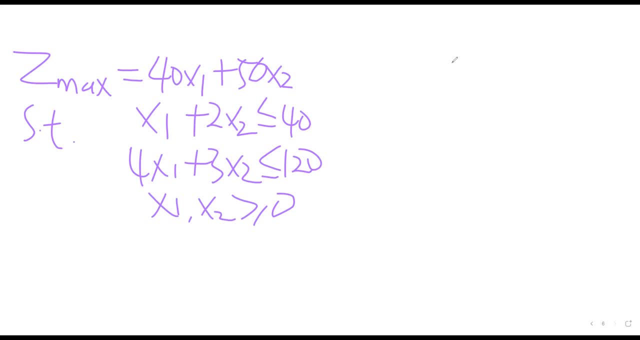 form. the non-standard form non-standard is. this is not, it's not the the. the standard one is a non-standard form. so now one of the things you gotta learn is to convert it to the standard form. okay, you learn how to convert the non-standard form to the standard form. now write this down. these are the four things. 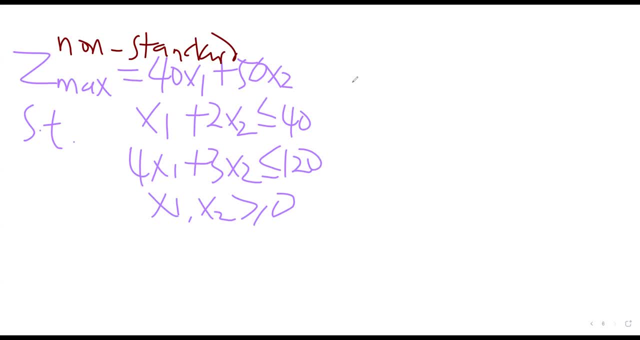 that will happen if you are converting the linear programming problem- lpp linear programming problem- from the non-standard to the standard form one. okay, the first one is that you will add the slacks. you will add the slacks to the objective function as zeros, you add the slacks to the objective function. 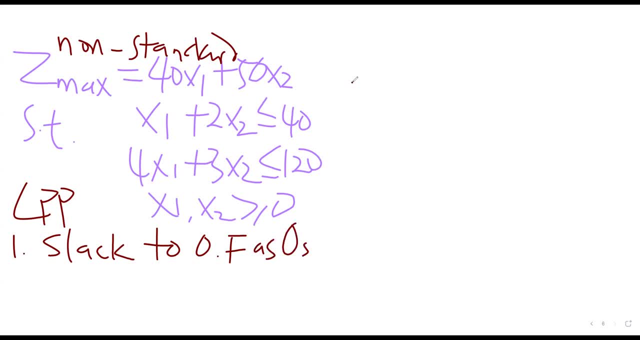 as zeros. but before we move on, let me just quickly explain the slacks. the slacks in any company, in any organization, in farmer journal limited, are those resources that should have been used but were not used. by the end of the production process those resources were not used. 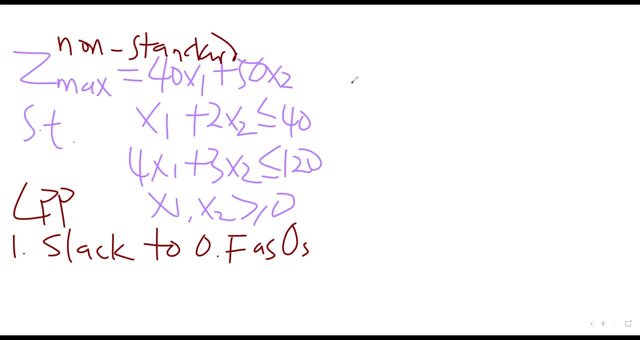 take, for example, a resource like labor hours. how many hours do you go to work and spend time in the workplace? it's eight hours. now suppose you have to use a tower to do somewhat, but you didn't do that. you go to the workplace at 10 o'clock. it means the traffic is lower in that time. you have to use the labor labor zone to to do something, but you might even need to use that. now suppose you have to use that to do some work. now, you didn't do that. you go to the workplace atapa. it means that time you have to do some work, it means that your work's time at demonstratethis one. you need to use the labor work atBEABnalliele пер. lyrics and utilise these. 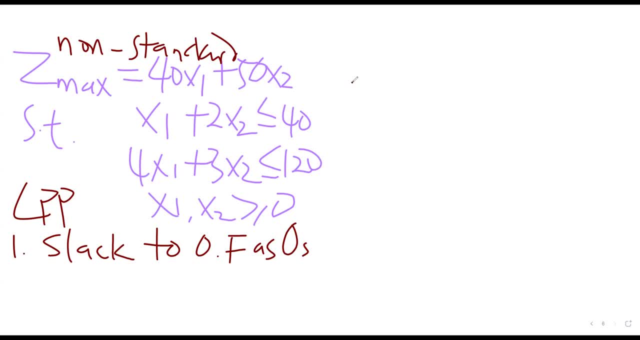 Two hours is already gone. He started reading the newspapers. It's 12 o'clock. Four hours is already gone. So now you have wasted some hours. That is called slacks, So the slack is an unused resource. Another name is that a slack is a wasted resource. 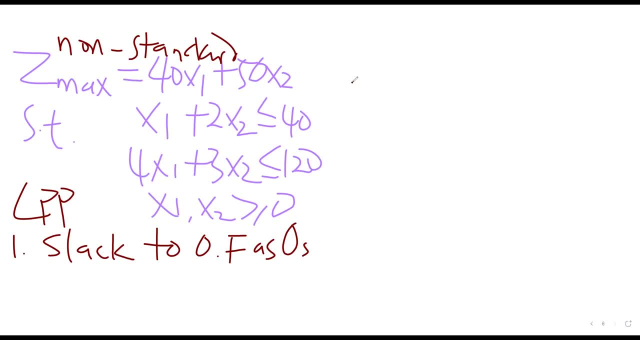 It can be wasted time, It can be wasted material, It can be wasted anything, And in the government sectors, in the government standards, and the private sectors. Now, it doesn't mean that the private sectors don't generate slack, but the government sector generates a lot of slacks. 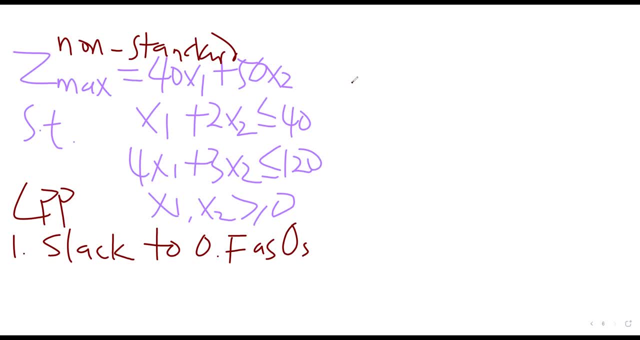 There are a lot of slacks in the government sector, a lot of wastages. People are sitting down watching Cantata and Kumbaya when it is 3 pm Instead of them actually doing some work. So slacks is said to be. 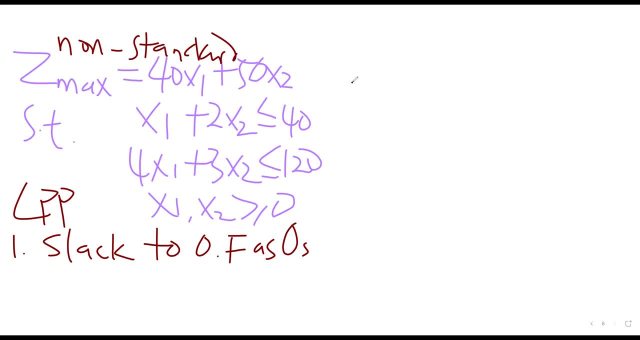 the inefficiencies Put that down. There are wastages, There are unused resources, Inefficiencies generated in the company, And so every resource will bring about a slack. The slack can be zero. That means that all the resources were fully utilized. 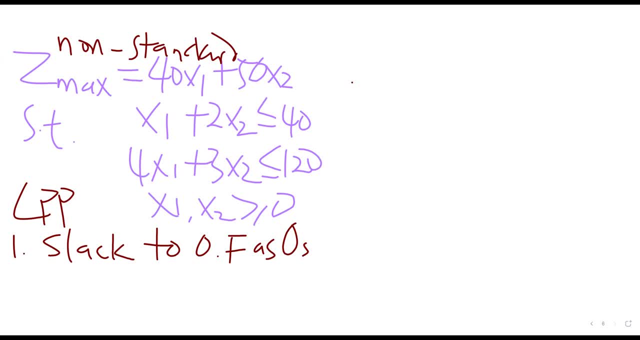 Or the slack can be positive, not zero. Ouch, that is not good, Because once you have slack, it means that some resources have been underutilized or they have not been used, And that is bad for any government, any company, any organization. 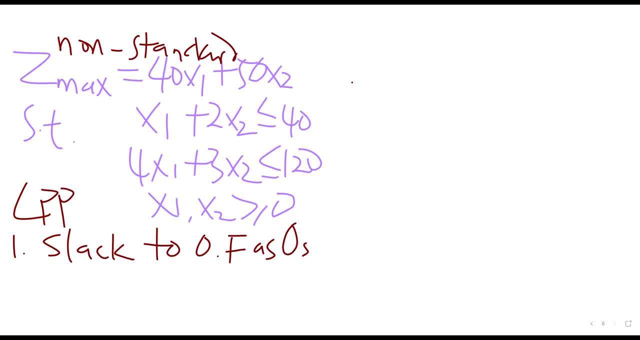 The problem in most countries and in most businesses is that they don't calculate the slacks, And so they are abundant. For example, a company can be said to be the best bank in the country, the best bank in the banking industry, when in fact so many hours were not utilized. 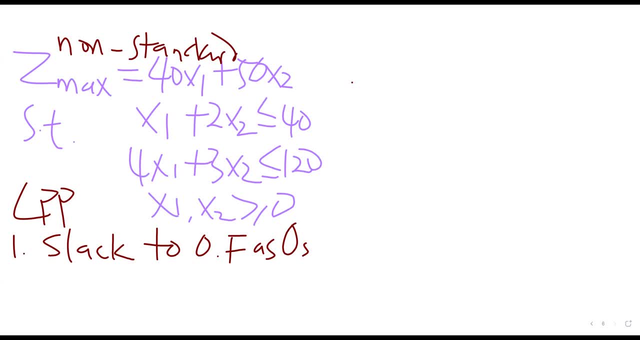 In generating the revenue or the deposit mobilization that was supposed to have been done. So slacks are the unused resources, Slacks are the inefficiencies And you have to take the time to quantify else you are doing as a company. So most of you in the businesses tell your bosses. 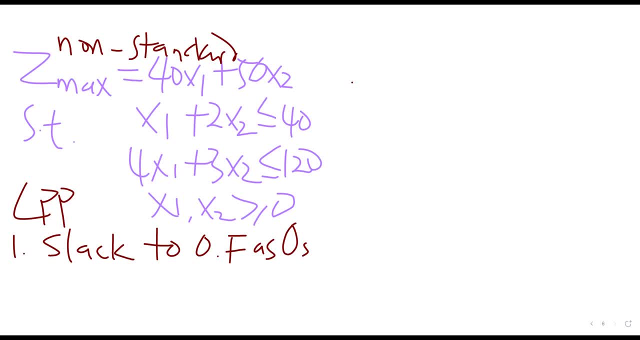 some of you. by learning this course, you'll be able to advise management on slacks. Now, once you are supposed to use those resources and you don't use them, listen here. Once you are supposed to use the slacks and you don't use them, they are gone. 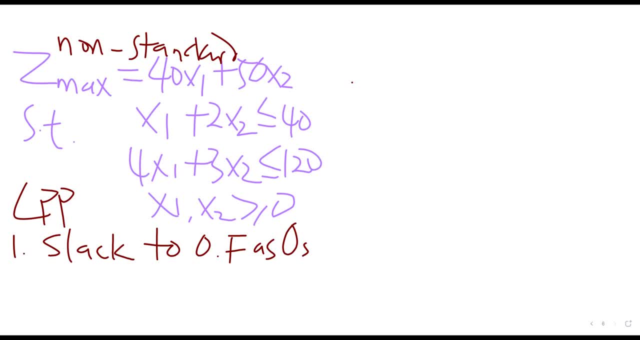 You can't come back the next day and say, boss, please. yesterday I spent six hours in traffic. I couldn't get to the office early And so I want to spend six hours. I mean, you really want to do that. 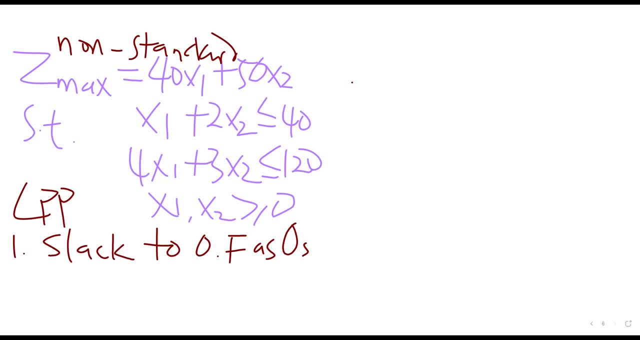 So the slacks? they don't add anything to the profit. That is why in the objective function the slacks are zero. I normally ask you this question in an exam, So if you don't understand it, go ahead, raise your hand. 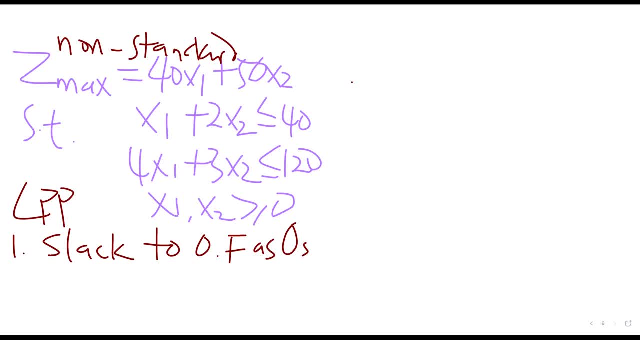 In the objective function, which is the profit function or the objective. the slacks contribute nothing to the objective function, Why? Because the slacks are unused, And once they are unused they are gone. Once they are gone, they are gone. 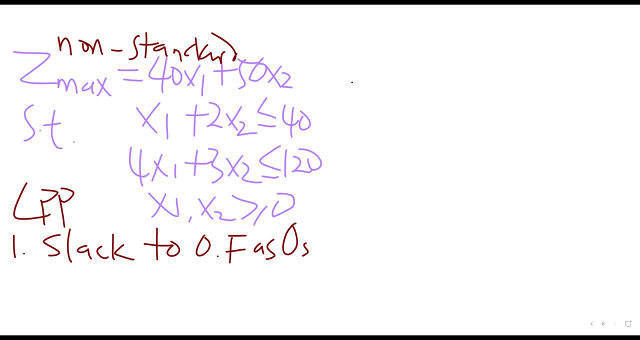 And there are so many. Once you have been inefficient on the job, you have been inefficient on the job Even if you come the next day to come and do that when you wasted the previous one, it's gone, And so the value of the slacks in the objective function are zero. 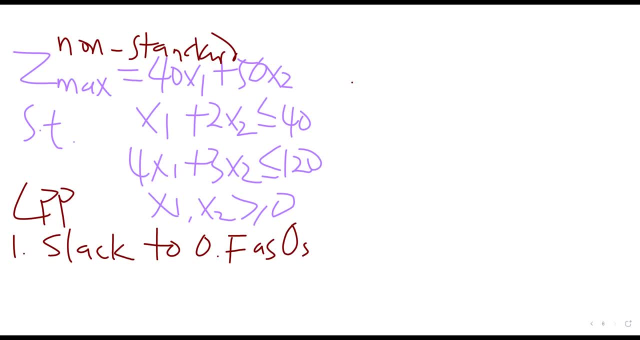 Let me write that for you to see. So if this is objective function Zmax, which is equal to 40X1 plus 50X2, we are going to add the slacks. But listen, the slacks are given a name. 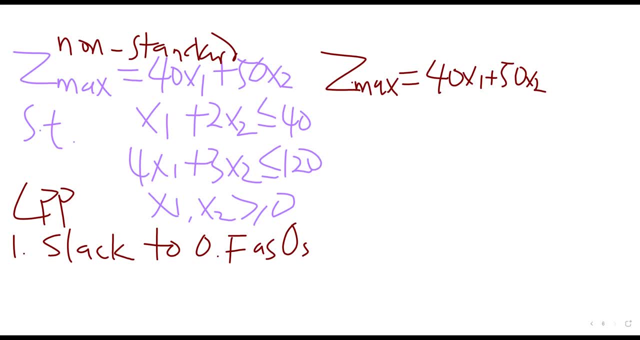 The number of constraints- and that's my next point before I come and add that: okay, The number of constraints, The number of constraints that you have, excluding the non-negativity constraint, okay, The number of constraints will equal the number of slacks. 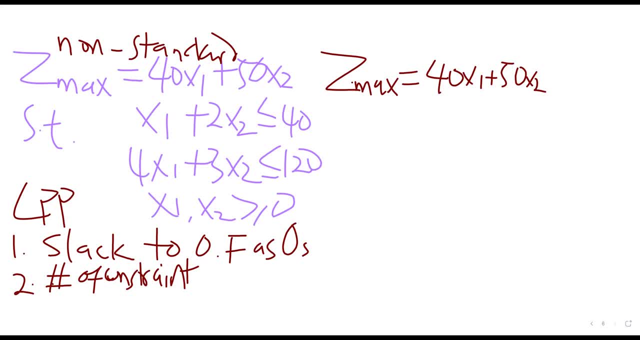 Okay, the number of slacks you need to have. So, excluding the non-negativity constraint, guys, who can tell me What is the number of constraints we have here? Who can tell me that? What is the number of constraints we have? 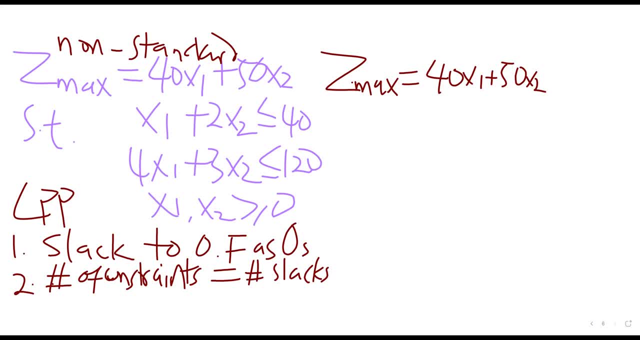 We have two. Good, Okay, you have been very participatory. I like that. okay, So that's two. So how many slacks do you think we need to have in this model? How many slacks do you think we need to have? 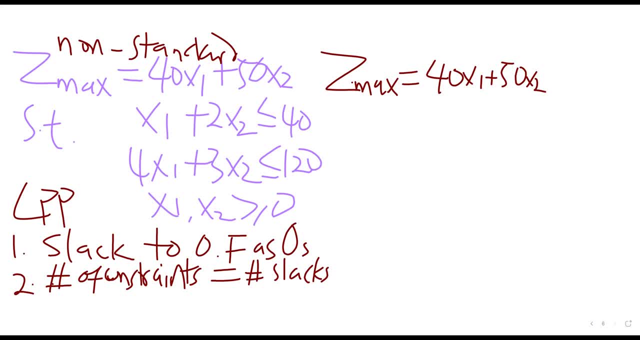 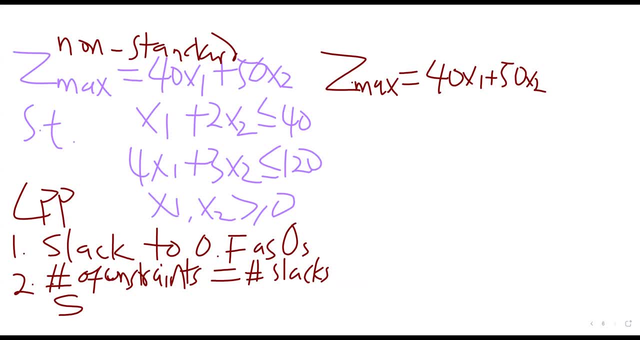 The second slack is called S2.. The third slack is called S3.. And then it's on and on, And because in the objective function we have already said, the slacks are attached with zero, So you will write the slacks as: plus zero S1, plus zero S2.. 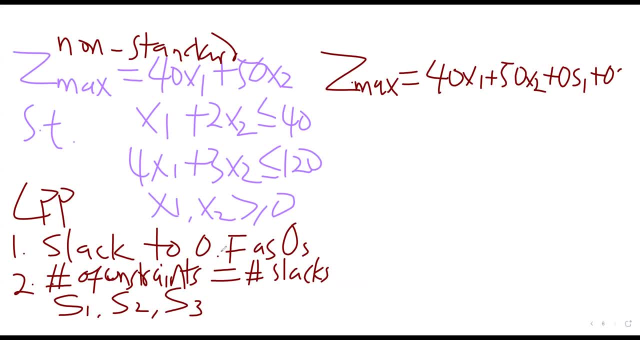 That is how you introduce the function of the function. use the slacks in the objective function. now your question might be: why zero? because we've said that the slash contribute nothing. that's what americans say. the british will say: the slots do not contribute anything to the objective function or the objective value and because of that they are. 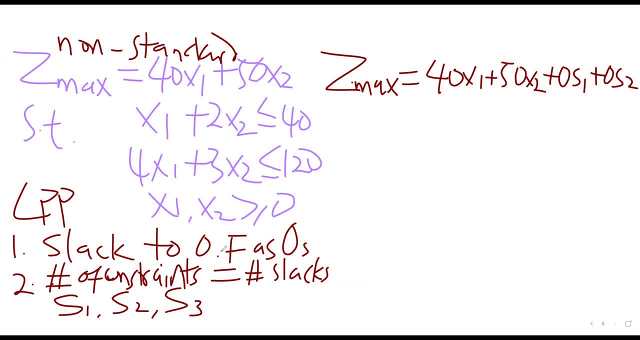 given a value of zero. so so that when you multiply the zero by the s1, you still get zero, which means i contributed nothing. so when you are converting it from the standard form, the non-standard form, to the standard form, that is what happens: the slacks are introduced as zero. then you go to your subject. 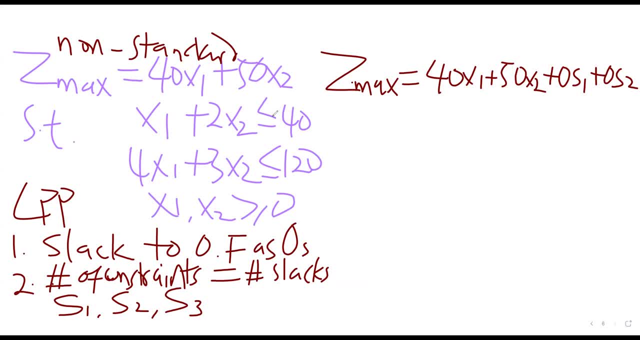 two, which leads me to the third point. the third point is that the slacks are subtracted from the constraints. each slot is subtracted from the constraint- the left-hand side of the constraint. okay, each slack is subtracted, and i'm using the word subtracted because you are dealing with maximization. 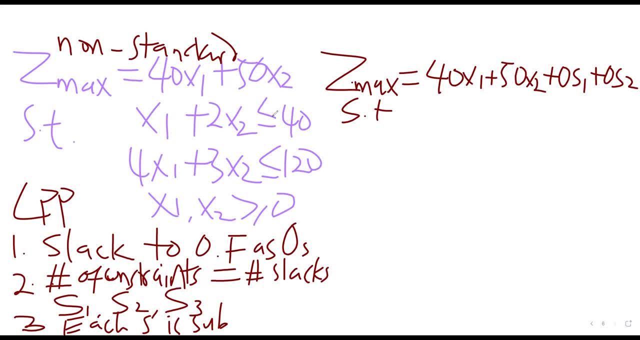 okay, it's subtracted from the left-hand side of the constraint. so what is the left-hand side of the constraint here? well, the left-hand side of the constraint is what you are seeing here, this part there and this part there. okay, and so in rewriting this, you are going to write x1. 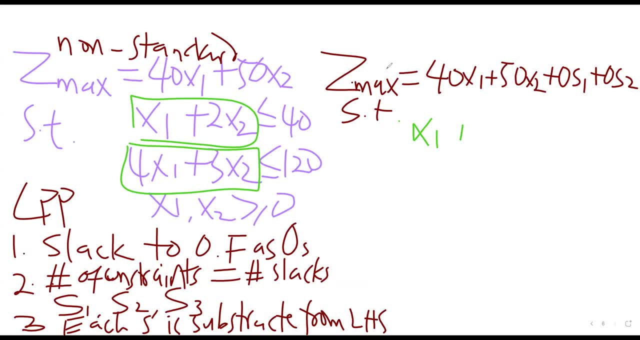 plus the 2x2, then you subtract the first slack, which is s1, and then you convert the inequality to equality. okay, and that is the last part of the rule. the last part of the rule is that in the constraints, in the constraints, the slacks convert the inequalities to equalities. okay, i'll write. 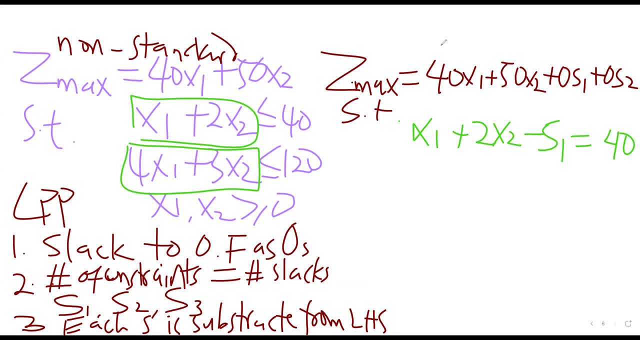 that you should get it in the constraints, the slacks. they convert the inequalities to what? to equalities. so i'm going to let one of you tell me how the standard form for the last constraint is going to be like. who can raise their hand and tell me how would i have to write the, the, the, the standard. 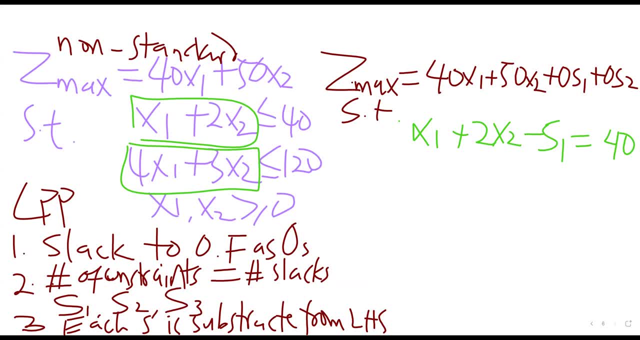 form. okay, so, so somebody, somebody says that i should go over, i should go over the fourth point, so let me write the fourth point. okay, the fourth point is that: okay, the slacks convert the inequalities to equalities. that's all. that's the fourth point. the third point was that each slack is subtracted. 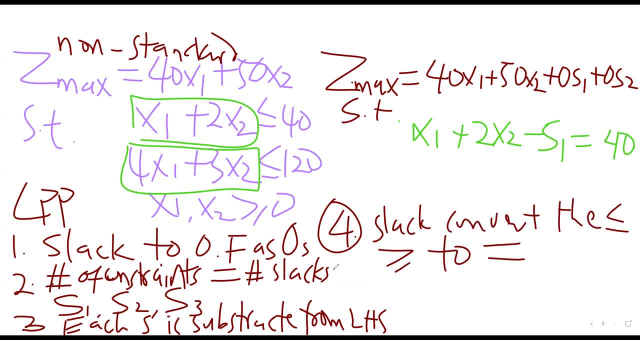 from the left-hand side of the constraint. each slack is subtracted from the left-hand side of the constraint. the fourth point is that the slash converges the inequalities to equalities. now who can tell me how i should write that constraint, given the rules I've just said? 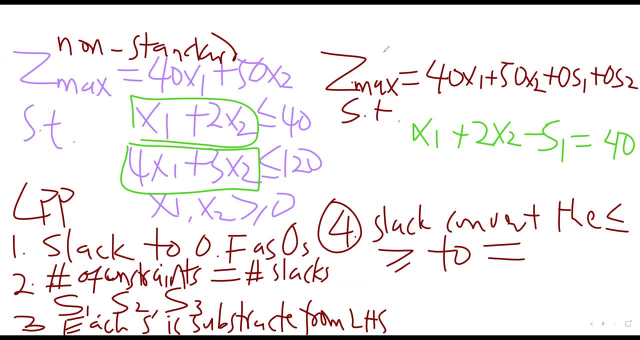 How would you have written the second constraint? Okay, Pankofi Jr said 4x1 plus 3x2 minus 0x2.. I'm sorry you've lost it there. You've lost it there. Who can tell me? 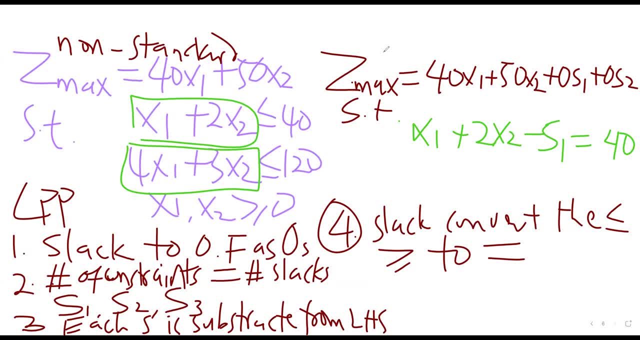 Who can tell me? How would you write that one? How do you write the constraint with the presence of the slack? Who can tell me? Who can tell me? Excellent, Linda, I like your answer: 4x1 plus 3x2 minus s2.. 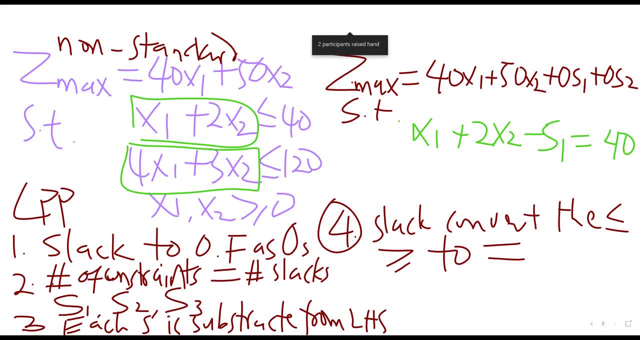 That's the right answer And I'm sure Samuel and Grace and James, all of you are cracking that code. So the slacks for that second one, if you are writing the standard form, it will be 4x1 plus 3x2 minus s2.. 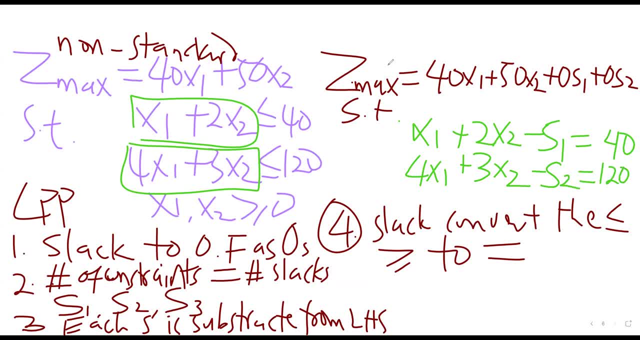 Before you bring equal to 120.. Okay, that is how you. So what it means is that each constraint becomes, you know, gets- a slack. The number of constraints will equal the number of slacks- I've already said that- And each constraint will have a slack. 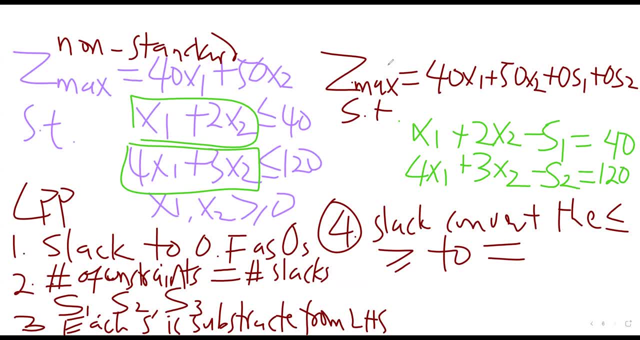 When you are done, there's one more constraint. You don't want to joke with it. There's one more constraint, And that is a non negativity, but this time, because of the slack, you have to add that, So that one more constraint is x1 plus 3x2.. 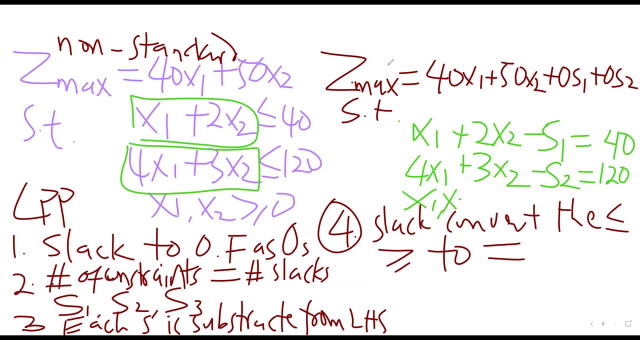 X1 comma, x2 comma, s1 comma- that is a slack. one S2 comma greater or equal to zero, So that one is not equal to zero, That one is greater or equal to zero. So that last constraint is also the non negativity constraint. 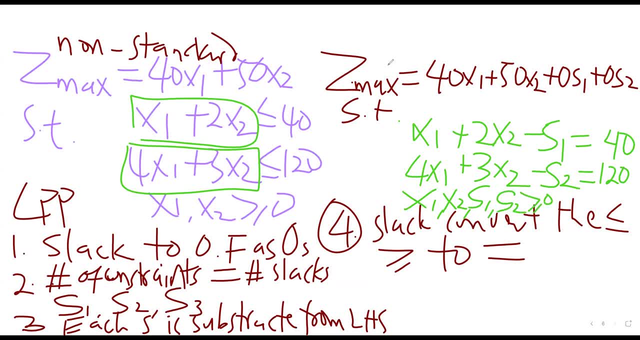 At this time. the slacks have been added. The slacks have been included, So that's that. That's the end. How many is that? There's a lot. Look over time. There's a lot, But we're in the middle of each other. 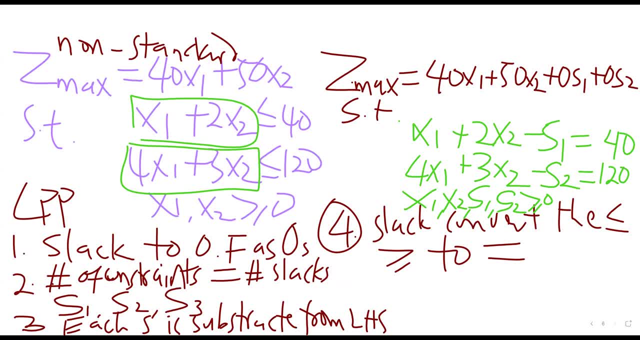 What is the standard form that we have been discussing all along the standard form. So next time I give you a certain equation or I let you formulate a certain equation, I can also tell you that after formulating the equation, you should tell me the standard. 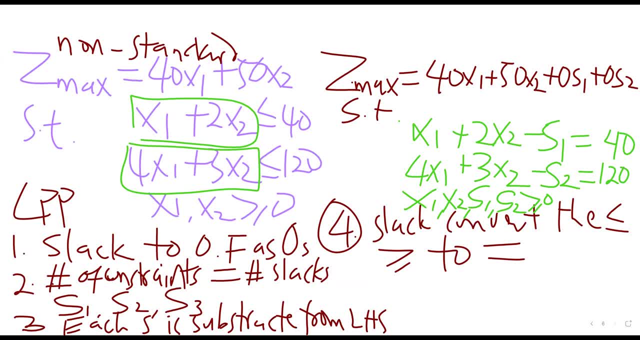 form. Now, how are you going to tell me that All you got to do is to follow those four steps I've given you? Ensure that the slacks are given a value of zero, but in the constraint they are not given a value of zero. 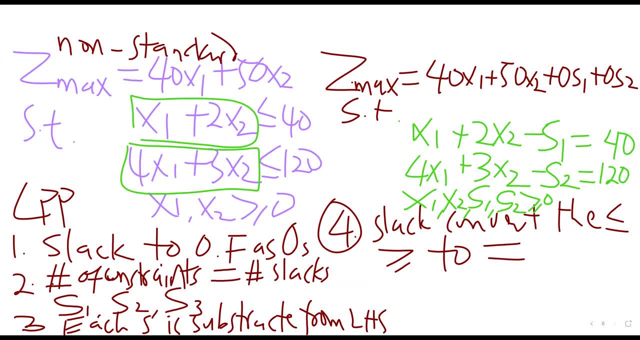 The reason is because in the constraint- remember- they are added to the usage as minus. They are added to the usage as minus, And so you don't have to include them in that. Now I'm going to trick you small to see. 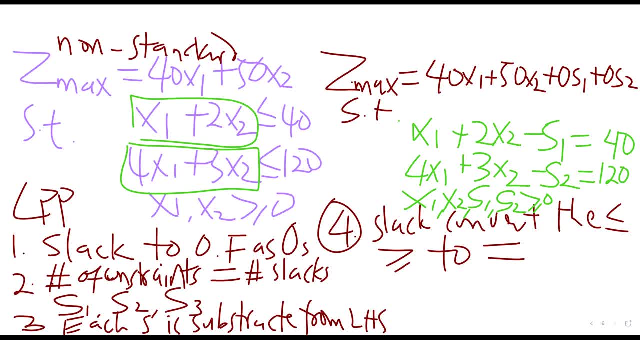 Now we, Our job now is to calculate the slacks at each of the corner points. Do you remember the graph, The graph? Okay, good, Now you remember the corner point. We have point A, We have point A, We have point B, We have point C And the point B. 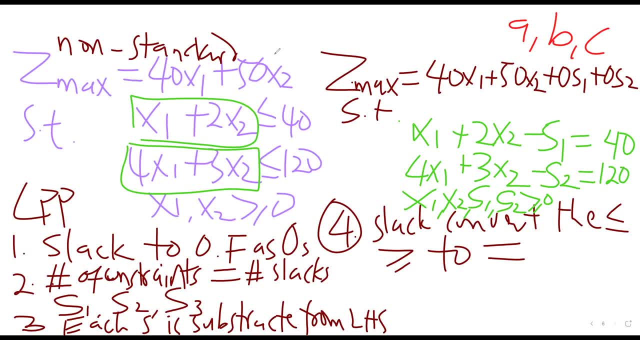 was a point that gave us an optimal solution. point Now, the thing is this, and what I wanted to learn a little bit here is that You should be able to calculate the slacks at each of the corner points. The slacks contribute nothing to the objective match. 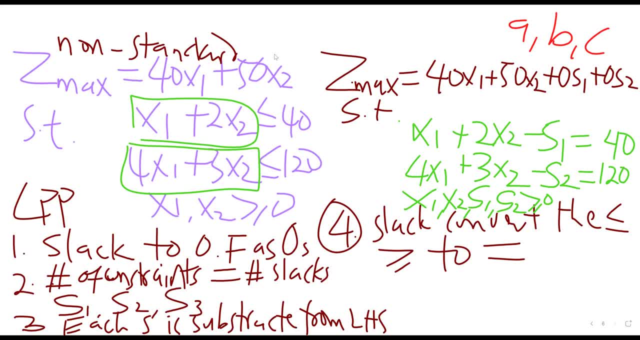 We know that In the standard form. we know that. But what we are going to do is that we are going to calculate the slacks at each of the corner points. So let me just remind you of a few things. The corner point: 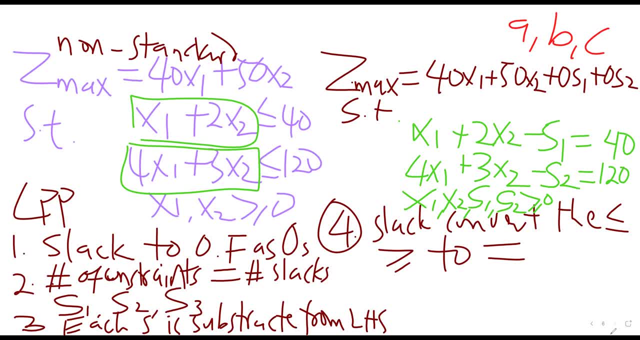 Now, in order to calculate the slacks at each of the corner points- you have to calculate the slacks at each of the corner points. You have to remember the equation. Let me rewrite the equation all over again. The equation is 40x1 plus 50x2.. 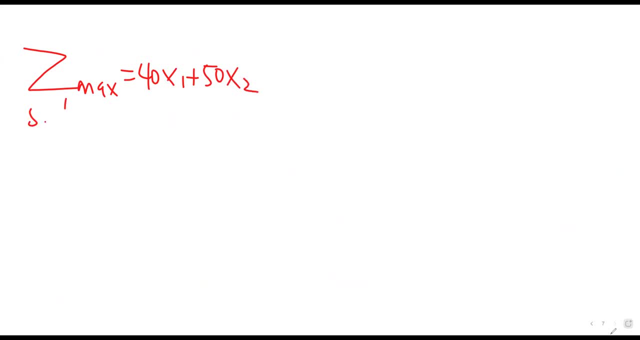 I'm writing the original equation: Subject to x1 plus 2x2 less or equal to 40. Then 4x1 plus 3x2 less or equal to 120.. And then your x1,, your x2.. This is the non-standard form. 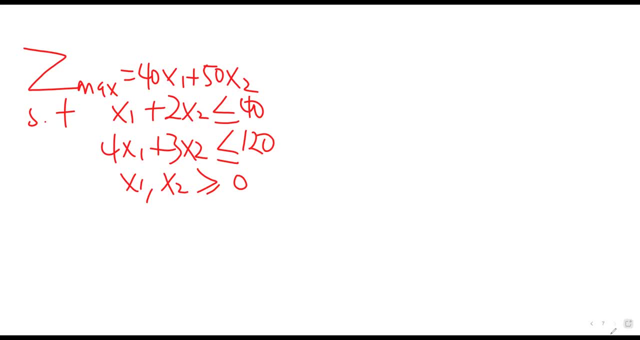 Okay, Now we want to know the coordinates. If you remember the coordinates for each of the points, Okay, I remember them. What were the coordinates for A? Well, the coordinates for A were, you can remind me, it was zero and then a certain. 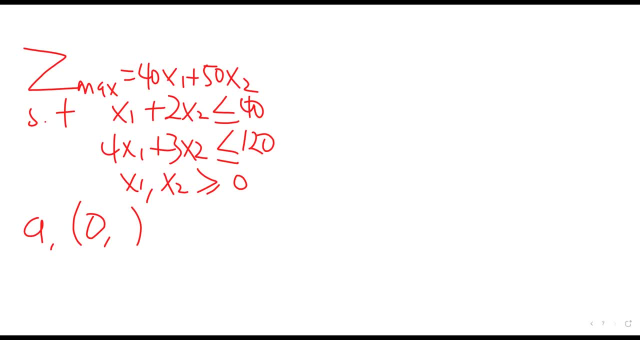 number. I just want to be sure you are following. That is why sometimes I ask you: All right, Zero and 20.. Somebody asked a question. Let me see. It says that Somebody said I should repeat the non-negativity. 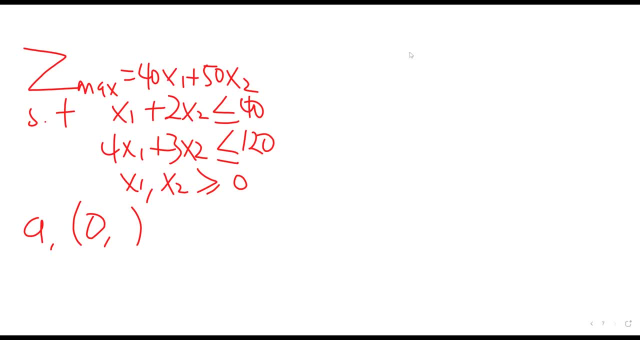 The non-negativity is x1, x2, s1, s2 greater or equal to zero. That is the non-negativity. It doesn't matter which constraint gets which slack. Yes, The first constraint should have the first slack. 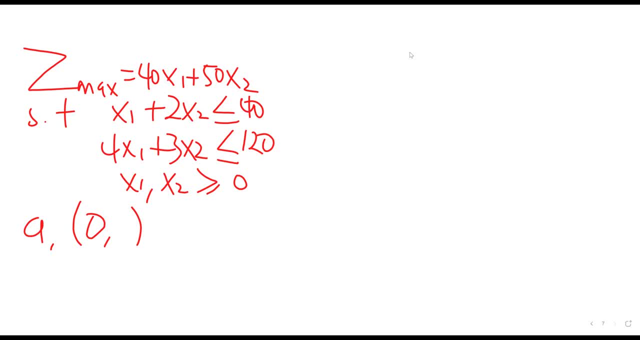 Egan, that is the answer to your question. The first constraint must have the first slack. The second constraint must have the second slack. The third constraint must have the third slack. Okay, All right, So A is zero 20.. 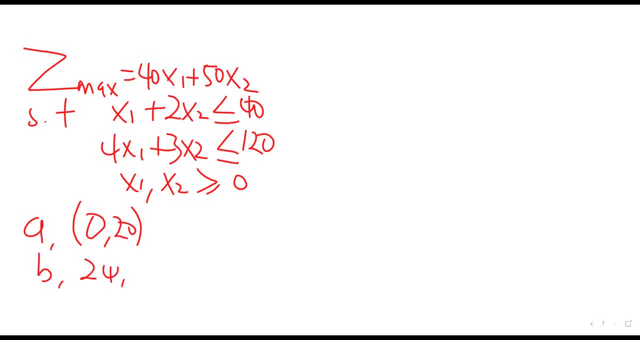 B was 24 and then 8.. And then C was 30, zero. Let me make sure that is correct. Okay, So what you now to do is this: You are going to take A and then you drop A into the first constraint and into the second. 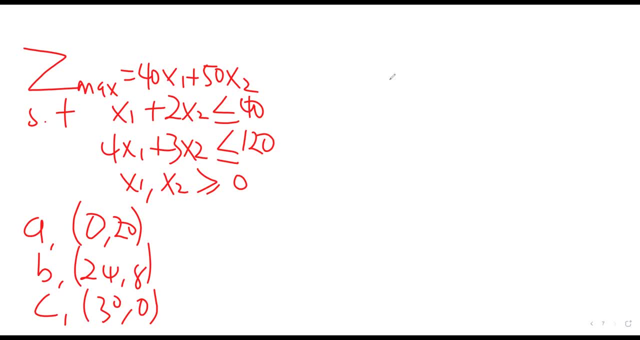 constraint And then you tell me: the slacks I'm going to do for A, You do for B and C for me. So if I drop A points the coordinates into the first constraint, that is, the labor constraint here. 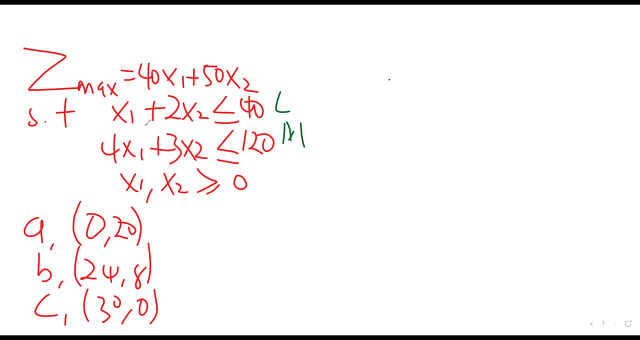 Okay. And then the male constraint, Labor constraint. If I do that, okay, where x1 is zero And x2, look at x2.. Okay, So in this case x2, I'm going to put in the 20 there. 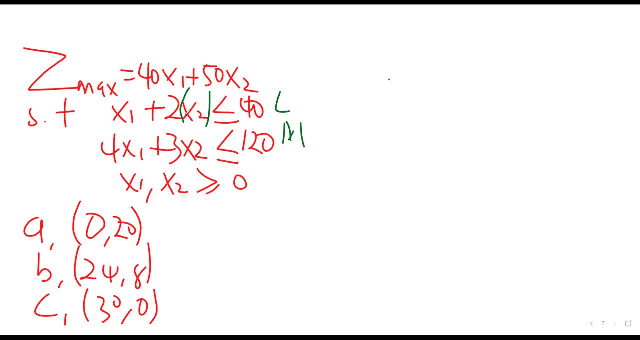 If I do that, then it will mean that you will have 2 times 20.. And that will be equal to the right-hand side, isn't it? That will be equal to the right-hand side. So is that s1 will be equal to what? 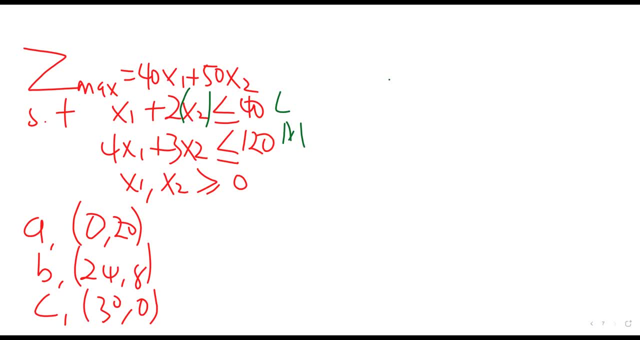 The slack there will be equal to what? For that constraint, For that constraint, labor, the slack s1 will be what? Zero? Okay, So now x1 will be zero. What about s2?? Okay, For that same. you know, let's go to the male constraint. 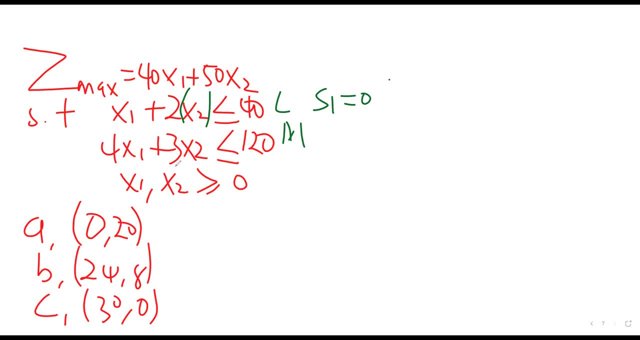 Okay. So when you go to the male constraint, you drop the same thing there. Okay, You drop the zero to the 4x1, and then you drop the 20 to the 3x2, so it becomes 3 times. 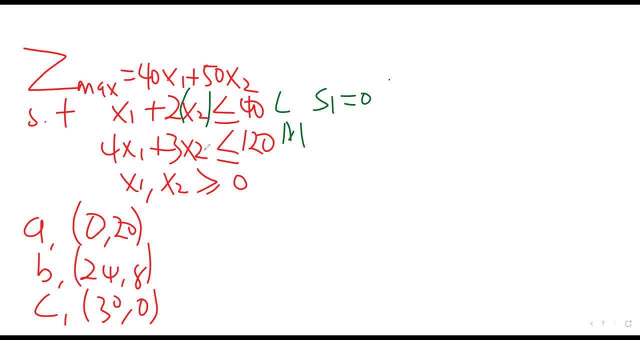 20.. Okay, When you do that 3 times 20, the slack 2, the s2 will be equal to what? Let me see whether some of you are thinking, Thinking faculty Beautiful. So you will have 60 gallons of slacks. 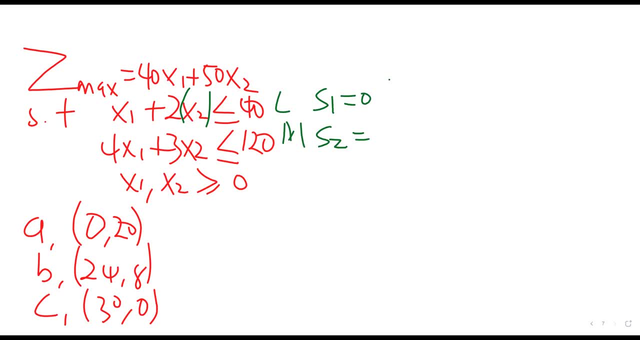 Okay, So the s2 will be 60. Because it will be 120 minus the 60. Remember, you are dropping 20 here. You are dropping 20 here, So it will be 3 times 20, which is 60.. 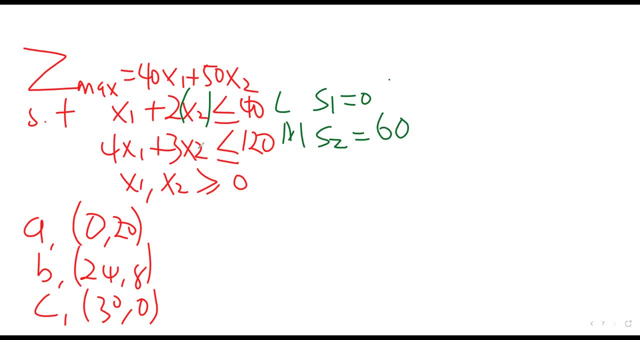 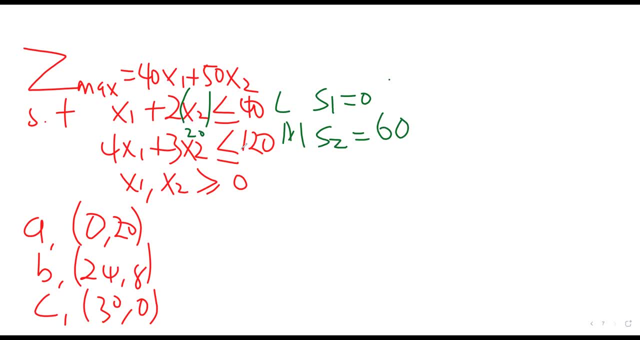 Okay, So you have the s2.. Okay, You get more 20.. However, first you need to remember that you have 60 more before you get to the 120.. So there's a slack, there's a wastage, there's an inefficiency, that on used milk, which 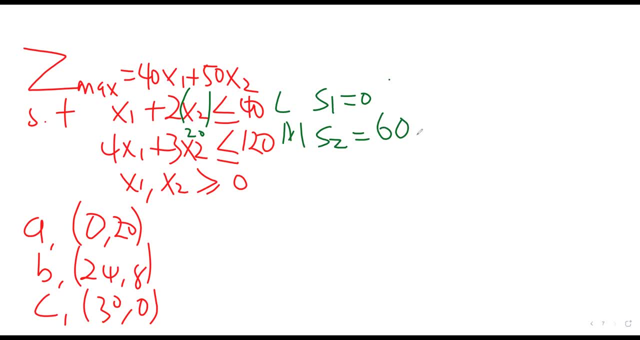 is what 60.. So for 0.1, a you have slack of zero for the s1,, 60 for the s2.. Now let's go to the coordinates of b. Okay, The coordinates of b. what is the slack s1,? what is the slack s2?? 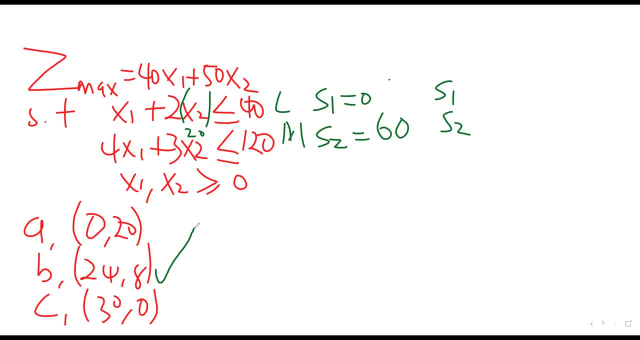 and then the coordinates of c. please, if you already raise your hand, i just want to give a max to somebody. okay, coordinates of c. what to be? the slack s1 and the slack s2, that is, if you are working along without any copycatting teofania. 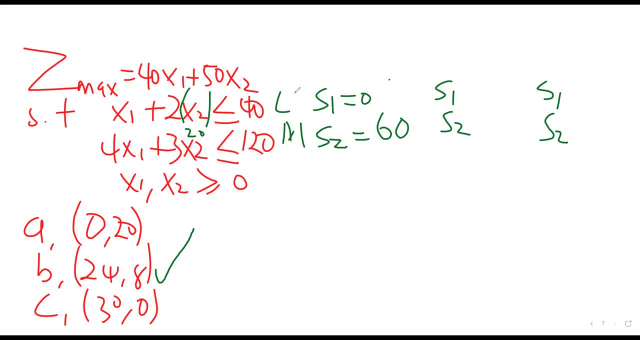 yes, so for the b labor is equal to zero, so it's equal to 40, so there is zero slack. and then milk is also equal to 120 hours, so zero slack for both labor and milk. i'm just kidding, that is correct. okay, you have zero there. excellent, very good. i've given you two marks for that. 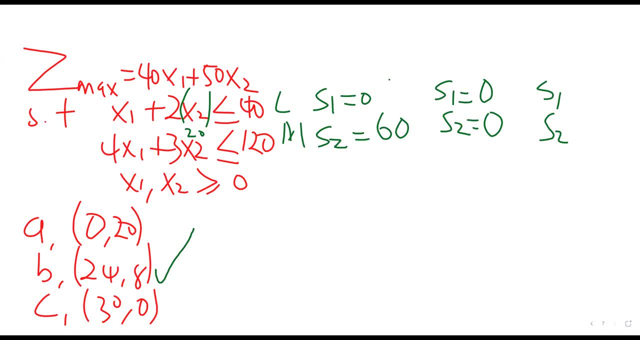 bennis would work it out for you. so take note, you have two months. let's go to another person for the coordinates of c. but the coordinates of c, let me go to Special authority job coordinates of c. yes, we have the coordinates to teachvolt, the first country. the slack will be 10. 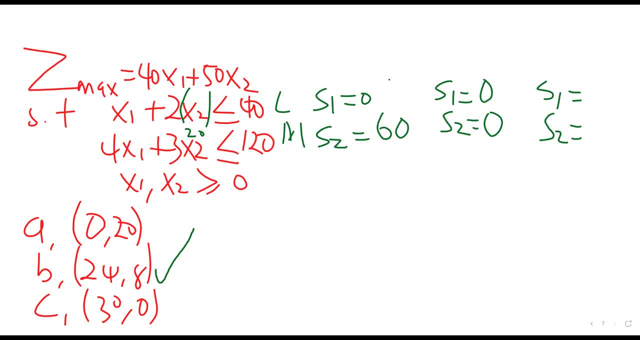 and the second one, the slack is zero. excellent, very good. that's also two months for you there. so, guys, you may be wondering, and sitting down on your chair, you have expected to sit down on your chair. what is this? what kind of hebrew? what kind of hebrew and latin are these people talking about? 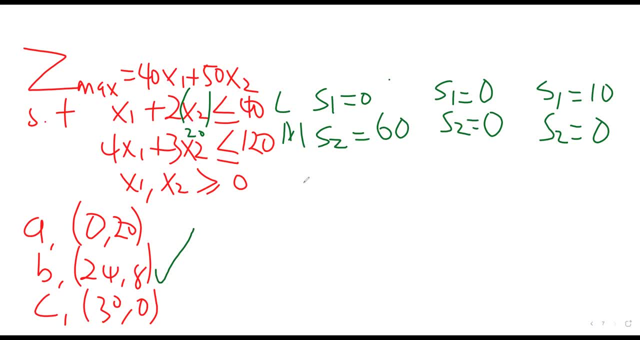 that i can't see. the whole thing sounds like hebrew to me. okay, and it is not about that. it is more about your capacity to understand what is happening. so let's go to, for example, the b. the b is simply a matter of drop. wherever you see the value of x1 and x2, drop the 24 and 8. 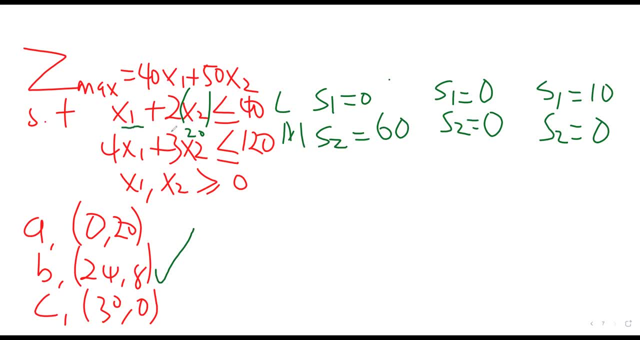 so if you put a 24 at x1 and you put the 8 at x2 in the first constraint, 24 plus 8, 8 here times 2 will be 16. so the 24 plus 16 that will be 40, and if it is 40 it means that the left hand 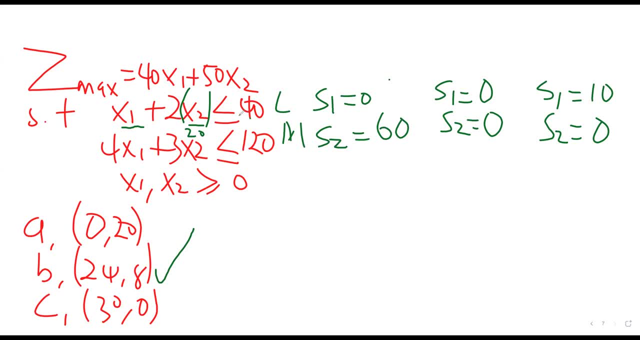 side is equal to the right hand side, of the left hand side, of the left hand side, of the right hand side. and, ladies and gentlemen, we've been saying it: when the left hand side equals the right hand side, then the slacks is what? zero, it's always like that. okay, okay, but when you do that, and then the 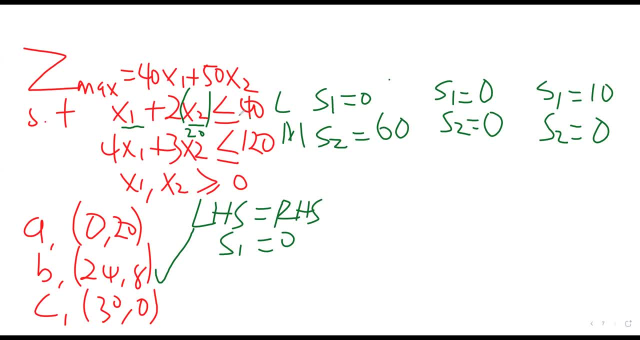 left hand side is not the same as the right hand side, then there is a slack there and you have to find the value of the slack. so, for example, if you look at c, the c values were third. okay, you have 30 and then you have zero. the 30 is for the x1. so, whatever you see x1, you put 30 there. 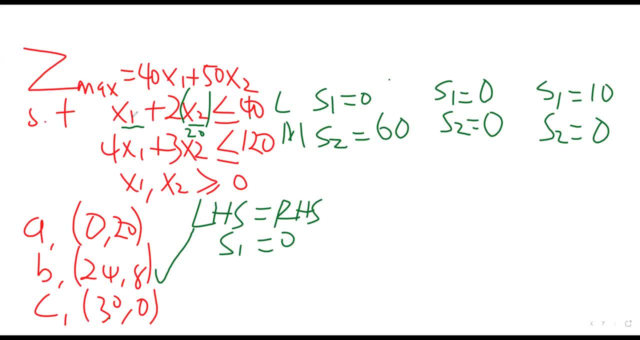 so let's go to the first constraint, the labor constraint. wherever you see x1, you put there today the x2 is zero, so you don't even look at it. so if this left one here is 30. that is not up to the 40.. 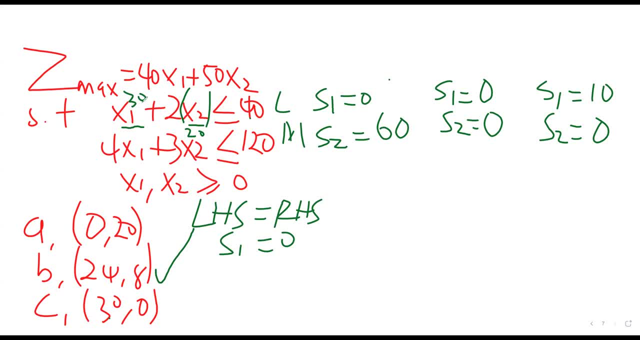 so even it's not up to the 40, there's a gap, and that gap is a slack. so there's a gap of what? 10. that is what my good friend said is 30. time. but let's go to the second constraint. okay, again, you put the 30 in the first one here. 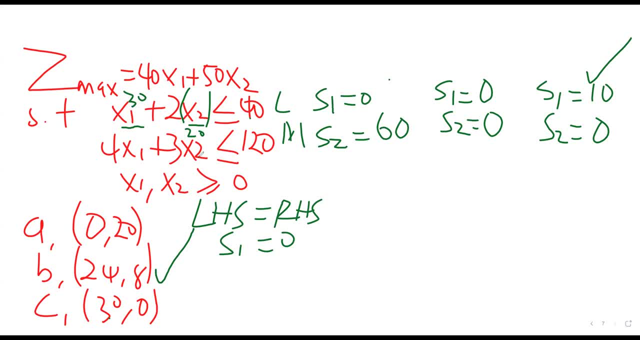 so you have four times 30.. that's why the x2 is zero. so you have four times 30, and four times 30 is what it's 120.. so you have 120 on the left hand side and you have 120 on the right hand side. so 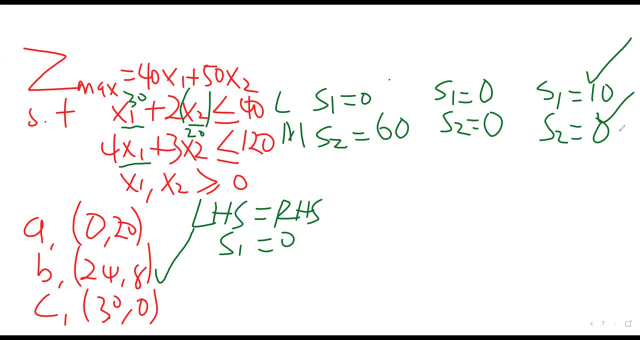 the slack will be what? the slack will be zero. that is why he said so. the point is that you should be able to connect the left hand side with the right hand side and the right hand side with the right hand side, calculate slacks at all the vertices, at all the corner points, at all the coordinated points. 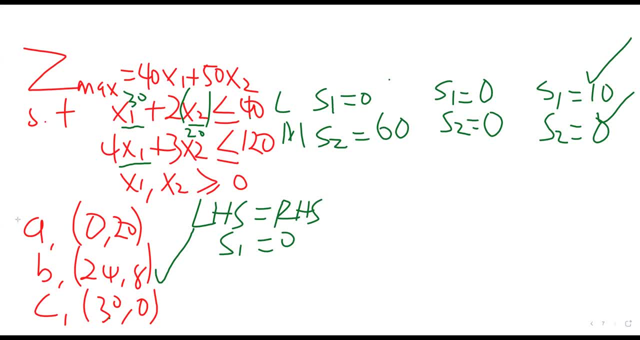 you should be able to identify the slack. so anytime you get a slack, calculate them. calculate the slacks at the corner. but there's something interesting in our work we've done today. watch it. you will notice that the one that gave us the coordinate, the b point, that gave us 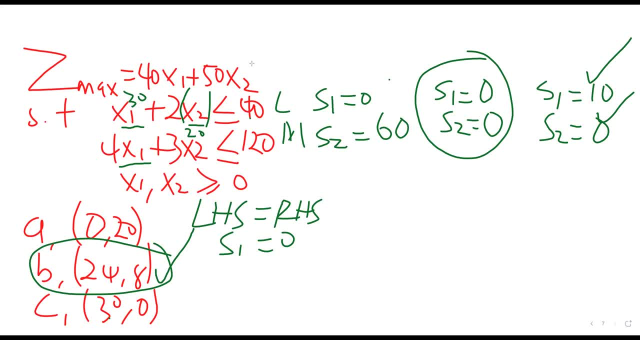 the highest profit. it also gave us zero slacks. what does that mean? what it means is that if the company should produce at a point b, they are going to be efficient. they are going to be efficient in that production. there's not going to be any wastages, there's not going to be any unused resource. all the 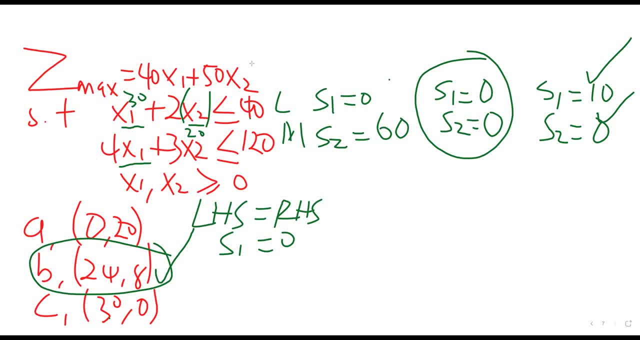 resources are going to be fully utilized, and that is pure efficiency. and so that is why it makes sense for you to advise management to produce at the point of what b, because that point and point will give them the best, best solution without even incurring any slack. 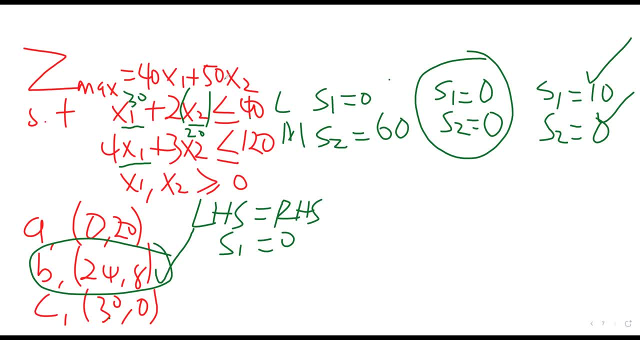 Now that is not to say that it's always going to be, that you know, anytime you produce at the optimal, you will not incur some slacks. Please note: sometimes you'll be producing at the optimal and still incurring some slacks. 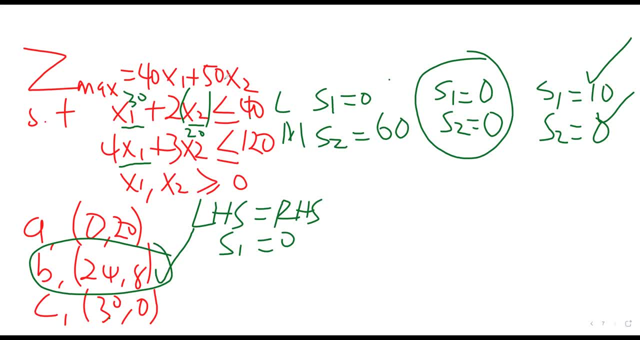 But of course, you would want a situation that will give you the best, highest output. So when you're learning this, you don't just learn and say I'm lost, Because when you say I'm lost, it means that you are in a jungle. 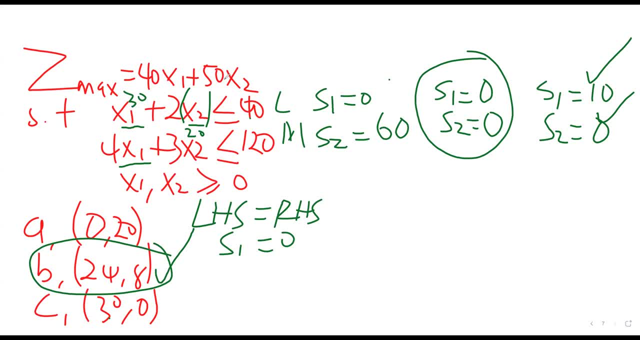 But you say: I do not understand this very aspect of why this and this is happening That way. you have a prior knowledge to contain. See, knowledge begets knowledge, Knowledge commands knowledge. So there are some questions a person will ask me, and I know that that person cannot. 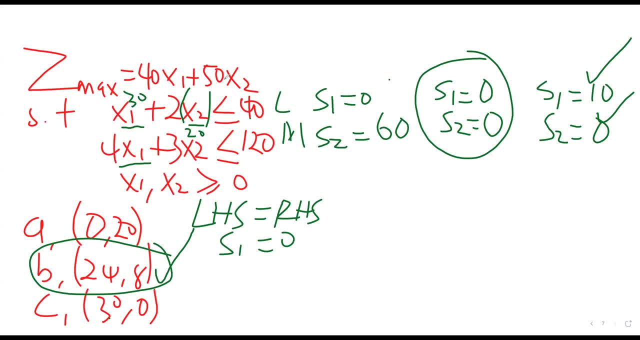 stand here now. The person can't stand here now. Why? Because a person needs to go and learn the very, very basics to be able to ask that very question. All right, So we have been able to do this standard form and all of that. 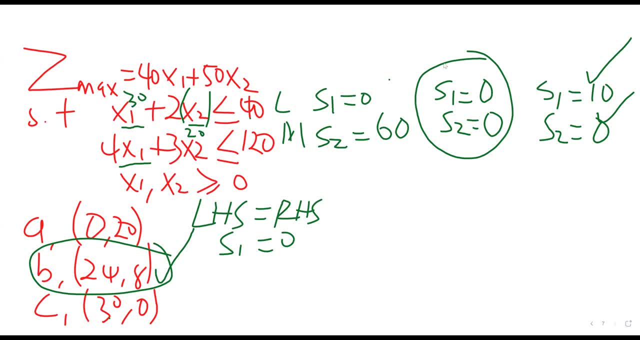 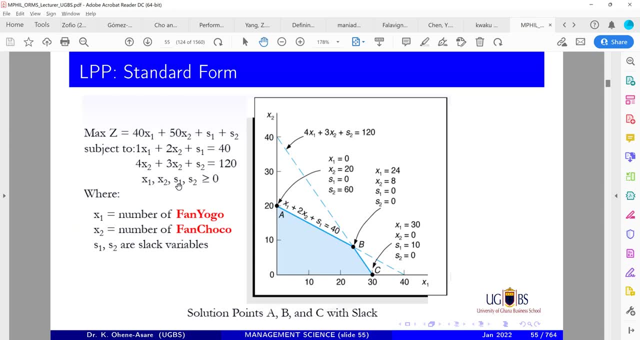 Now let me show you something. I'm now showing you something in your slide. Just look at the slide. So in your slide you will see that I've done the conversion of all the fun you go, And at each point you will see the slacks. 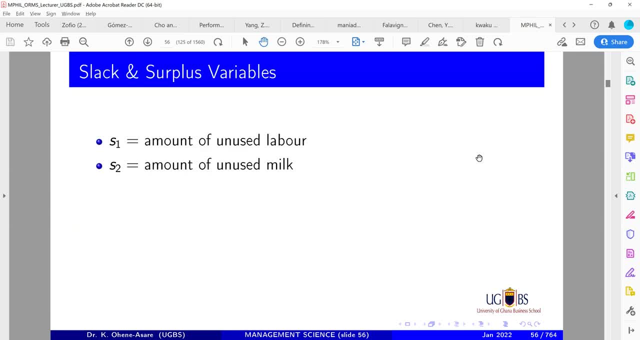 There You will know whether the slacks are what it tastes or the slacks are not what it tastes. Now let me ask you a question. Let me see who can give me the answer to this. Who can tell me the values of the slacks at the origin? 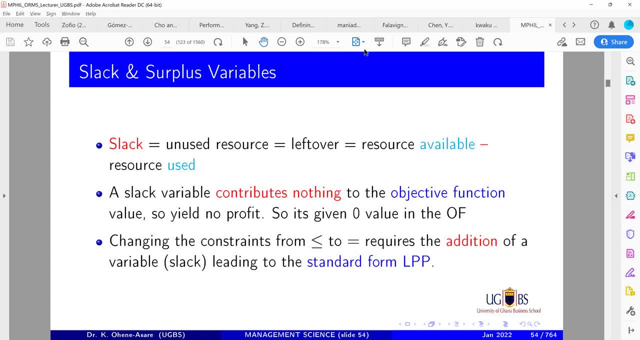 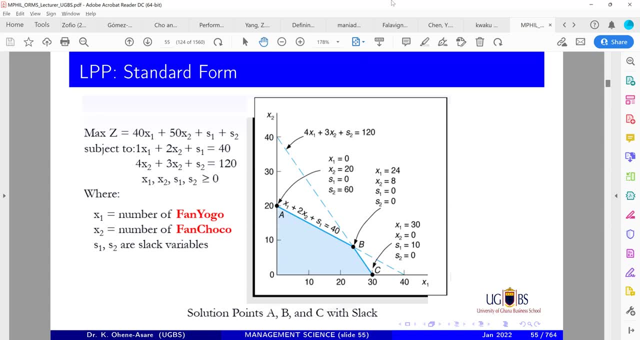 Okay, What do you think will be the value of the slacks at the origin? Look at the picture there. At the origin, what will be the value of the slacks? Who can raise their hand and tell me If you can tell me that? 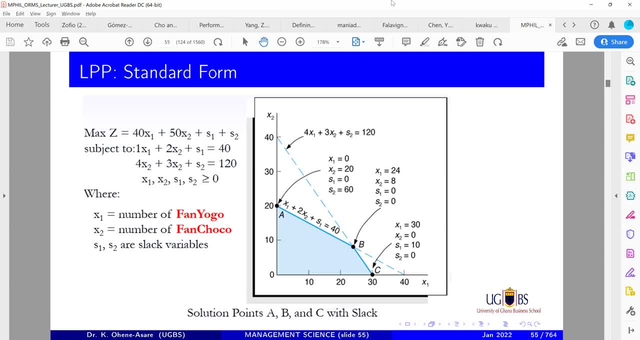 It means you are fully Fully with me. What is the value of the slacks at their origin, Vincent Jason? Yes, sir, At the origin, S1 will be 40 and S2 will be 120.. Excellent, Why. 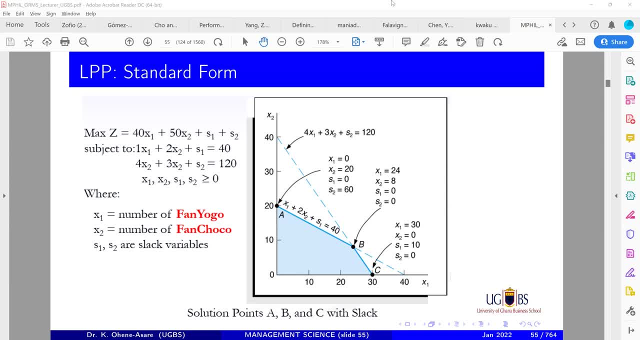 Why did you give the answer? That's because at the origin, we are not producing any fun you go or fun you go, So there will be maximum wastage. I like that. I like that word you used: There will be maximum wastage. 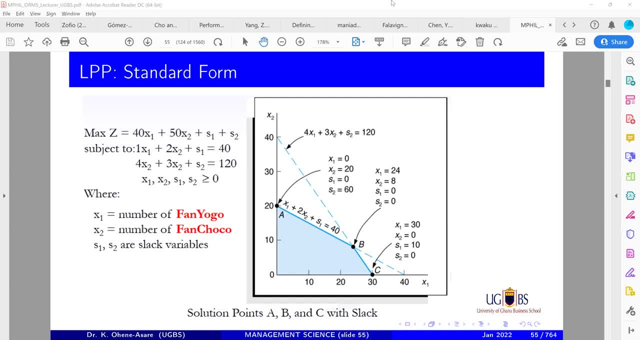 So what it means is that you have not used any of the resources. So the unused resources are what is there. But that's very good, I'm giving you two months for that. That is an intelligent answer. So at the origin you have not used the resources anyway. 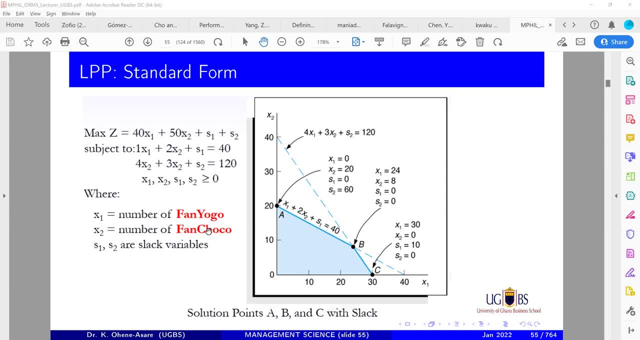 So all the resources are unused. So if all the resources are unused, then the maximum number of resources will be the available resources. James, is your hand up? Yes, Do you have a question on that? Do you have a question related to that? 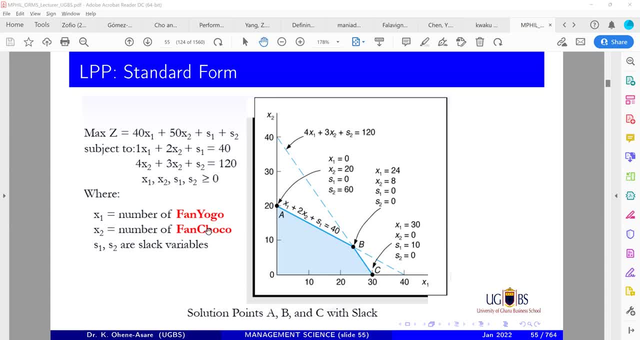 So that is it At the origin. I don't have to give the answer, No problem. So you lower your hand once the answer is given, Because you can't give a double answer to an already given answer. I know you want mine. 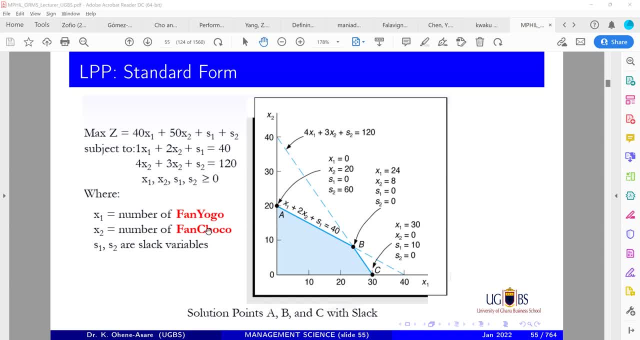 That is life, All right. So that's You see, your ability to understand these things is very good. Now let me ask you something. As you look on the stage, As you look on the, I want you to educate me on something you know very, very tiny here. 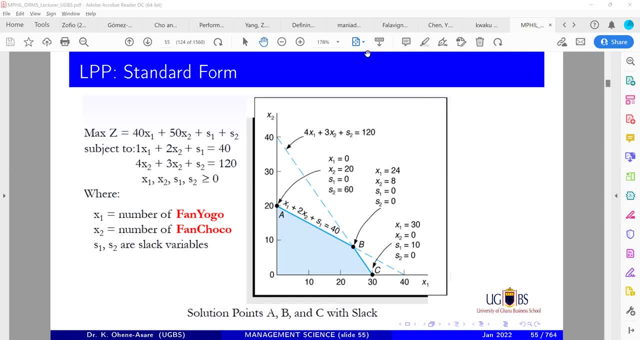 Now, if you look at, If you look at the formulation very carefully, If you look at the formulation very carefully, You will notice something related to the production capacity. If I ask you just on the screen, Let me just move to another formulator. 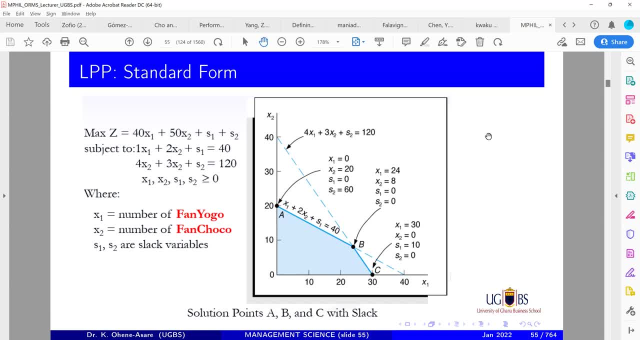 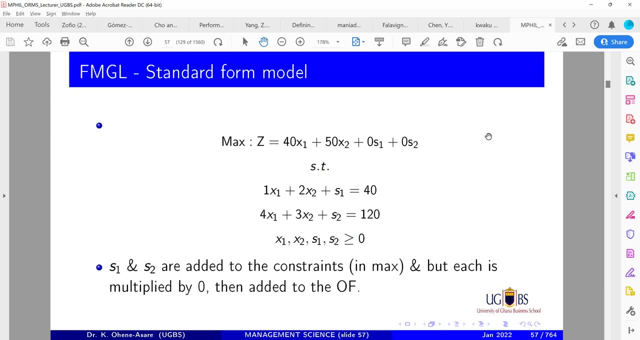 I just want to go to another formulator, anchor, to ask you- So this is for the slide Now when you look on the screen- If I were to ask you without finding the answers, okay, And I ask you that, what is the total number of gallons of milk that was used by this company? 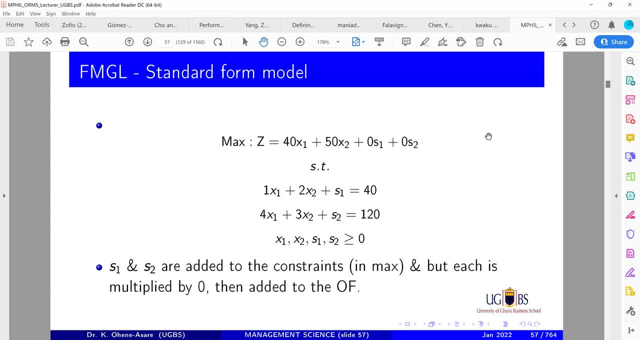 Which mathematics will reference that? What is the total gallons of milk that was used by this company? Who can tell me that? What is the total gallons of milk that was used by this company? If you look at it, Used, used, used by this company. 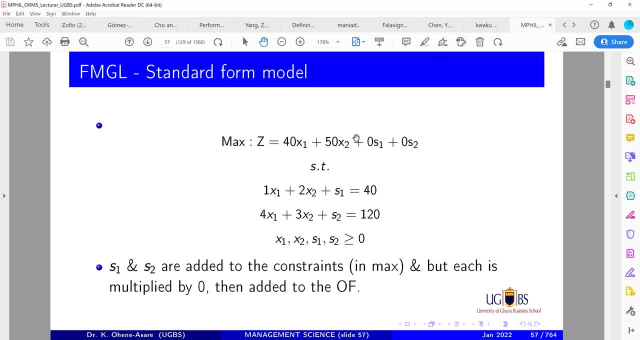 What is the total gallons of milk that was used By this company? by this company, remember, the usage is the left-hand side of the equation, the available is a right-hand side of the equation. so if i'm asking you that, gallons of milk, how many? 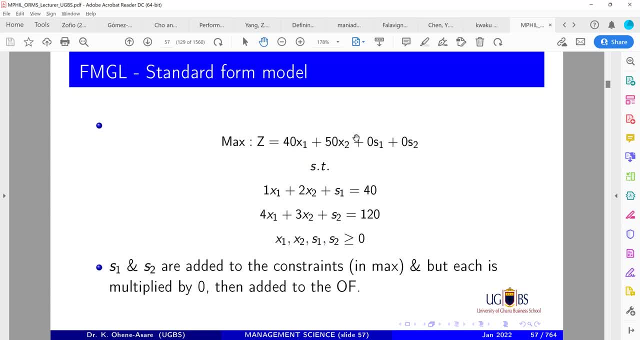 gallons of milk was used by this company. what would you say? let me go to irama, irama. what answer do you have for the gallons of milk that was used by? okay, could it be um less than or equal to 120? yes, but on the screen, just tell me what it will be. that's what i want. 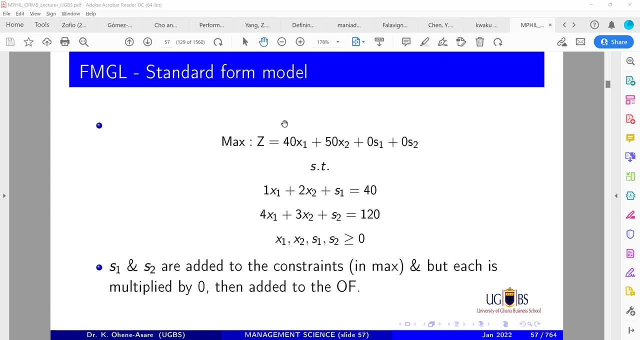 i want you to tell me, because you don't know the value yet. you don't know the value yet. but if i were to ask you, okay, you, you don't know the value. so what do you see in the, in the story, that would tell you the value, james? 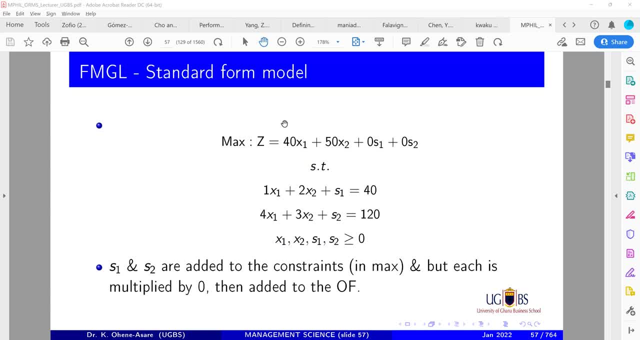 you have something to give to us. what would that be? um, i have. um, i'm a little bit confused. yeah, from the onset you were solving, you were subtracting that slacks from the left side of the equation. but here lies the slice: is having, um, you are adding the slacks to the left side. 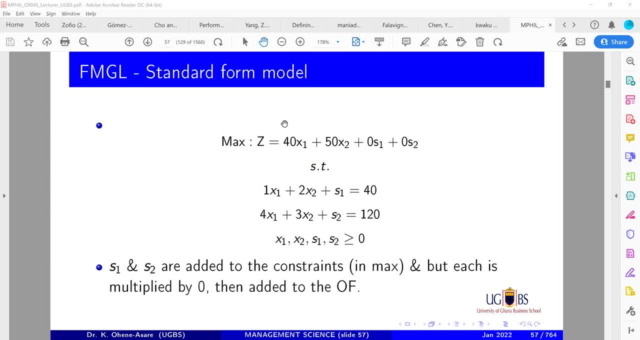 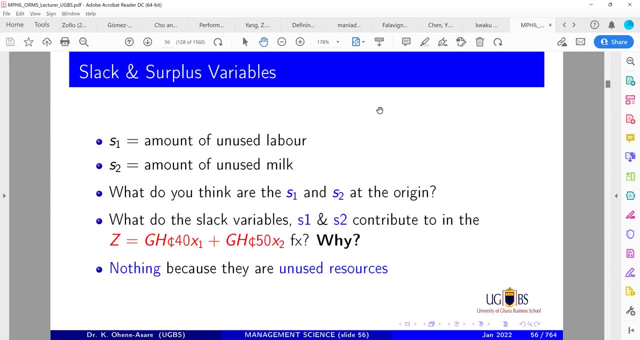 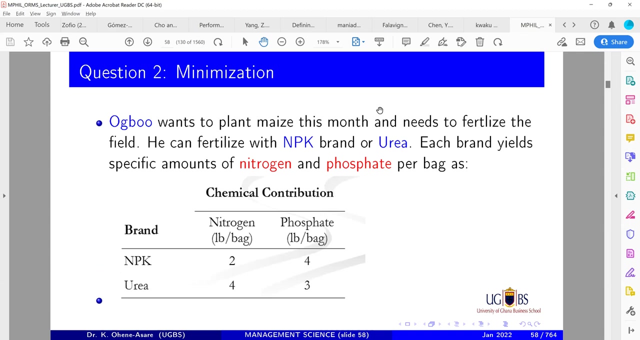 of the equation. was i subtracting? yes, please, okay, okay, then that's fine. it rectifies okay. yes, thank you, okay. yeah, that's a good point of notice. yeah, supposed to be subtracting. let me go to the original so that you all see the original equation. 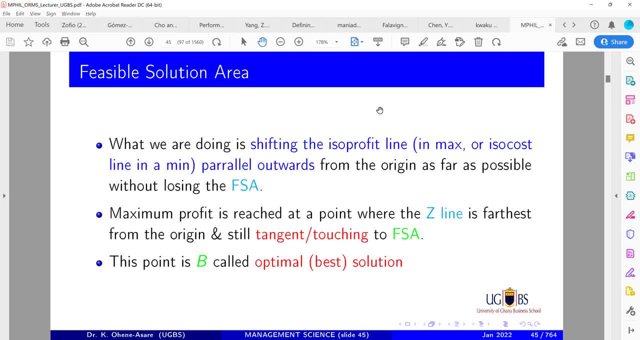 oh, so you were just saying that you didn't. you aren't going to answer my question. okay, so let's go to kelvin to see whether kevin will be able to answer that question. kelvin, yes, yes, sir. so if we want to know the number of gallons that were used, it's 4x1 plus. 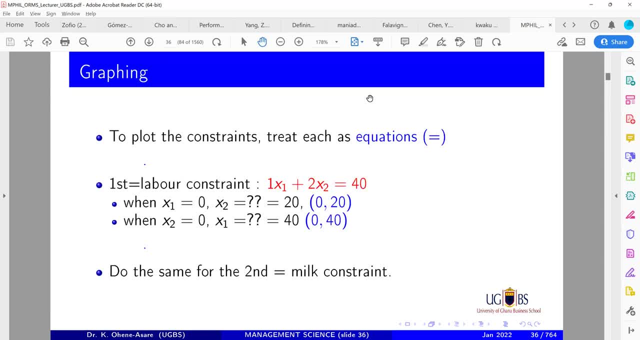 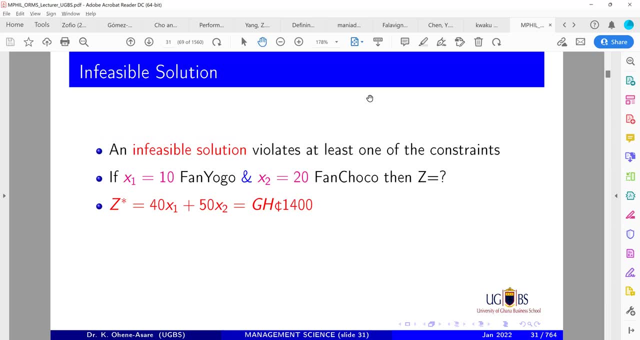 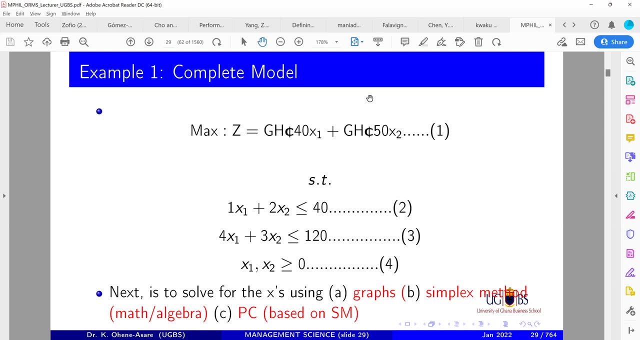 3x2, exactly, exactly, assuming we don't know the value of the slacks. i just want to see if i can show you the entire question. okay, so this is the entire question. yes, okay, so what if i ask you how many hours of labor was used to produce fan choco? 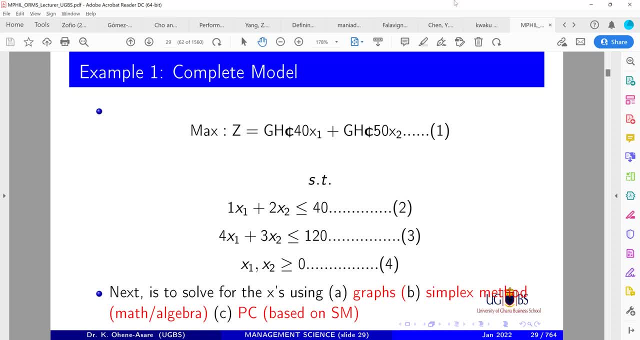 what to represent that. how many hours of labor was used, just as you're looking at it on the screen? hours of labor was used to produce fine chocolate. Victoria, I like your answer 2x2.. Very good. How many gallons of milk was used to produce fine yogurt? How many gallons of milk was used? 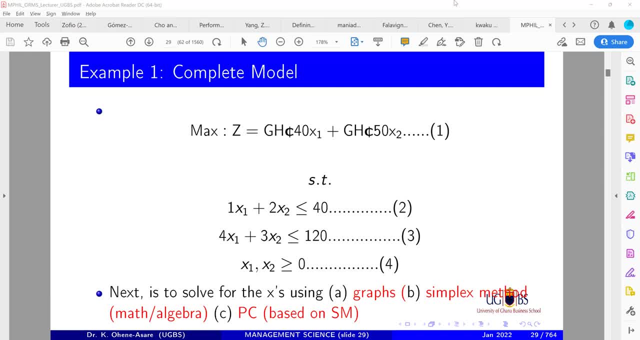 to produce fine yogurt? You can type me an answer there. How many gallons of milk was used to produce fine yogurt? Excellent, That is 4x1.. Okay, Now listen. What was the total profit of farmer gunner limited? What was the total profit of farmer gunner limited? So this is: 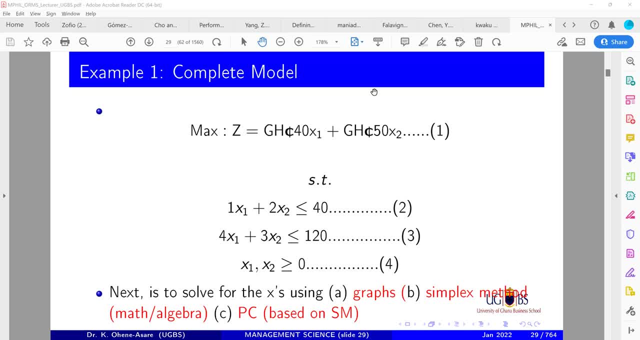 before you even solved it. What was the total profit of farmer gunner limited? What was the total profit, Total profit, Total profit of farmer gunner limited. All the answers I'm getting are wrong. I don't need a numerical answer. The right answer is from Linda in. 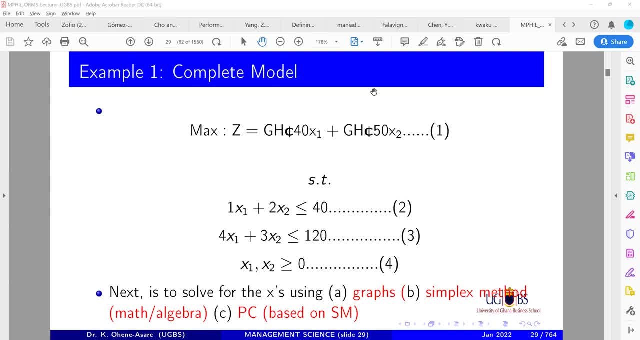 Victoria: 40x1 plus 50x2.. That's the right answer. 40x1 plus, That's the total profit. Now, when you now know the values of the x1, you can substitute it, But now, as it is on. 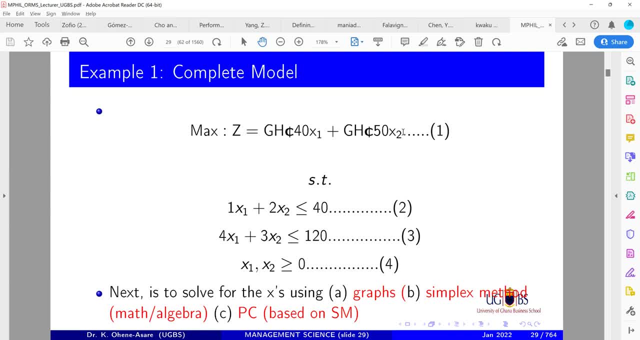 the screen. that is the total. So how much profit was made in the production of choco? How much profit was made in the production of choco in this time? Sorry, How much profit was made in the production of choco? It's 50x2.. It's 50x2.. It's 50x2.. 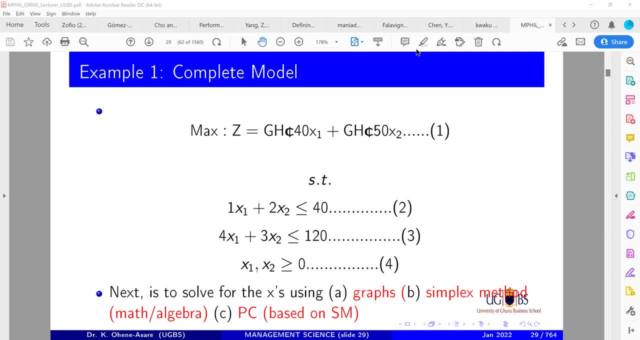 Your colleagues are doing it and you are not doing it. It means that you need to sit down and drink water and absorb the information at your own relaxed time, All right. So, ladies and gentlemen, your ability and your capacity to be able to decode these calculations is 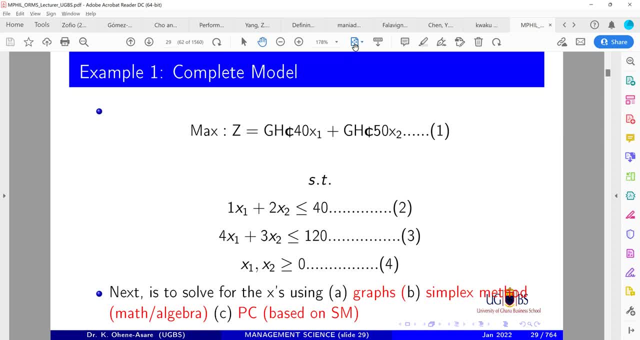 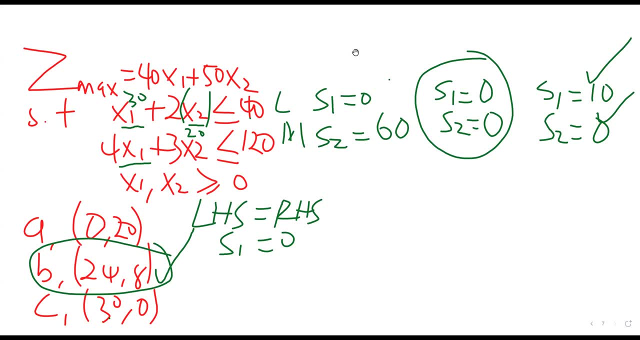 the first step, Okay, In learning this, Now, this linear programming that we have done today. they are normal, They are regular, They are very regular. When I say they are very regular, somebody might not understand. But what do I mean by regular? Okay, Now, what it means is that you found: 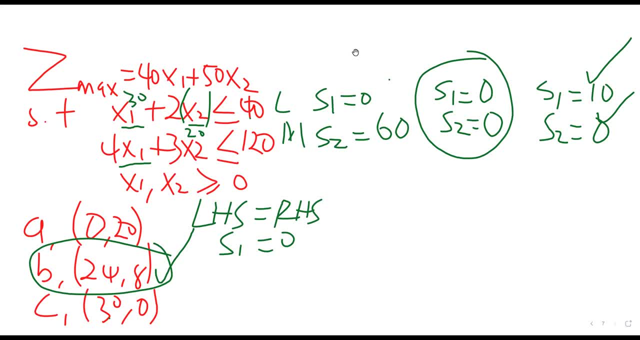 one solution. You got the solution first of all And there was only one solution. If you can remember one solution point we had Because the point B, Producing 24 units of fine yogurt and 8 units of fine choco. So 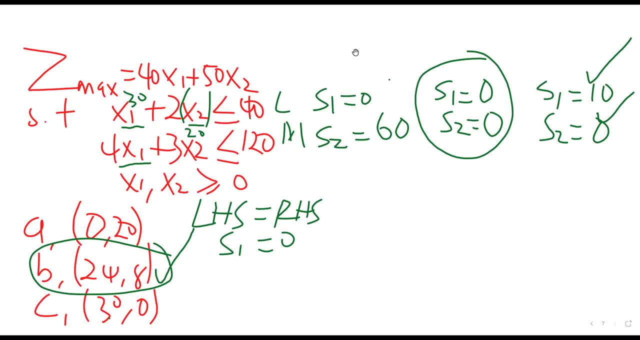 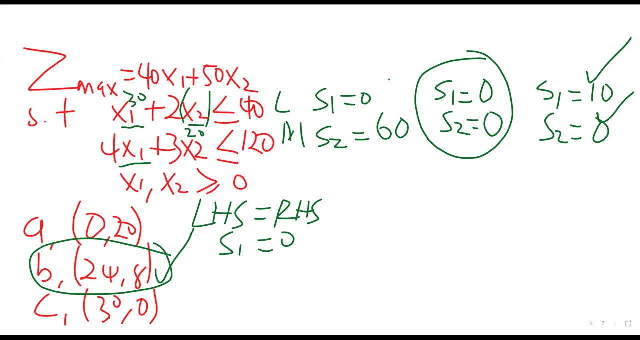 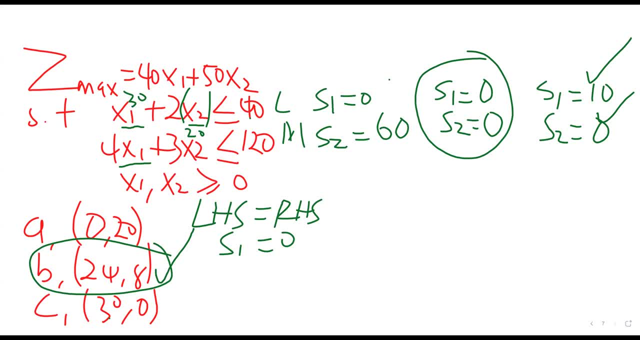 Try their science to come up with multiple solutions. How can you- you know, can make many calculations- Find multiple solution? right, Can you make multiple? And so I'm going to show you something we are going to do next- Okay, Next time- what we're going to be doing. 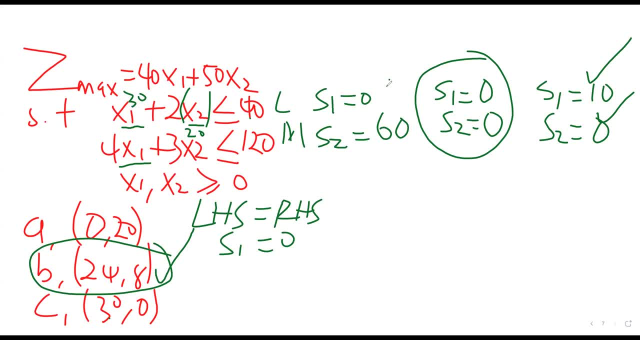 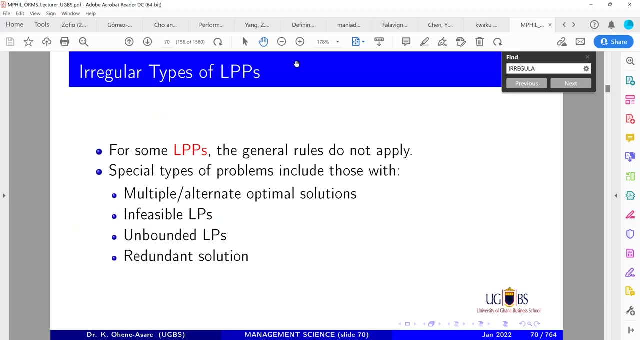 We're going to be learning, Before I go, something known as the irregular types of linear programming model. okay, okay, and we are going to do that next time. irregular types of linear programming model. the first one will be the multiple: optimal solution, infeasible solution, unbounded, and then redundancy. okay, the multiple. 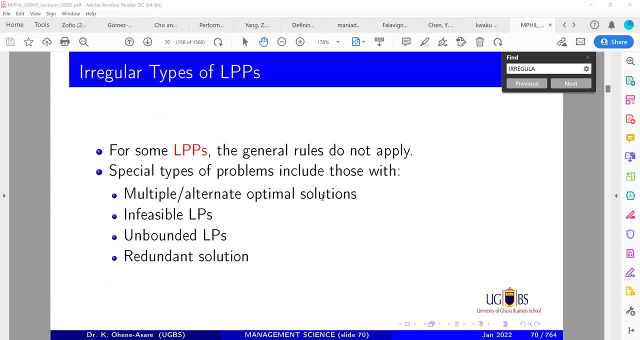 optimal linear programming, infeasibility, unboundedness and redundancy. now, they are not regular, they are kind of abnormal kind of, and so we are going to study them and know how you can identify them and why they happen. and why they happen. ladies and gentlemen, that brings us to the end of the entire caboodle.